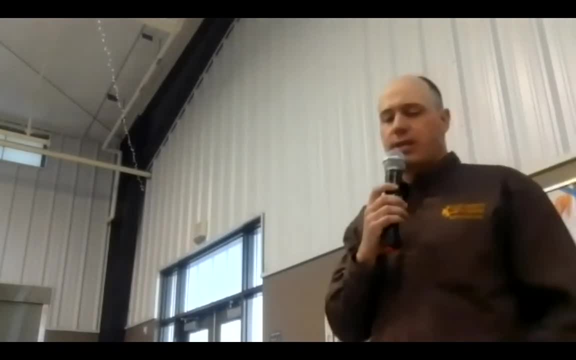 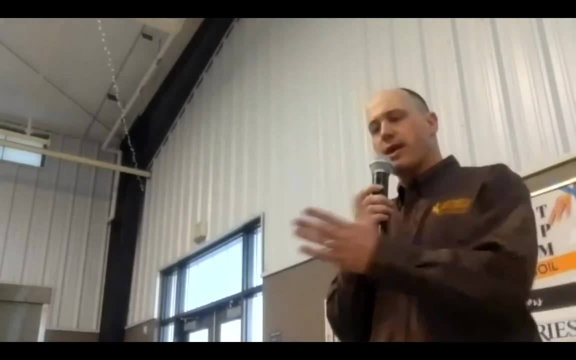 or ion battle, And then we'll go into a little bit on precision fertility. So we're going to get started first and talk about the ion battles, We're going to take a short break and then we'll roll into that second presentation on precision fertility management. So without further ado, 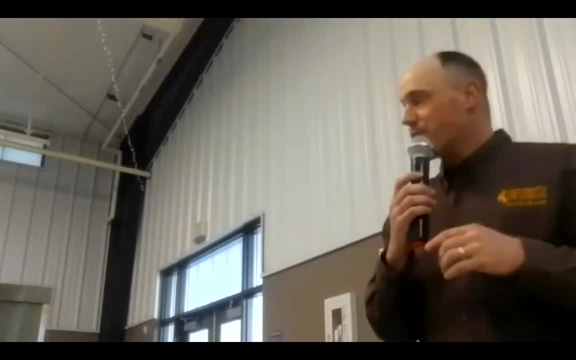 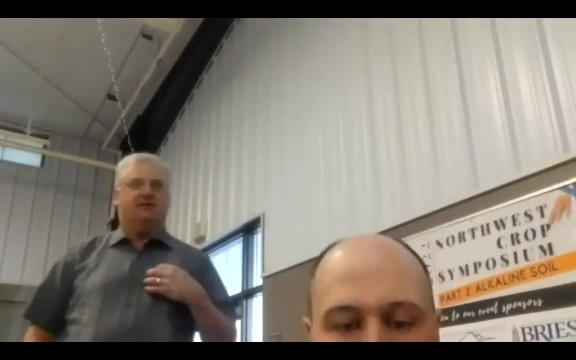 I'm going to turn it over to Dr Stevens. Dr Stevens, you should be live, I think, on your mic, but we'll just do a check before we get rolling and I'll share you All. right Sound check. Can you hear me online, Okay? 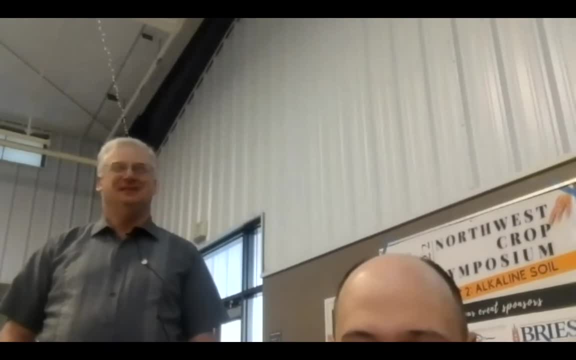 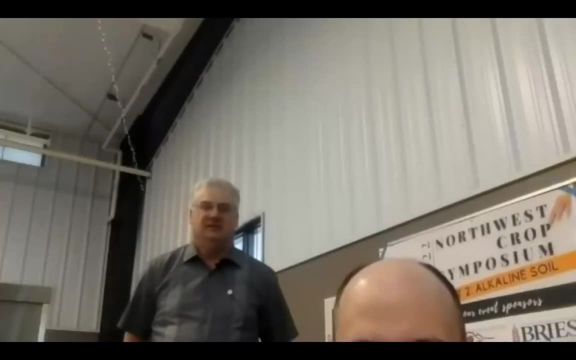 Testing, Testing. Okay, You can see you guys. Sounds like we're good, All right. Well, while Jeremiah's getting things going here, let me just tell you how glad I am to be here, to be able to talk to you a little bit today. 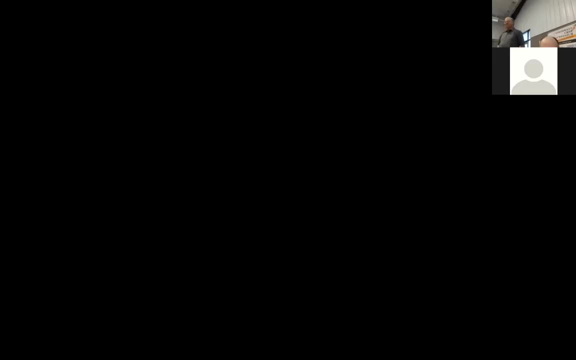 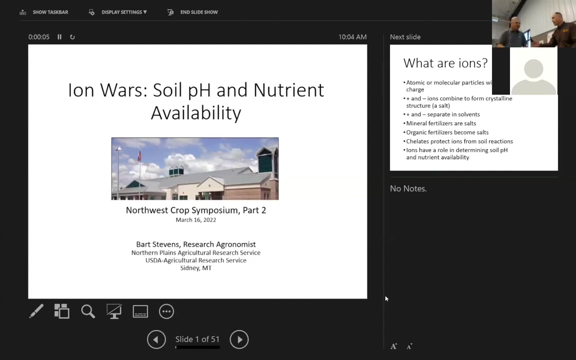 It's always good to come to Wyoming, Wyoming's home, and I'm glad to have an excuse to come back home. So all right, Thank you. I did try to get a little bit creative with the titles of my presentations. I'm a little hesitant to do that nowadays, to try and be creative or funny, because my wife tells me 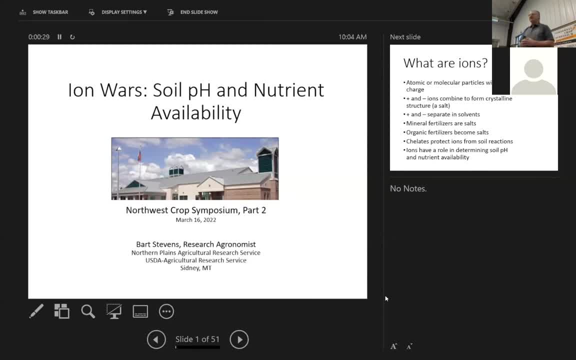 when I try to be funny, I'm just annoying. So I hope that's not the case here today, And I'm also glad to kind of be able to talk a little bit about research, Something that I don't do as much as I used to. I've taken on a little bit more of an 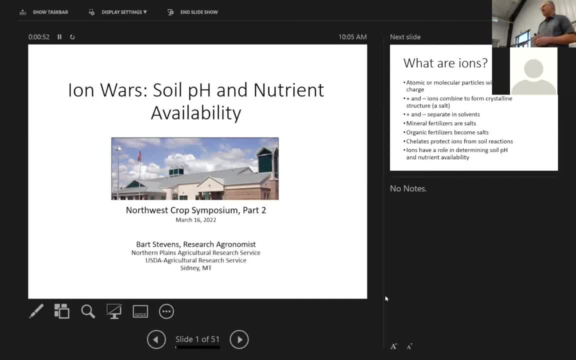 administrative role at our lab in Sydney And that takes time away from what I really love to do a little bit. But glad to have this chance to share some of my thoughts with you. A little bit of a disclaimer, I guess, as we get started here. 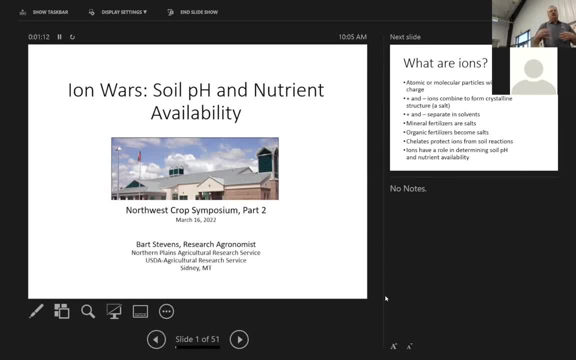 I want to talk a little bit about some of the processes that are involved in in how nutrients react in the soil and make some practical applications to that, the best I can and same with the variable rate technology stuff that I'm going to talk about not going to get too sciencey. 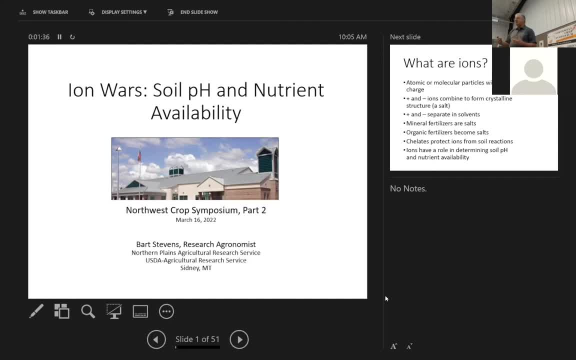 but I'm also not going to go through a list of products that are available and say this is what you should use and this is what you shouldn't. first of all, there are too many and they all have a little different, different properties. but also that's. that's really not what my role is. 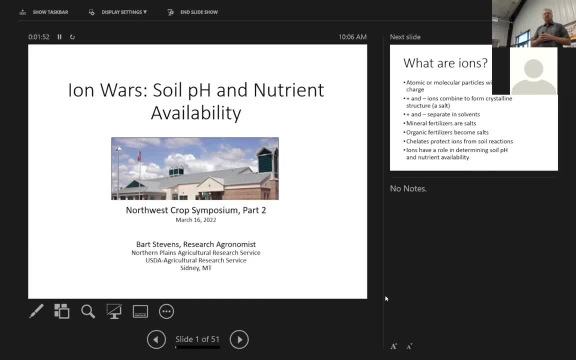 at USDA, at our research lab, we're looking at things a little broader sense in our research, but I'm going to try to draw on some some research that I've conducted over the years and and some of my colleagues and friends, and hopefully share some information with you. 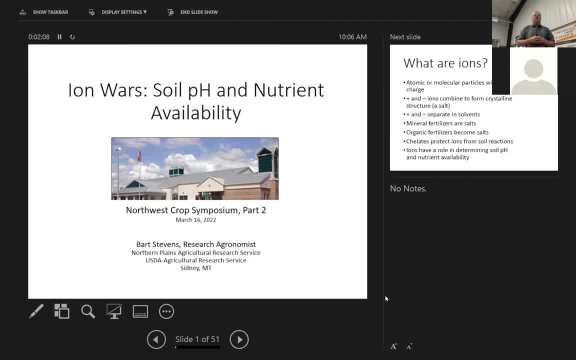 it'll be helpful. so glad you're here and I want this to be, you know, informal. please speak up if you have comments, questions, and I expect I'll probably learn as much more from you. but before the day's over the media for me, I hope you learned something from me. all right, so let's get started here. 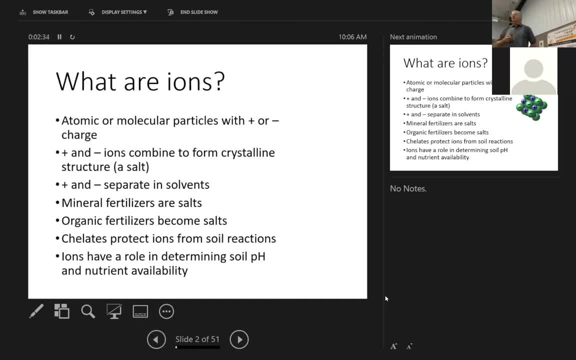 I'm focusing on ions, because our fertilizer nutrients are ions when we put them into the soil. so what are they? they're charged particles. what minus goes back to high school chemistry, for we all remember that with fondness. I'm sure they can, you know, be in solution. 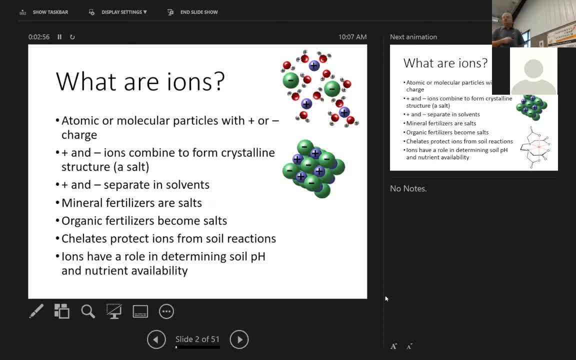 individually, or they can form structures and crystals when when they're in the dry form. and the fact that they have these charges on them is what's important to our discussion today, and that's why I'm going to start off with some of the new research that I've done. 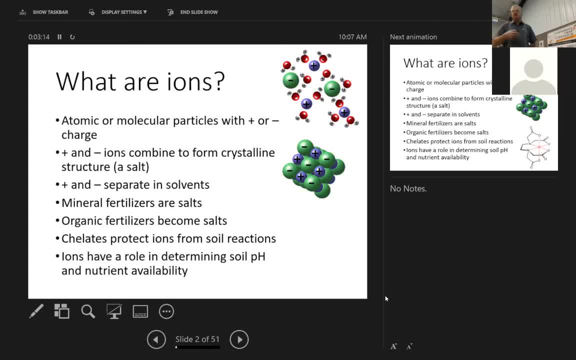 to see if any of this has come up as a good question is, in particular, what did you learn from what you know? in our field, there are different features to a lot of the different varieties of a soil. there are different baskings in the soil. some of them are run off the soil. 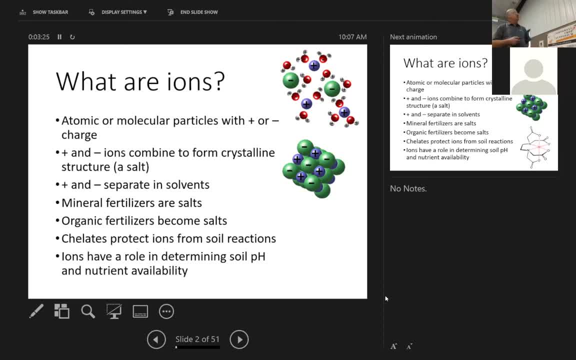 some of them are positive. some of them are positive and, as you're probably aware, even our soil particles have a charge as well. they're primarily a negative charge, but there are some some positive. wouldn't happen if we didn't have water as a solvent, So water is a critical part of this equation as well. 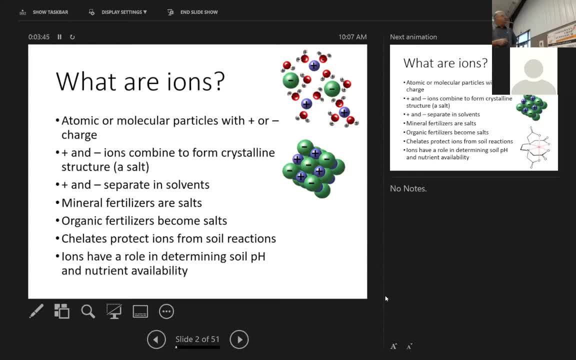 Our mineral fertilizers are salts for the most part. Organic fertilizers may not be to start with, but they become salts. That's how the plants absorb them in the ion form. Now let's talk a little bit. we're just briefly about chelated fertilizers as well. 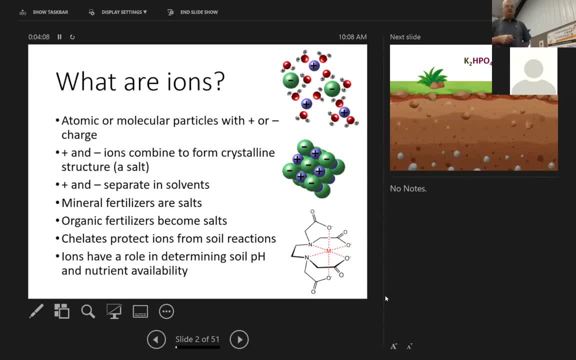 A chelate is kind of a complex molecule that I'm showing on the bottom right of the screen here. that kind of wraps around that salt or that fertilizer ion which is represented by the red M in the middle, And it kind of forms a little bit of a loose bond. 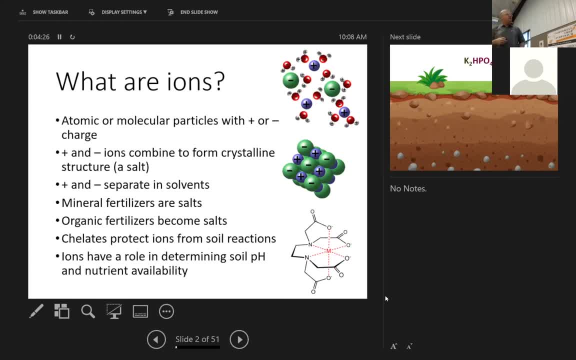 so that it can be released fairly readily. but it protects- protects it from some of the other reactions in the soil that we'll talk about in a few minutes. So pH is kind of what we're going to focus on here, And that is definitely an important factor in all of this. 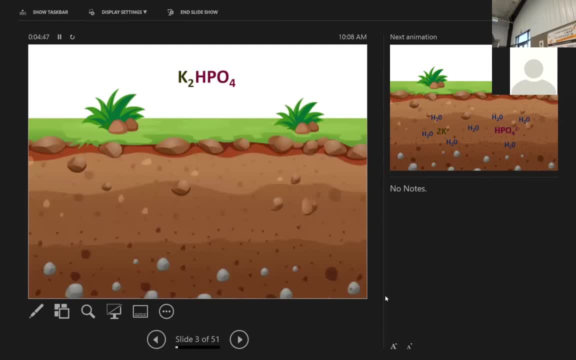 All right. So a little bit of a conceptual thing here. I've got on this slide chemical formula for a potential fertilizer. Now this is not one that we really apply Normally. this is not one you can probably buy down at the co-op. 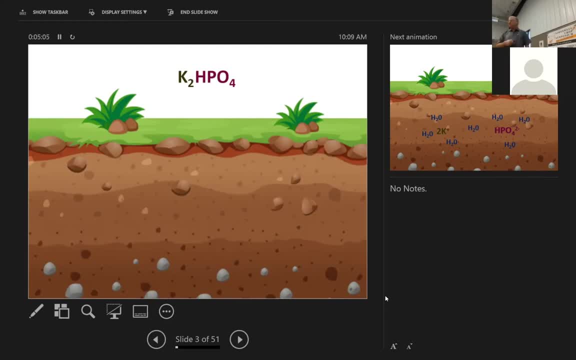 but it represents two nutrients that we're interested in: Potassium on one side and the phosphate on the other. All right, And we've got our soil here with plants going on it, So ideally it'd be nice if we just put that fertilizer. 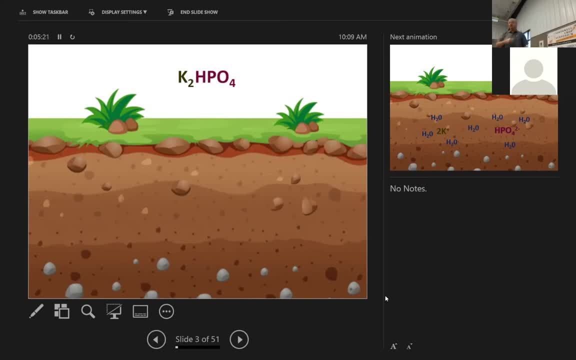 on the soil. it would just. right now it's in the form that the plant can use it- Put it on the soil. It's going to just go there and sit And wait until the plant needs it. And when the plant needs it, 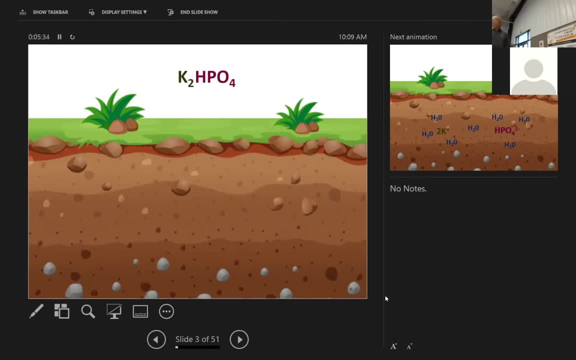 it's just going to take it out, Not that simple, though. We do have soil assistant hydroponics where it does work that way, but the soil is a much more complex environment when we add this fertilizer, So we're going to put that on that soil. 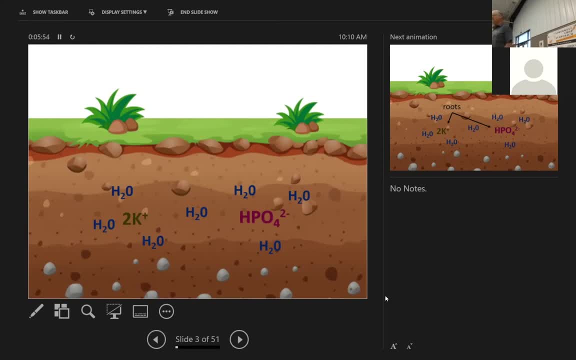 Okay, Like I mentioned before, the first thing that needs to happen is it needs to interact with water. Can't have any benefit from that fertilizer without the water. Okay, So far, so good. It's available, The plant can take it out. 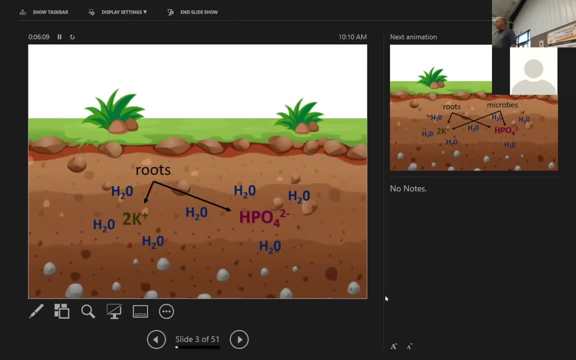 And so roots are definitely a part of this equation. They have an impact on these ions, They attract the ions to them, They flow, they attract the water, which brings the nutrients to them. Okay, So far, so good. Well, now a little bit of competition. 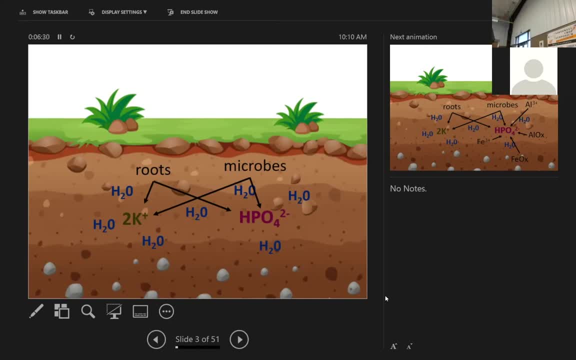 We do have those microorganisms that are in there as well. You know billions per teaspoon in some soils. They need those nutrients too. So we've got a competition And that's not necessarily all bad. We get some temporary immobilization from the macros. 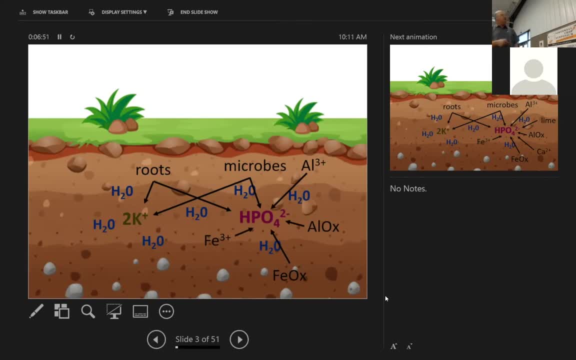 but they will eventually release that back to the soil where the plants can get it All right. Now we're getting a little more complex, So we've got things like aluminum And iron in the soil And they can tie these nutrients up. 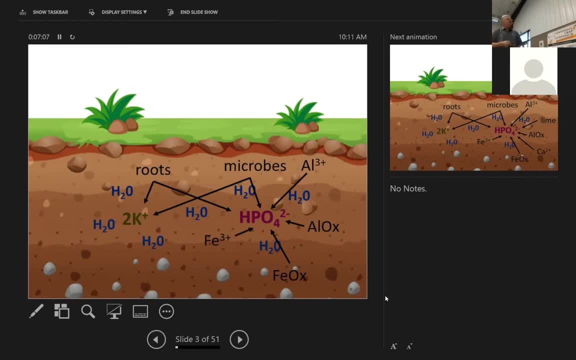 especially phosphorus and some of the micronutrients in forms that are hard for the plants to get. Okay, We don't have a ton of aluminum and iron in our high pH soils. Much more of a problem in acidic soils, but still can be a little bit of a factor for us. 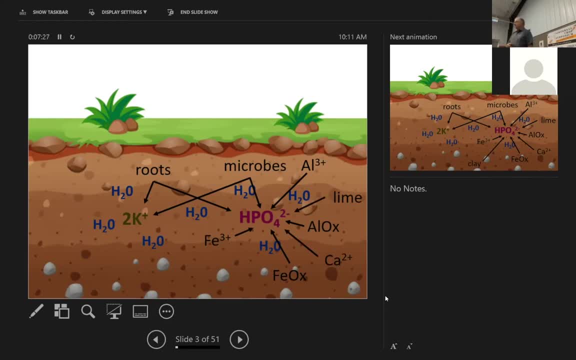 All right, Now we're getting more relevant to our soils. Our lime, which is calcium carbonate, and calcium in the soil can interact with phosphorus in particular. So far, potassium is looking pretty good. You know, most of this is kind of focused on the phosphate. 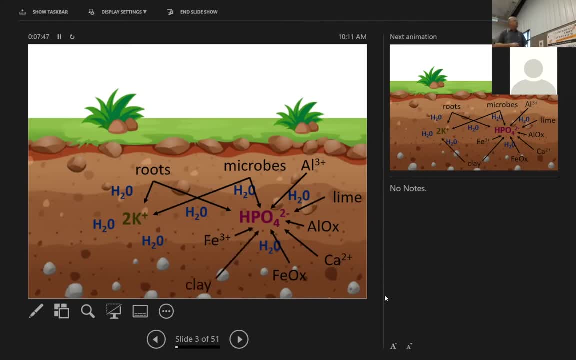 but these are the things that we're concerned about Now. is there anything else? Well, yeah, we've got clay. Anybody got clay in their soil? Well, we're in Wyoming, so you know we got clay. 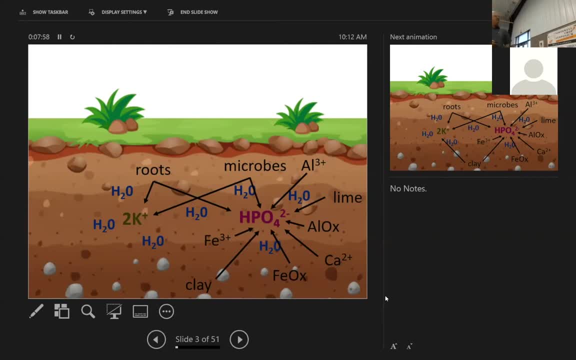 That's a good question. We've got more than half of that clay in the soil, And so that can have both a positive and a negative effect on our nutrients. Now, if we're talking about potassium, then the clay can hold that potassium. 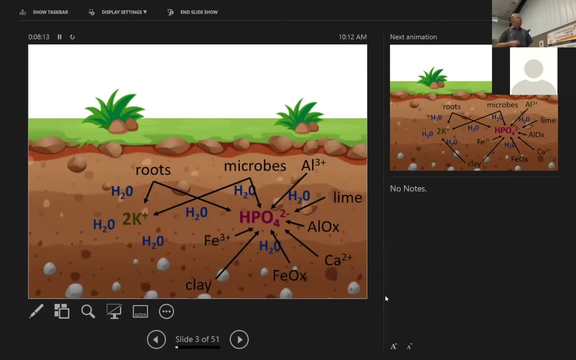 in a form that's pretty readily available to plants. It's exchangeable potassium, what we call it. It can also fix a little bit of potassium. Some soils are particularly bad at this, depending on the type of clay that we have as far as a potassium fixation, But it can also bind some of our phosphorus. 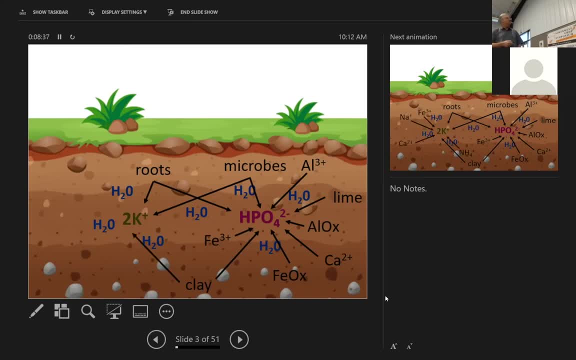 attract it to the surface of the clay and bind it there. I already mentioned the impact on potassium. Now the other factor. you know, iron sodium, calcium, ammonium do have a little bit of an impact on potassium because they're all positively charged So they're all kind of competing with. 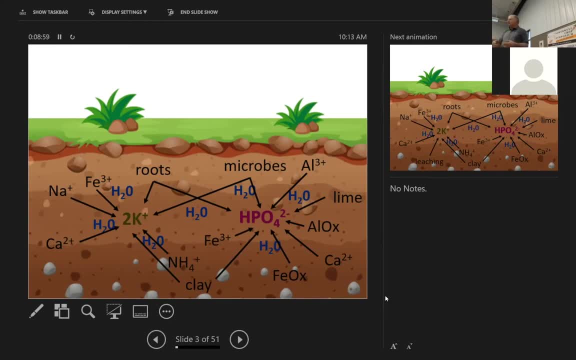 potassium competing for sites on the clay mineral and also competing for uptake in the plant. So if we have a huge excess of some of these, then sometimes that can induce potassium deficiency because potassium just can't get in. Okay, usually not a problem, but can be All right. 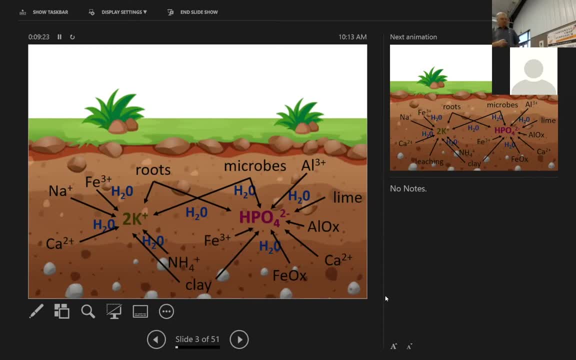 Let's see if I got anything else on there. Oops, Oh leaching. We can have a little bit of leaching. Neither of these are particularly mobile in the soil. especially phosphate, It moves just fractions of an inch from where you put it. Potassium moves a little bit better, especially in sandy soils. that don't. 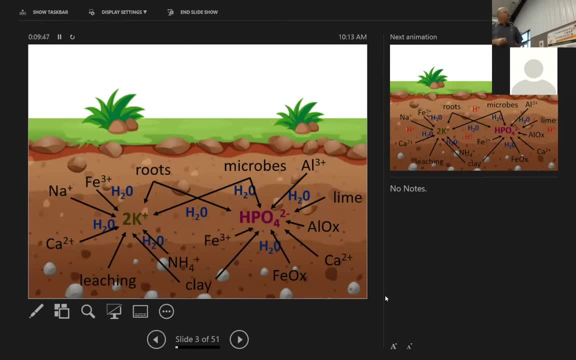 have that cation exchange capacity so it can be leached out, Generally not a problem with phosphate. So here's kind of the conceptual picture of this ion war scenario that I'm trying to set up. Questions, Comments- You probably already know all of it. 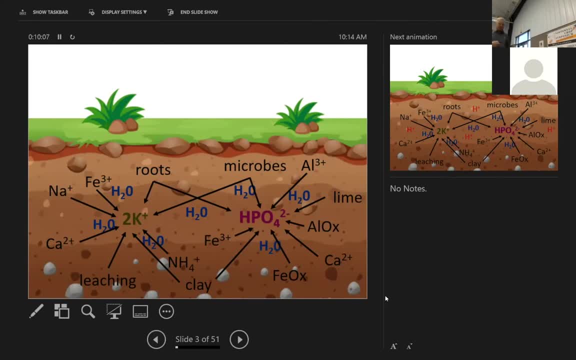 but kind of want to kind of set things up a little bit. Okay, Jeremiah, I don't know if there are comments online. if you want to give a shout, Okay, I will try to remember that. All right, All right Now one more thing I forgot I had on here. 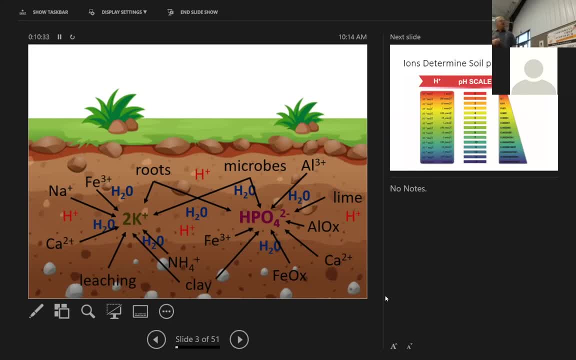 We're talking about pH, So I've got these red hydrogen ions in here as well. That's what pH is is how much of that ion is in the soil. In high pH soils it's very small amounts. In low pH soils. 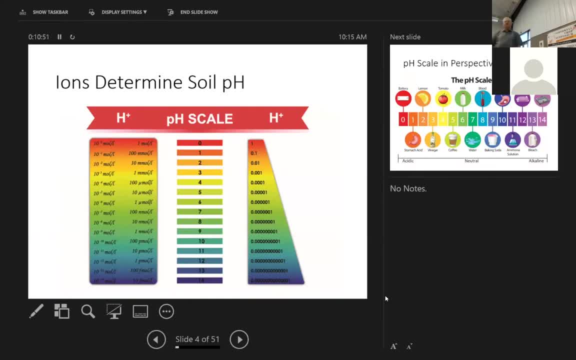 that gets to be a problem. Okay, All right. So pH scale. Just really quickly. Just a reminder: we go from pH of 0 to 14 on the scale, And when we go from 1 to 2 on that scale, it's not just doubling the amount of acidity in the soil. 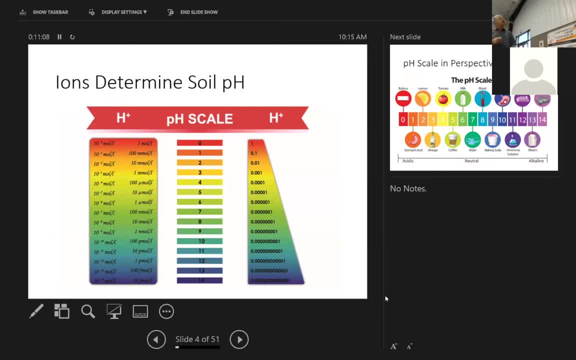 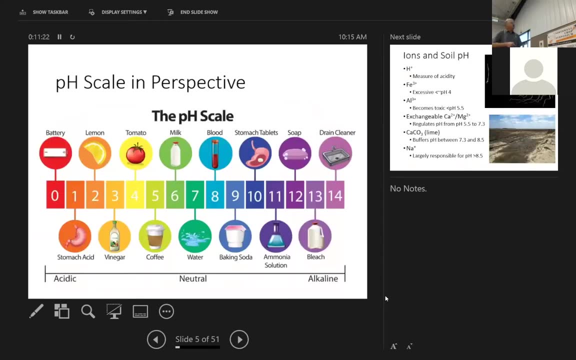 It's 10 times, you know. So it's a log scale. So actually the amount of acidity goes down. Sorry, I got that reversed there. It goes down by a factor of 10 to each one. So pH unity actually quite a lot, All right. So what does that mean in terms of everyday things? I don't. 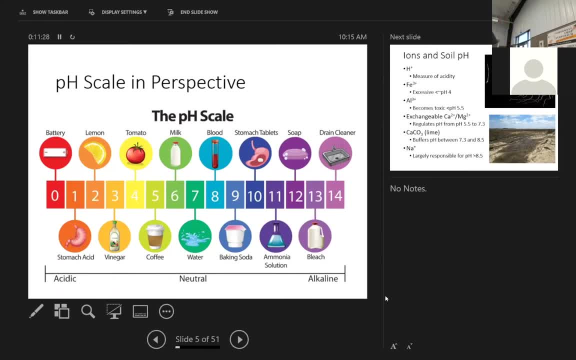 want to go over all of these. You've probably seen this pH scale from 0 to 14.. Basically, we've got water in the middle That's neutral, And we've got things on the outside- Battery acid and drain cleaner that burn you, And then some variation in between there. Okay, 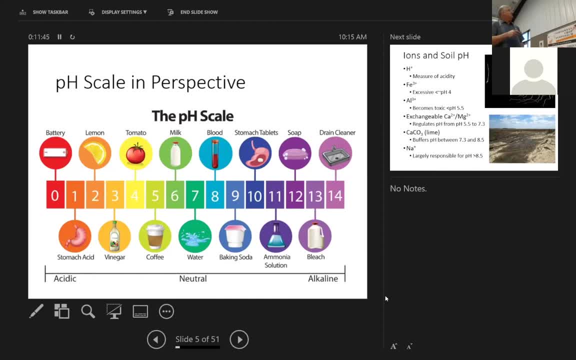 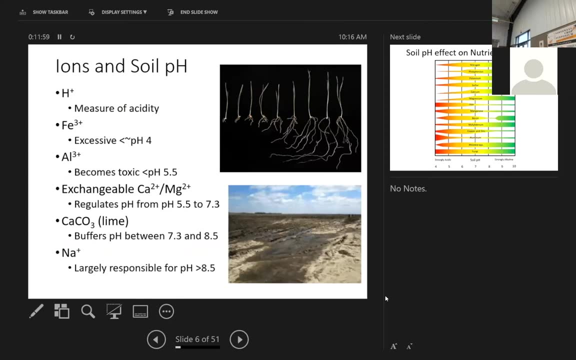 Our soils are generally, you know, in this probably 4 to 10 range And ideally more in the 7.5 range. Okay, All right. So let's talk a little bit more about ions and how they impact soil pH and how that impacts crop production. So, as I mentioned, when we're measuring pH, 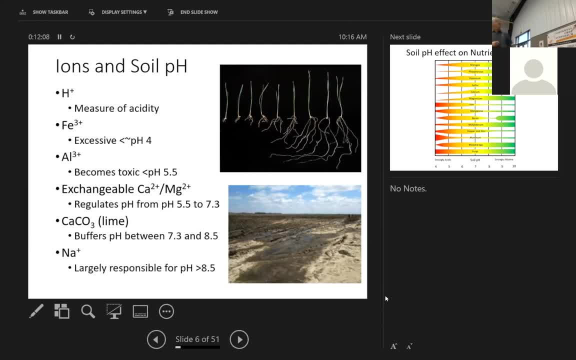 we're really measuring the hydrogen ions Okay, But that affects a whole lot of other ions in the soil, So kind of going from the extreme of an acid soil down to a high pH soil on my screen here, from top to bottom On the lower end, we can have too much iron in the 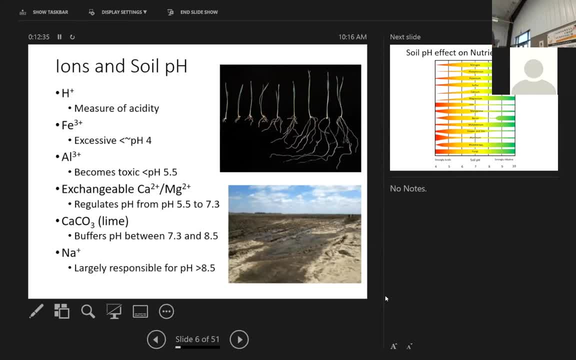 soil. We have a lot of iron in the soil but it's mostly tied up. But as we get down into pHs below 4, which I would hope we would never be and I don't expect we would ever be anywhere close to- 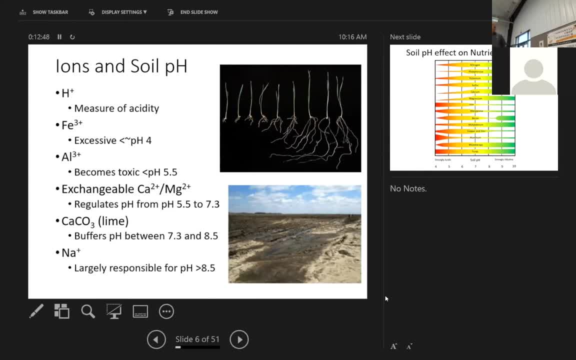 that here in the Bighorn Basin. But if we did then we would start to see problems with iron And that's a little bit more common, But again, not a problem here. There's aluminum in acid soils And there are some in Wyoming, You know. go on the other side of the mountain. 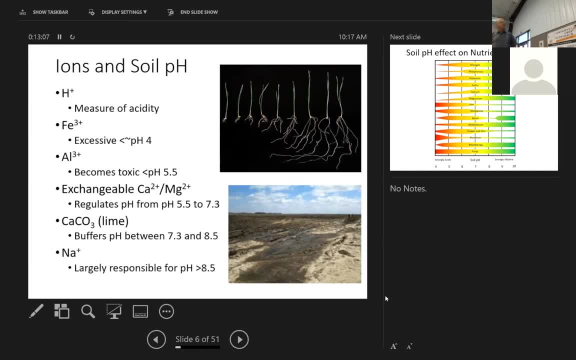 eastern Montana some sandy soils. you have some low pHs So it can be a problem. We have them in eastern Montana. But if we get down below 5.5, then aluminum, which is a constituent of the bottom of our soils- a lot of aluminum in this soil. it becomes soluble And aluminum is toxic. 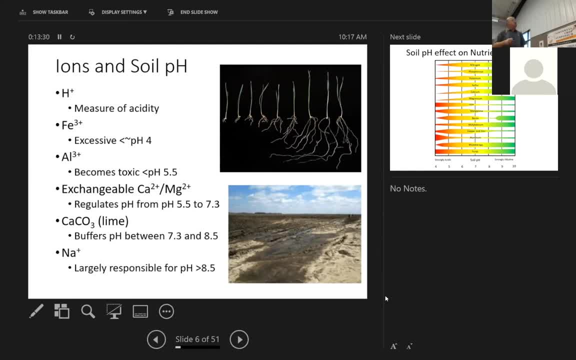 to plants, especially roots. Here are some barley plants on the top right looking at the effects of aluminum toxicity on the root system. So on the far right, normal root system, no aluminum toxicity. And as we get farther and farther to the left we get more and more aluminum damage. So it can have. 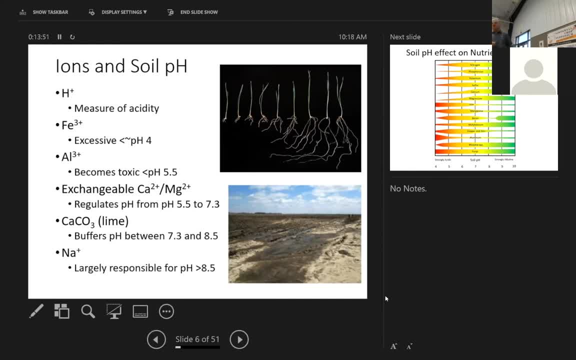 a huge impact. We don't want to have that problem. That's a bad one, All right. So let's get more into our range at the bottom of this table, Exchangeable calcium and magnesium, and primarily calcium, are what dominate our soils and determine what our pH is going to be. Now we can have exchangeable. 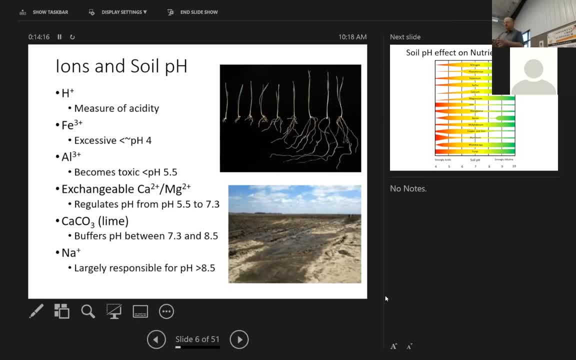 calcium, which is on those clay particles along with potassium and everything else, And we can also have free calcium carbonate in the soil. We have both. We have quite a bit of calcium carbonate And that can be a good thing and a bad thing. Calcium carbonate is a base. 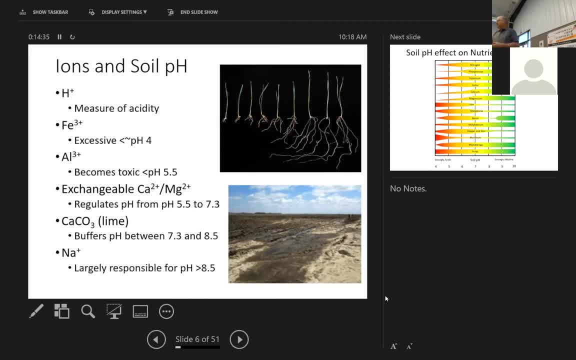 So it's alkaline, has a high pH. It's also a very good buffer. What that means is is that keeps the pH from changing a whole lot. Okay, That can be a good thing too. So, you know, we can have anywhere from a couple of percent to maybe up to seven, eight, nine percent. 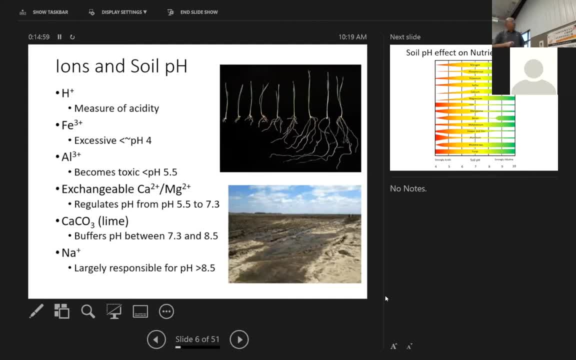 calcium carbonate in our soils. I'll talk about more about that in just a minute. So I said it's it's a buffer, So it keeps our soils between 7.3 and 8.5.. So for those of you who looked at the soil tests, does that kind of agree with where your soil test is usually in that range And we're usually closer to 7.8.. So we're in that range. It's a buffer. So I said it's a buffer, So it keeps our soils between 7.3 and 8.5.. So for those of you who have looked at a soil test, does that kind of agree with where your soil test usually fall? And we're mostly closer to 7.8.. So you can have It's a buffer that stays in that range. 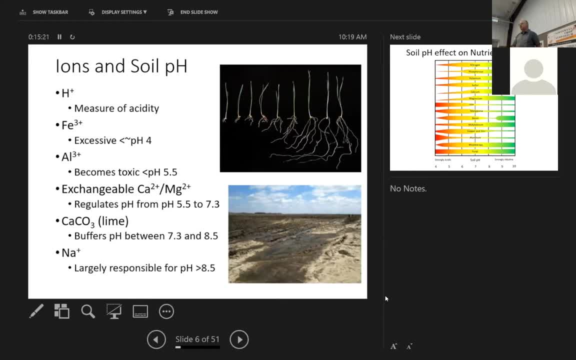 of our soils closer to the 7.8,, 8,, 8.2.. Can I ring a bell? Okay, All right. So as long as there's calcium carbonate in that soil, it's probably gonna be in that range. 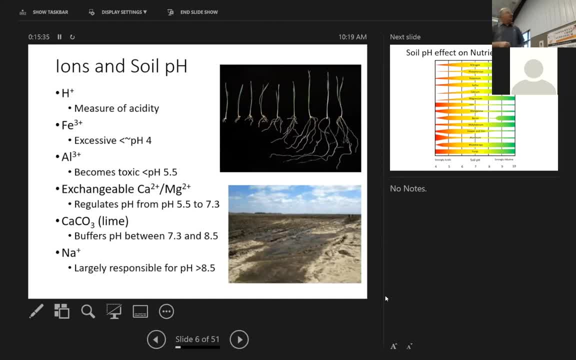 Now, if we get above 8.5, that indicates a problem that we have too much sodium And sodium carbonate causes a higher pH, greater than 8.5.. And that leads to soil problems that are kind of a mess. We call them a black soil or a slick soil- slick spot. 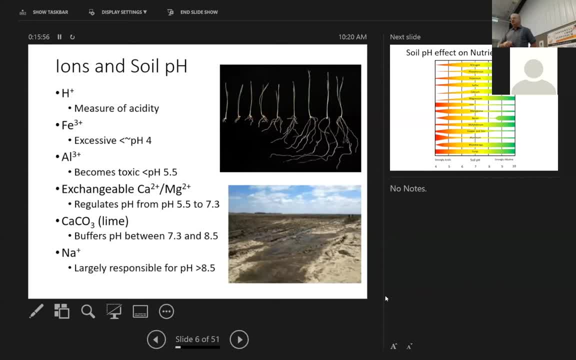 Just doesn't grain very well. nothing grows, Just kind of a muddy mess. It's similar to some of our alkali spots around here, And in our alkali spots we have a lot of other salts involved besides just sodium, So we get that white alkali on the top as well. 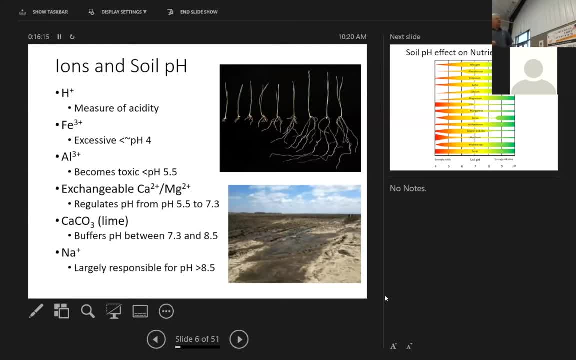 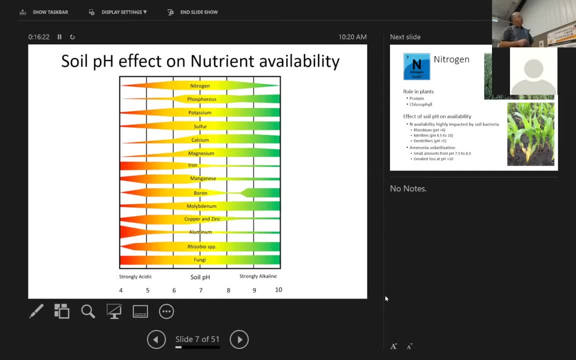 So we don't wanna go too deep into the soil. We want to go deep into the soil. We don't wanna go there either. All right, So let's talk a little bit about how that affects nutrient availability. If you've been to a soil fertility class, 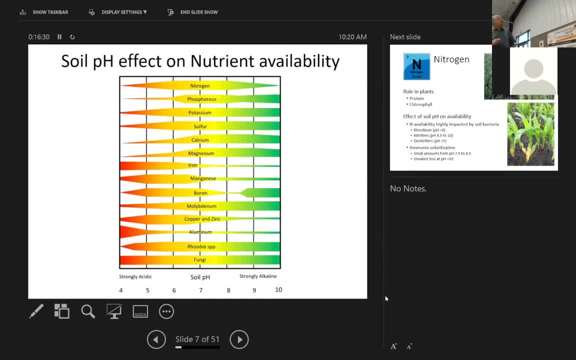 you've seen this graph for this chart. The wider the bar on this chart, the more available that nutrient is. So, as you can see, most of the widest parts of the bars are between about six and seven, seven and a half. So when you read about soil pH, 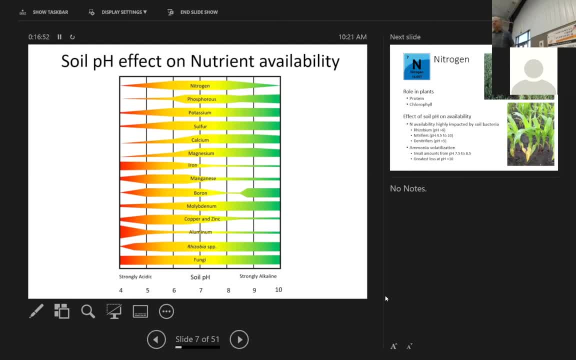 you usually read that that's the ideal range- six to six and a half- And that's largely because of this. But you can see that some nutrients become less available at lower pHs and some nutrients become less available at higher pHs And if we get into the extremes, 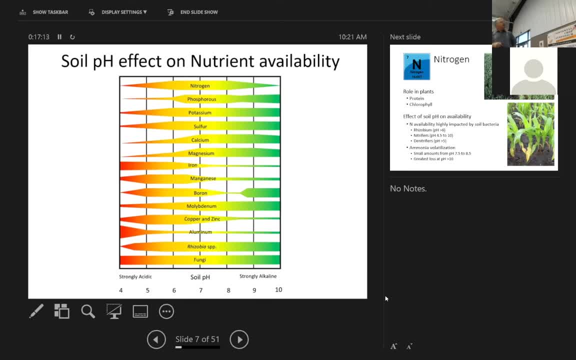 then it can cause some real problems. I've also got on this chart, a couple down here at the bottom, some microorganisms that are important in nutrient availability. Rhizobia is that bacteria that helps your alfalfa and your dry beans fix nitrogen. 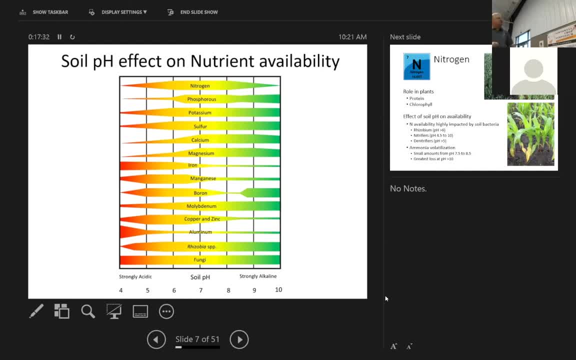 So that's an important one. And then we have fungi, and some other bacteria as well, that help cycle our nutrients. So generally, the fungi are pretty resistant to soil pH. Bacteria don't like the acid pHs, All right. So with that in mind, let's talk a little bit about some specific nutrients that are 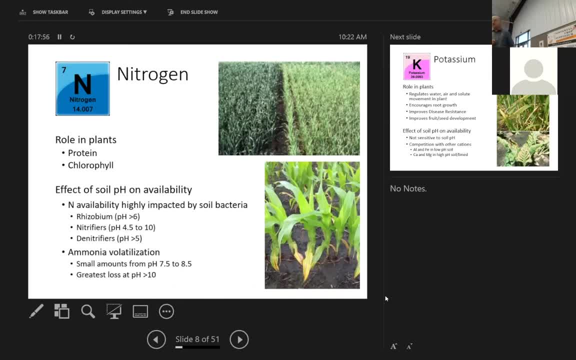 important to us and that might be affected by soil pH and some of the reasons for that. So let's start with the big one: nitrogen, one of our biggest nutrient input, and when it's deficient, it's obvious right. So why is it so important? 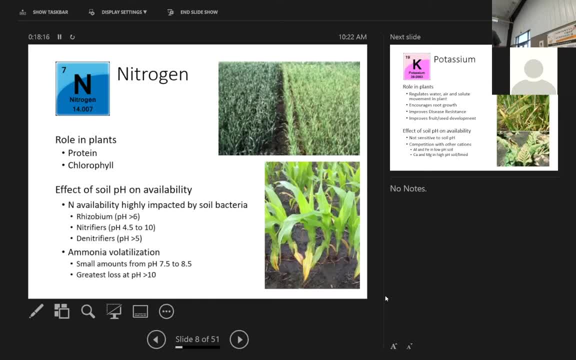 Well, it affects just about everything in the plant. It's a component of proteins and chlorophyll, and those are key to everything that goes on in that plant. So how does pH affect nitrogen? Well, it really comes down to that soil microbiome, those microorganisms in the soil that change. 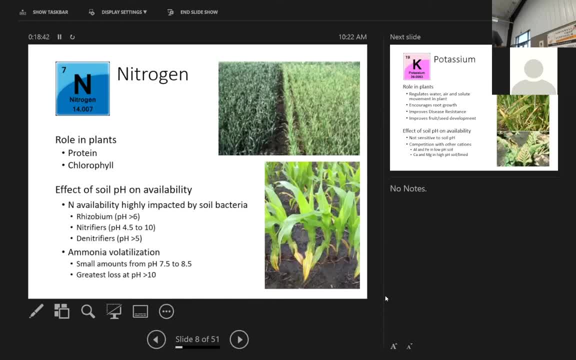 the form of nitrogen. I mentioned that earlier. It's in the rhizobium and we've got bacteria that change your fertilizer in into nitrate- if it's urea or hydrous ammonia if you have that- And nitrate is the form that plants generally take up, so that's an important one. 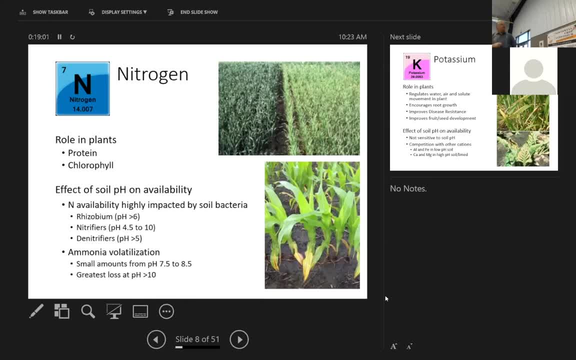 And if we get too acidic on both of those, then we have problems. But in our high pH soil that's not a problem. Now we can also have some problems with nitrogen. We can lose it, volatilize it because of nitrogen. 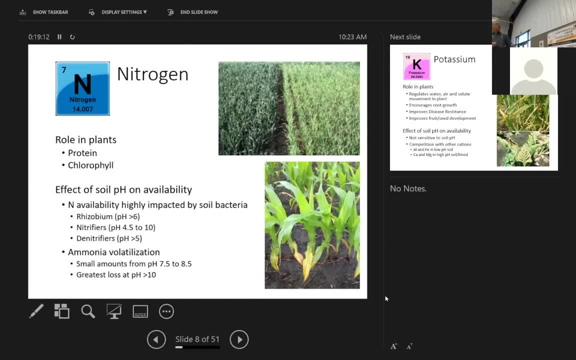 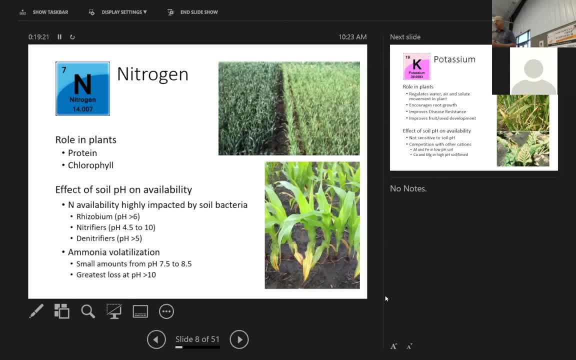 our soil pH is being kind of basic can be a little bit of a disadvantage because especially that enzyme that causes volatilization, that process of volatilization proceeds better at higher pHs than it does at lower pHs. The greatest one we get above 10, but really it can be pretty active in our normal soil. 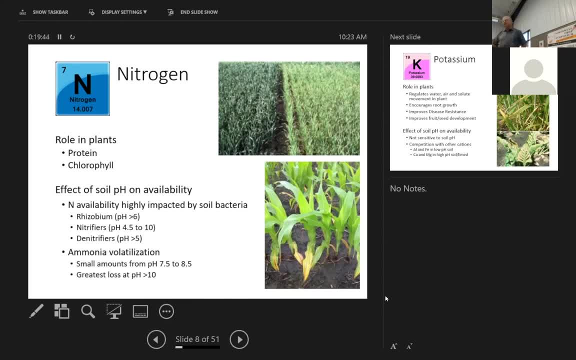 field change. So the key there is just to protect that urea. if that's what we're using it, incorporate it as quickly as we can into the soil and make sure that those conditions- for what volatilization losses- don't exist. Once it's in the soil it doesn't go anywhere. Questions on nitrogen. 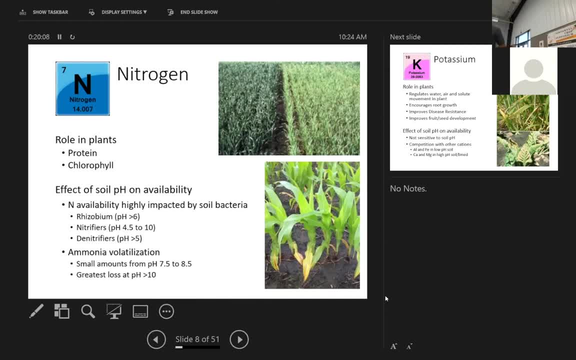 Pretty simple. yeah Well, if I understand your question right, you're asking about pre-plant nitrogen applications. how much to put on protecting against leaching or compensating for leaching? There are some products available that protect that nitrogen for a period of time. 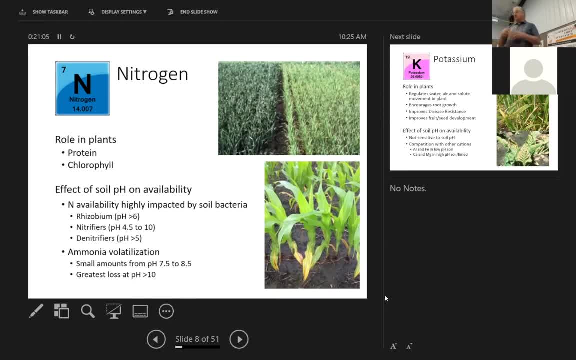 One is a polymer coated product that's just coated in a polymer shell that keeps that urea from reacting with the soil for a time and releases it more slowly for the growing season And that has has proven effective and oftentimes it's blended with regular urea because 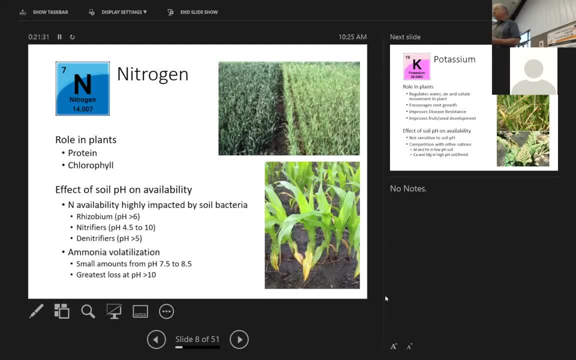 if it's all slow release then you might not have enough early in the season. So there's quite a bit of research on different blends- 50-50,, 75-25, whatever- on that kind of approach. So that's one thing. Here in the Binghorn Basin, one challenge we have is our dry climate and we can't rely on Mother Nature to germinate our crop most of the time. 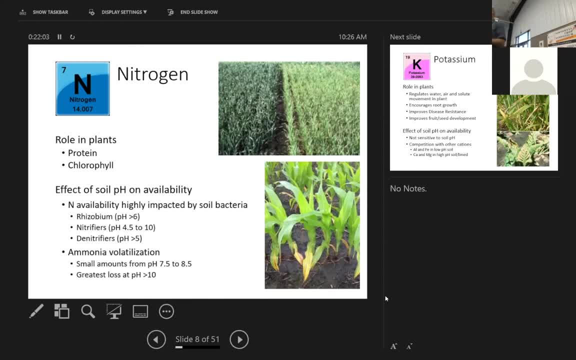 So we're really getting about takes a lot of water to do that, because I kept that soil out in the ground. you know, the problem with the soil is where can we get more water out of it? Yeah, it's hard. I've seen that on the soil, But we got a lot of different ones going around there. That's a big challenge. 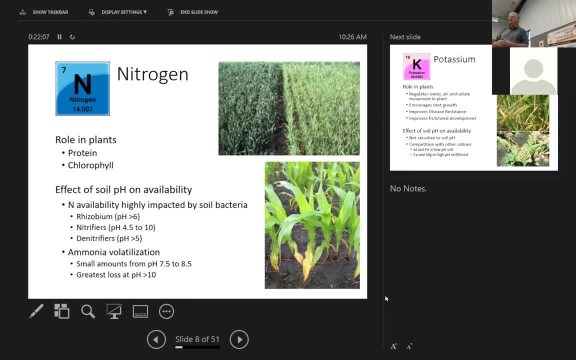 soil. I think that's where we get a lot of leaching if we have too much nitrate on pre-plant, So it is a little bit of a challenge. The polymer coated urea is one option. There are also products that we can treat fertilizer with, but they're supposed to kind of slow down their 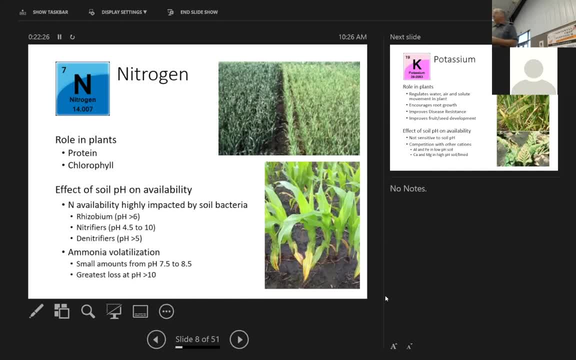 reaction and keep it from becoming leachable. Nitrate is the main form that we worry about. when it gets to that nitrate form it's most easily leachable. We've had for many years a nitrification inhibitor that kind of blocks that bacterial reaction and slows it down. 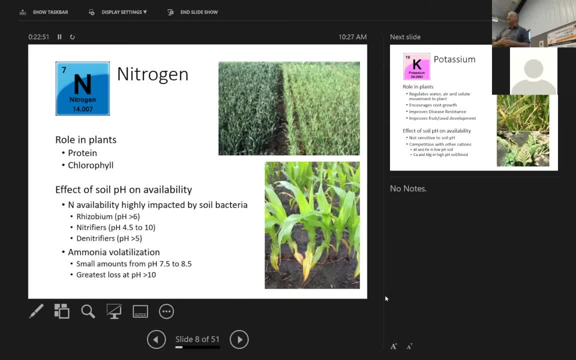 You need to remember about all those things that the weather dependent temperature especially. so the warmer the soils are, the faster that nitrogen is going to become a little bit. So one of our traditional approaches to it is to try to be more efficient with nitrogen and in this kind of a situation we put part of 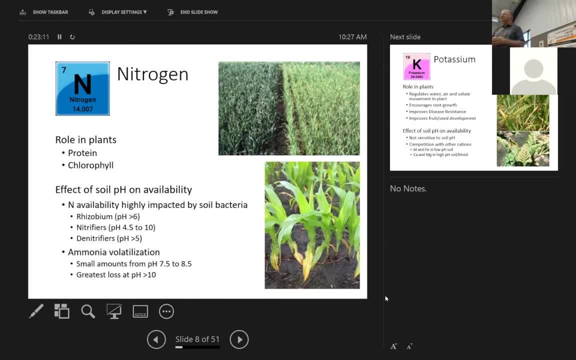 it on pre-plant and we leave it on in an extra fast crop field. But I do think we lose part of it with those pre-plant applications. I don't know if I answered your question adequately or not. Anything in particular you have. 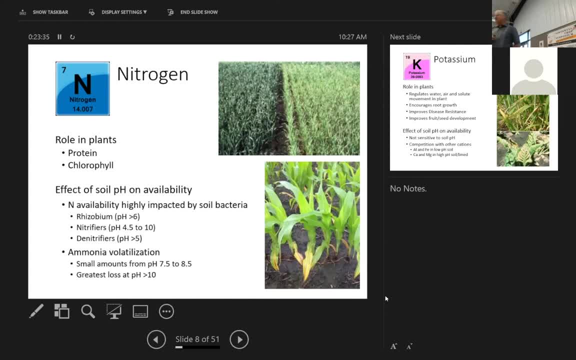 Another thing to consider. maybe if you put it in a band in a location that maybe is not going to be right under the furrow, Something like that might affect it a little bit in leaching as well. That might be a possibility, Mike. 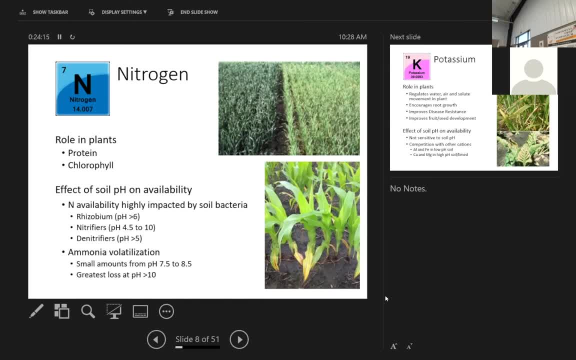 Mark, we're seeing more and more of the irrigation methods and, where my mind is going, I'll rephrase your question. So, with more fields going in, would you consider a greater amount of nitrogen? Would you consider a greater amount of nitrogen? 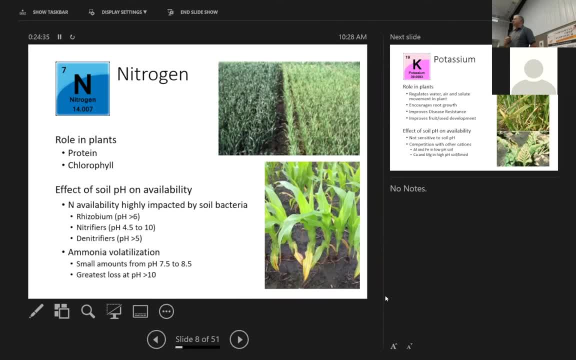 I have a question about that. Yeah, Good question. I hope everybody online can hear that. okay, The answer to your question is absolutely: With sprinkler irrigation we can keep that nitrogen where we want it more effectively. I had a colleague in the 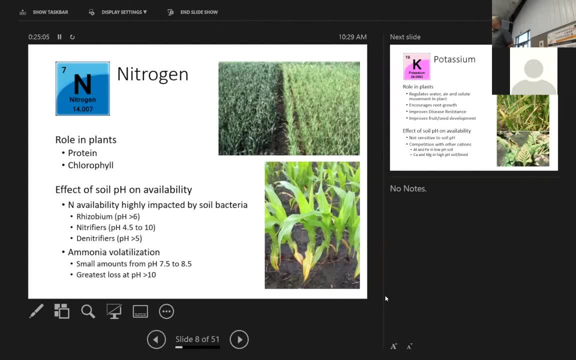 in Sydney with Montana State University who did a comparison for oil irrigation versus pink oil and nitrogen use efficiency, And they've shown pretty clearly that you get more nitrogen into the plant in the oil irrigation- sorry, regular irrigation- than oil irrigation. so yeah, 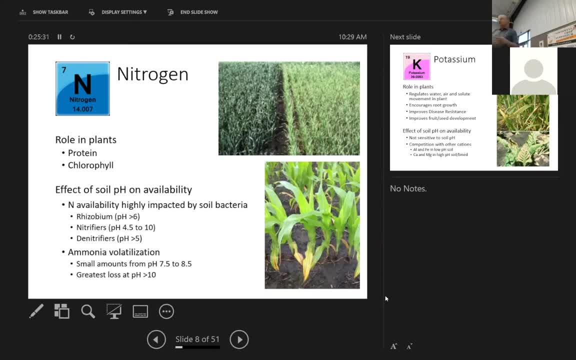 And in Sydney we don't usually do that. So that was another scenario where you know first the oil irrigation was at the plant, So you add in. you know you're getting up, But when you're putting on water with per irrigation, 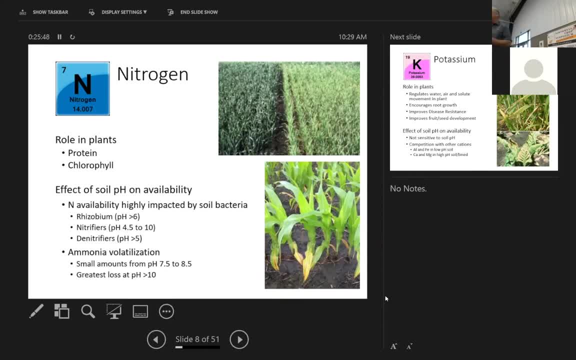 you're putting on lots of inches right Per acre And maybe even a foot or more with an irrigation, Whereas with pink oil irrigation you really can't do that. I mean, you're talking. it's probably less than an inch per application too. 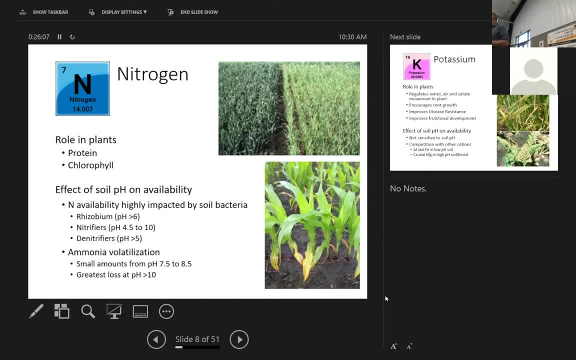 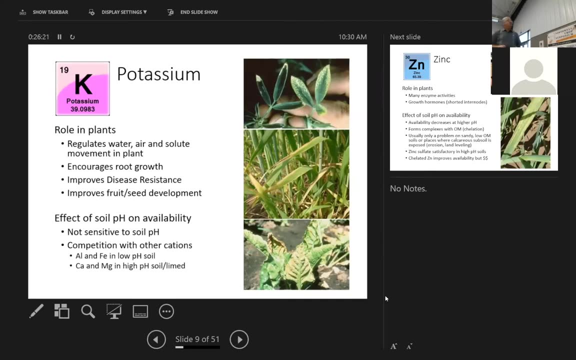 But yeah, that has a big impact in both protective and IPV. Another question: All right, let's move along here. Potassium's pretty, we can cover this one pretty quickly. Yes, it's important for these reasons that I've listed on the screen. 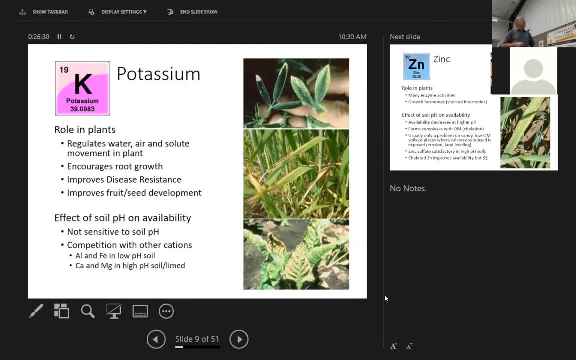 Does pH have an effect on potassium availability? Not really. Some of these other ions can have an impact, especially, you know, if we're adding lime to the soil, which we don't do a whole lot of here, but some I don't know if anybody's putting on too much lime here. 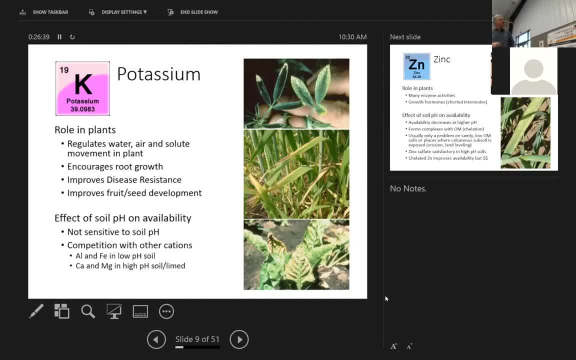 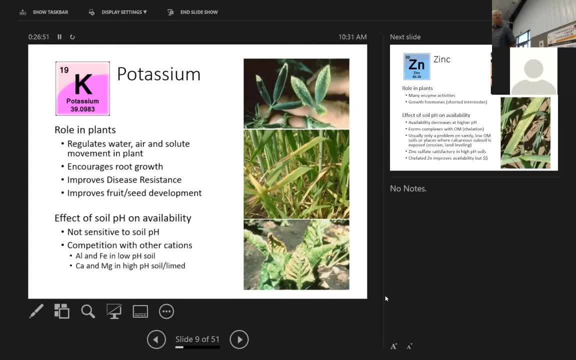 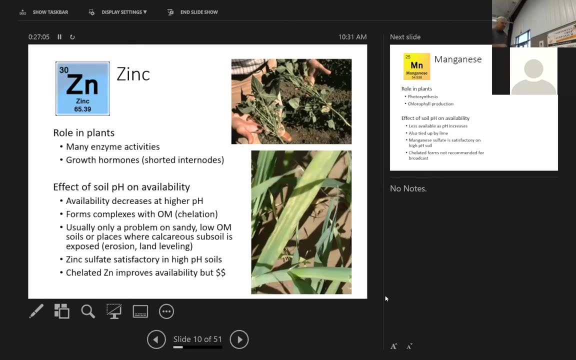 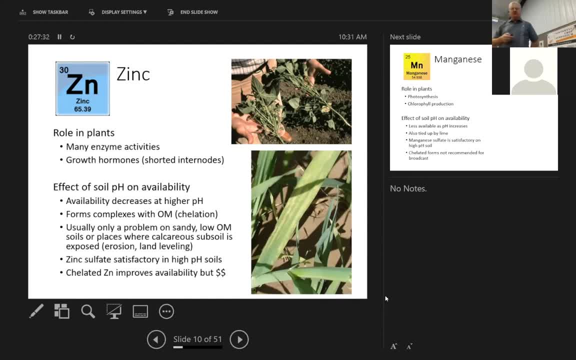 Thank you, Thank you. looked at all the different micronutrients and the only one that we really saw a response to is: we see that in eastern monocotana too, particularly with sugar beets and corn not so much. some of the small grains can be a problem with small grains- dry beans. 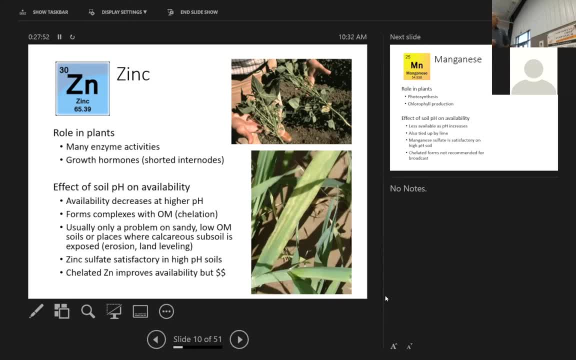 real important for dry beans, so it's an important one. does soil ph affect availability of zinc? absolutely. it will form unavailable compounds at high ph and becomes more available at low ph. it can actually become toxic if ph gets too low, so you don't want to go there. 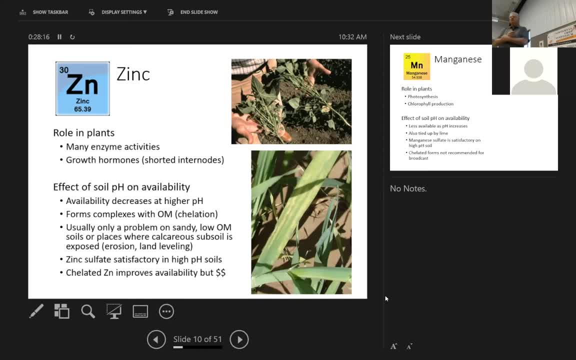 but really zinc is pretty straightforward. in my experience, zinc sulfates are a good fertilizer. it'll increase our soil test zinc levels and plants will be able to get it and it it'll stay available for quite a long time in the soil. it does react, but really pretty straightforward with zinc. 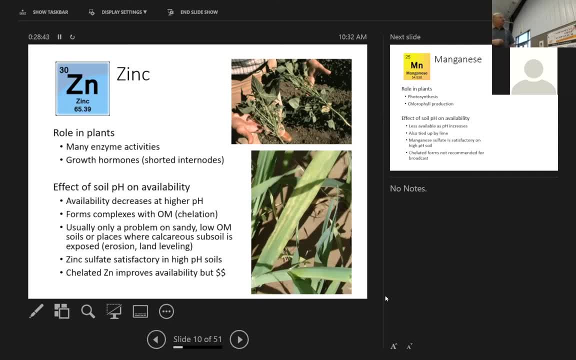 so it's satisfactory. i think our high q soils. we have to watch particularly on sandy soils, more organic kind of soils, or where you have some photos that close with zinc. so that's where we tend to see the most severe, because this is just symptoms, but we can definitely have some hidden. 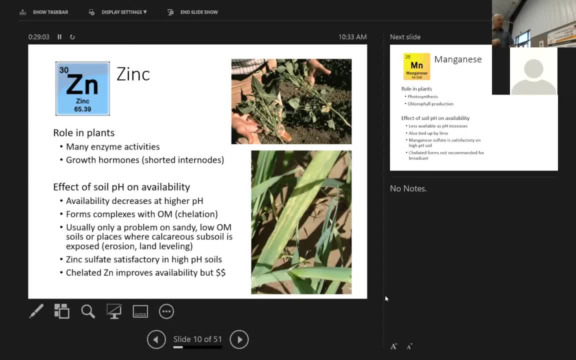 disease if you're not careful. we've got to watch that one now. what about chelated zinc? they're available for good products. their availability is better than something like zinc sulfate, which just is just the salt: pretty expensive, probably not practical on a broadcast basis. one of the advantages of chelates: 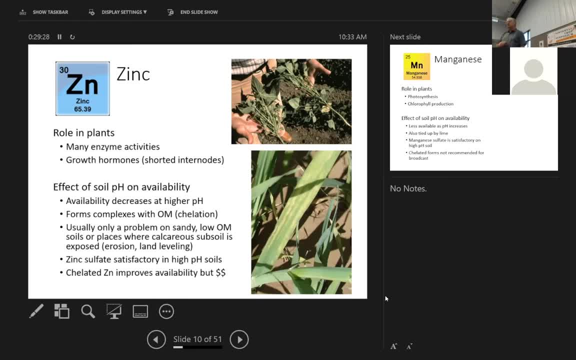 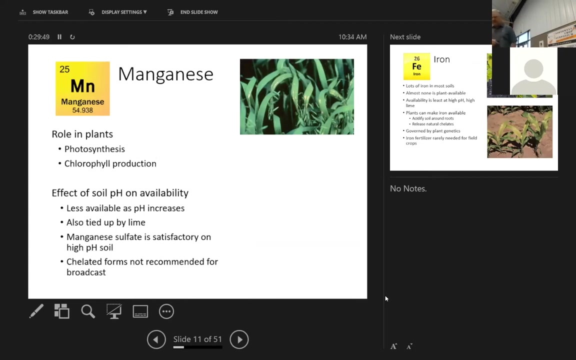 is they work well with liquid system. they mix well with just letting the other liquid fertilizer. so for starter fertilizer when per pop-up, if you're using a liquid, that's a great option. manganese: not a real big issue in my experience. when i when i was working here in powell, i did have one of the western sugar field. 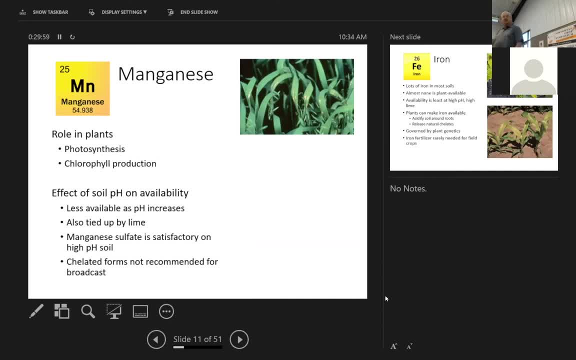 told me that they had a where they came across this really field that had some manganese deficiency and they put a little manganese on inside the problem. Effective pH similar to zinc, maybe a little bit greater effect than on zinc tied up by lime, but really manganese sulfate. 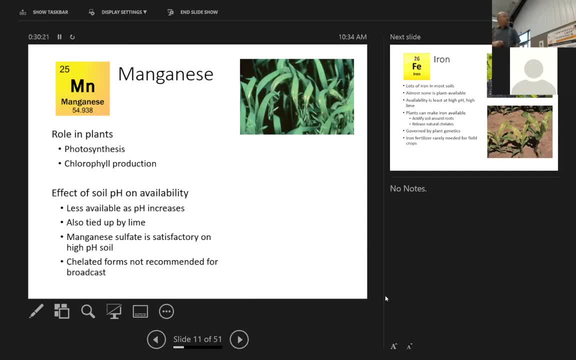 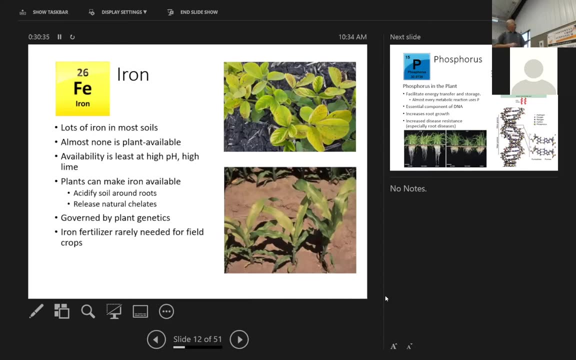 All right, let's talk about iron a minute, not because it's something that we really have to worry about here or we've managed, but it's. it's kind of a fascinating case to me. I did some research on it when I was in grad school. 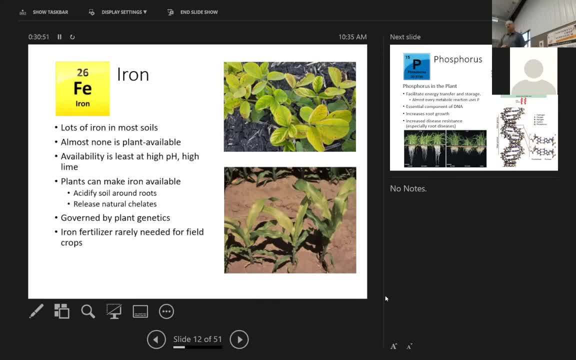 I went again at the University of Nebraska in west central Nebraska. There are certain crops where it can be a problem in certain soil types and these are real high, can be real high soil pHs or just typical talk area soils We get in soybean country and particularly in North Dakota. 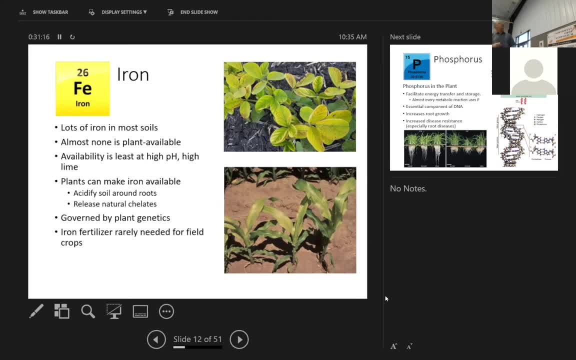 and Minnesota. you can have problems with iron deficiency and this is what it looks like, And then some some pretty high pH soils- it's about 8.5- probably can have problems as well. Interesting thing- interesting thing about iron is that iron is the fourth most abundant element. 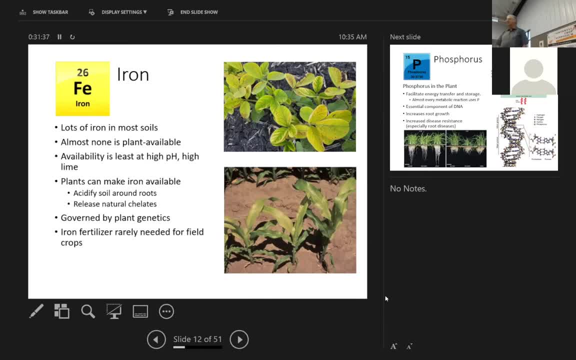 in our crop soil, in our earth grass, in the soil. There's lots of them, but, like I mentioned before, it's just. it's so insoluble that plants can't rely on. So what's fascinating to me is that mother nature has adapted and most of our crops, you know, we just. 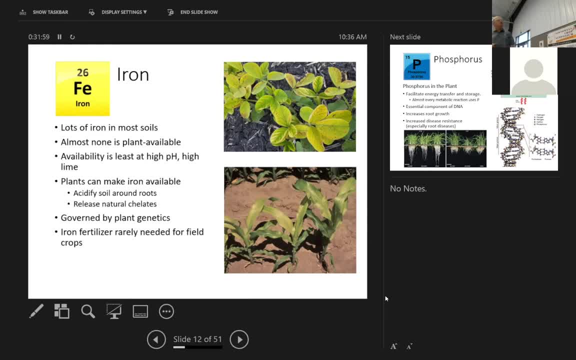 don't don't see a problem, and that's. that's more so because of the crop and the plant and its characteristics than the soil. Soybeans have developed the ability to to respond to low iron situation and they'll acidify the reed and then the soluble ions that are released- organic chelating. 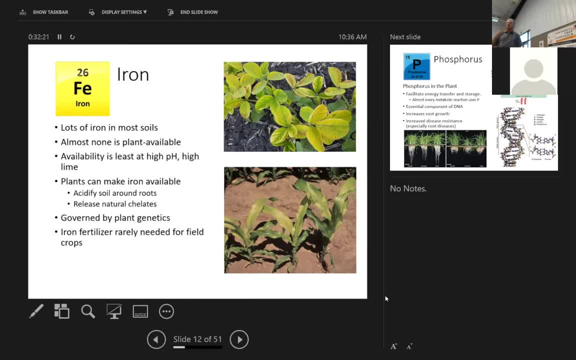 compounds that they produce to, to complex it and bring it into the reed. Now, that's a genetic thing. Some varieties have it, some don't, So that that becomes an issue in in those parts of the country where they have problems with that. Same thing with corn. It has a response, and, and every day. 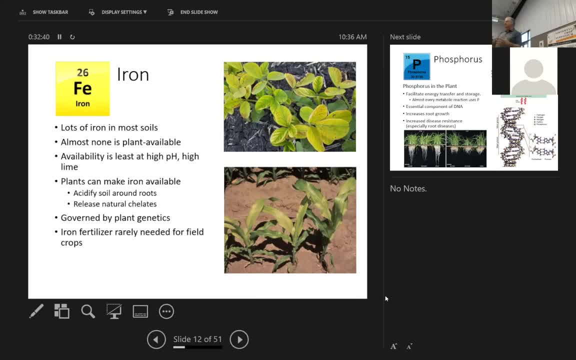 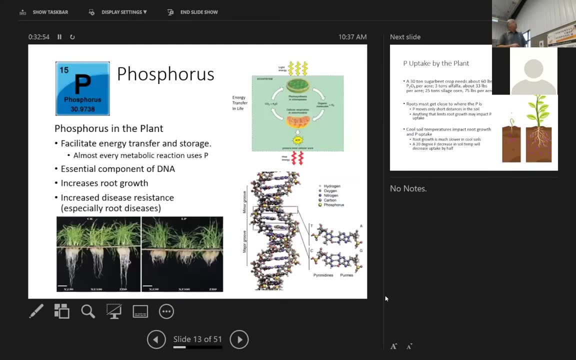 So just because the soil chemistry, that that ion warfing, is not in our favor, doesn't mean that that you're going to have a problem. All right, Questions on that, All right. Now this is kind of a big one, So I'm going to spend some time on this one. 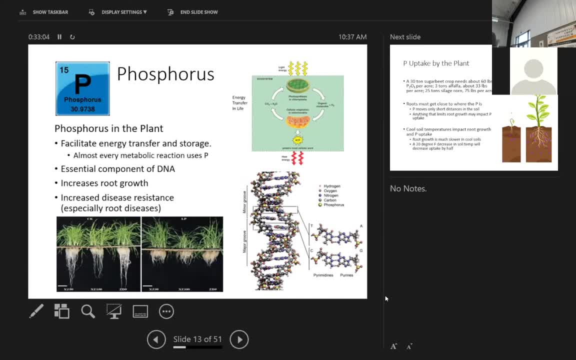 Let me get. let me know if I get too long-winded. I get a little shabby sometimes. Um, I know it's not easy to sit there on those hard chairs for a long time and listen to somebody talk. But, uh, anybody concerned about auspices? 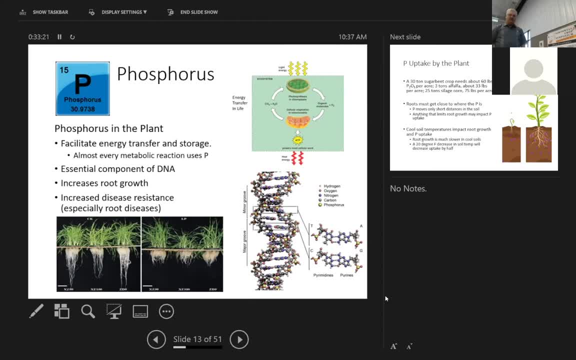 Well, going back to the days when I was on my my dad farm, um and I, I started becoming interested in learning more about soil science in college. First thing you have to do is: well, what can we do to to avoid kind of? and, and I think that 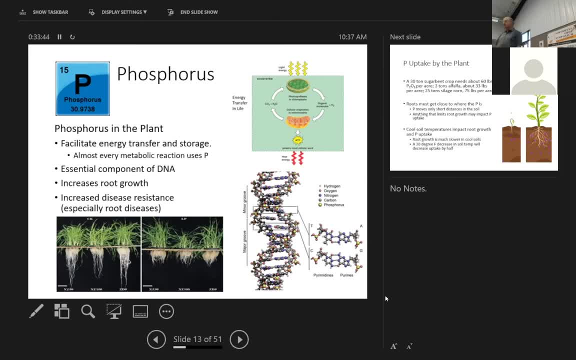 you know, it was certainly a valid question, Wasn't it? It is now No easy answer to it, But it's where it becomes more and more of a question, as our phosphate fertilizer goes from five to ten dollars a ton to 11 million dollars a ton. Right. 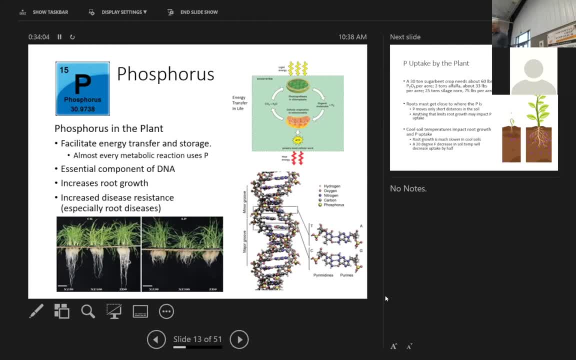 So let's talk a little bit about it. Let's add the silver bullet. Osiris is critical to the plant. It's involved in, you know, almost like nitrogen, involved in just about everything, but in a different way. Um, first thing is it, it's the currency that the plant uses to move energy. 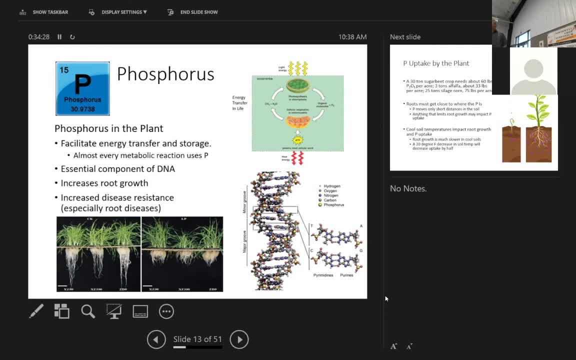 Um, you're familiar with a process called photosynthesis. Probably can't see that very well, um, from back there. but uh, here's a chlorophyll, a chloroplast. absorbed light energy produces a carbohydrate. It's a complex molecule that can just capture that sunlight energy. Okay, we rely on that too. 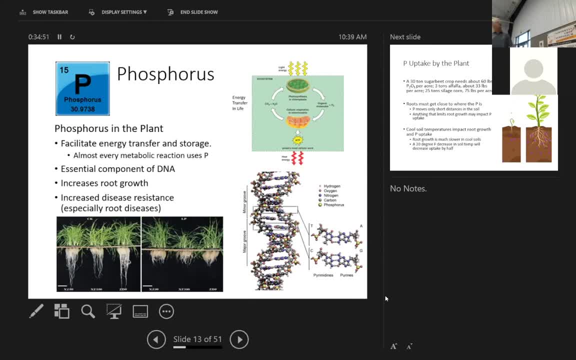 We rely on plants to get that energy from the sun, which is pretty cool, I think. All right. so the plant actually uses that the same way we do to support its growth, goes through the respiration process, which is the same process. There's a little mitochondria there. Plants have, we have. It transforms that, that sugar molecule. 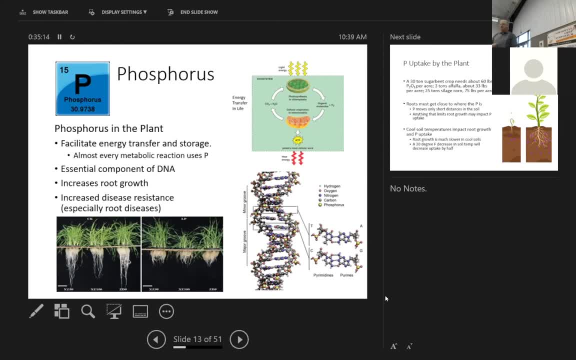 into carbon dioxide and water and energy. It releases that energy and then in that process it shoves it off to a molecule called adenosine triphosphate. That's three phosphate ions in it, And those three ions are bound together with a real high energy bond. 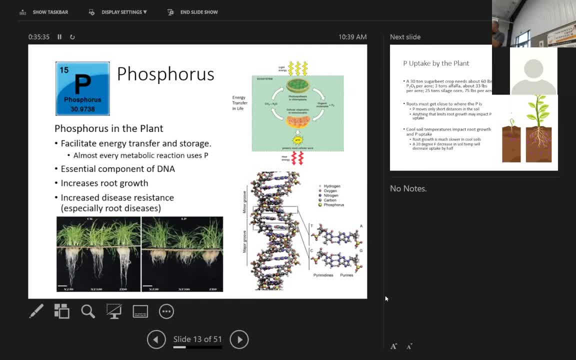 So when one of those is gone, it has the potential to add a third in it. So when there's two, you can add energy, another phosphate, and you capture that in, And then that plant can move that around throughout its structure to wherever it needs it. 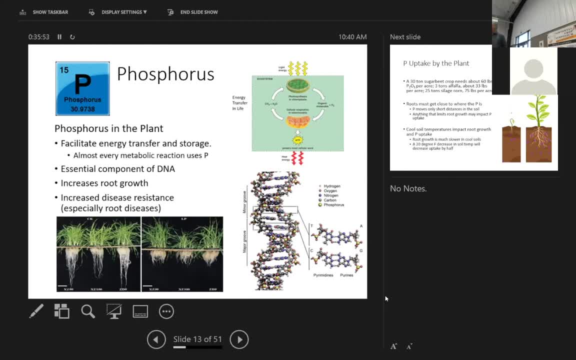 and provide energy to all the other processes in that plant. So without phosphorus- this is why the plant didn't have that energy- It's kind of stunted right. If you have phosphorus deficiency- they just don't grow very well. 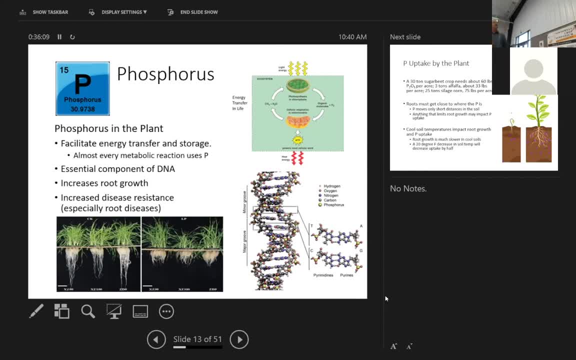 That's part of it. Now, the process also generates heat. Just as an aside, if anybody has a, When we harvest the beef and put them in a pile, that is still a living plant, right, And it still respires. 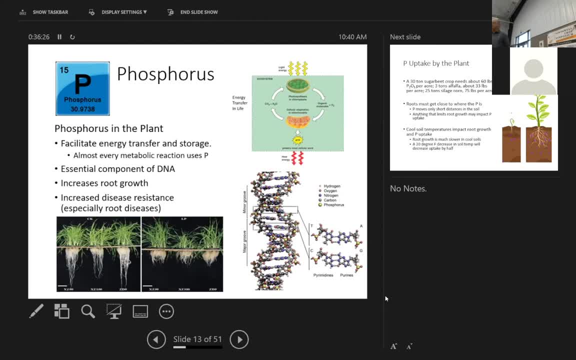 And if it respires too much, then that generates too much heat. You get a hot clot and that's when you start to get rot in the plant. So, same process, All right. so the other essential role that it has in the genetics of the plant. 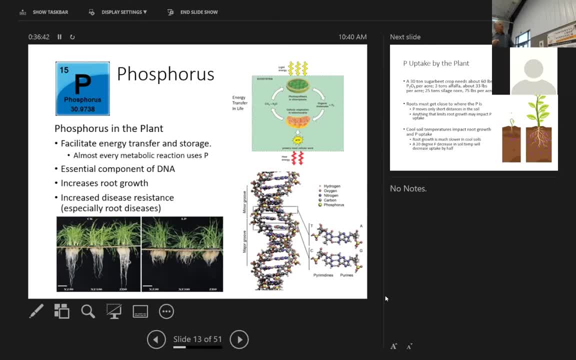 it's a part of this DNA backbone, So here you can see here the components of DNA and phosphorus. There's an important one, and it's here in these side genes here, So that's pretty important as well. All right, so phosphorus impacts root growth. 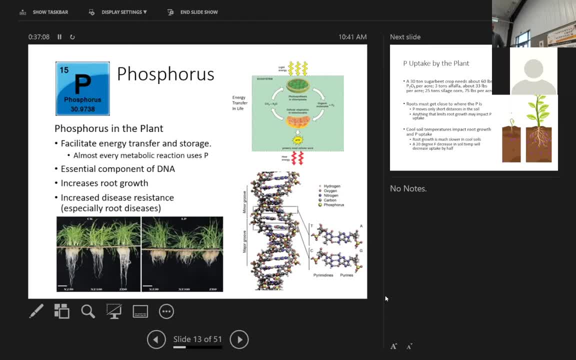 Show that on this image here at the bottom. This is a hydroponic study, Barley, I believe Roots here on the left where there's adequate phosphorus, And roots on the right where there's not. But there's also a genetic impact here as well. 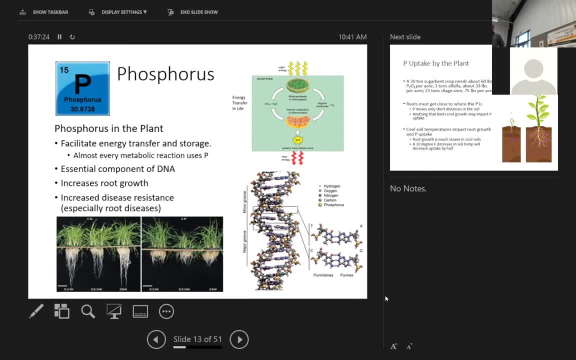 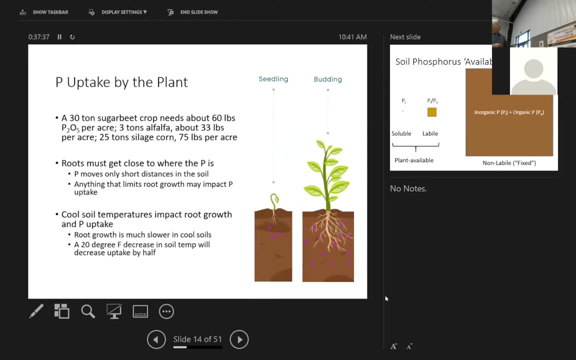 Some plants are more able to survive on lower levels of phosphorus. This one in the middle on the right is not One that is particularly efficient, So that's a factor here. All right, so how do we get that phosphorus into the plant? 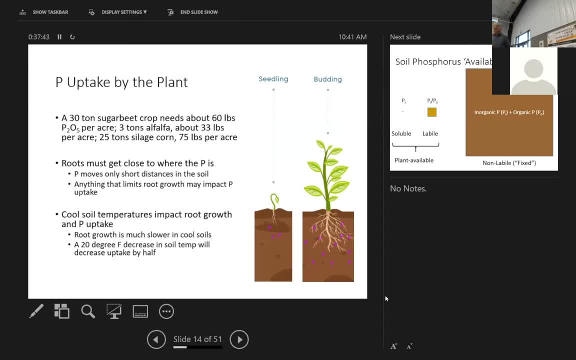 First of all, how much- And we're talking quite a bit- of phosphorus- that our crops will need. A crop of 30 tons will need about 60 pounds per acre. A half a crop: 32 pounds, 25 tons of size. 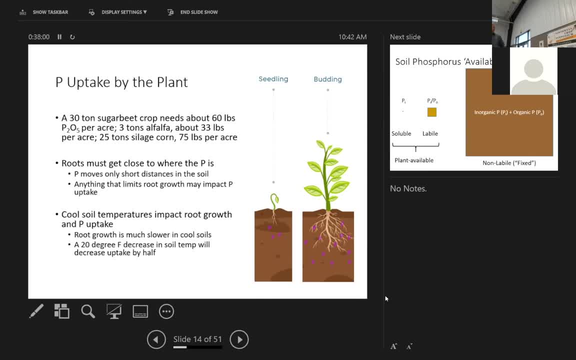 So we do need it, or the plant does need it in fairly large amounts. Now, the thing about phosphorus I mentioned before is it doesn't move to the plant, It stays where we put it. So the plant's got to go get it. So the plant really depends on expanding that root system to explore more of the soil profile or at least get to where the fertilizer is to get that phosphorus. Anything that restricts root growth is going to also restrict phosphorus Compaction Over the wet soils. 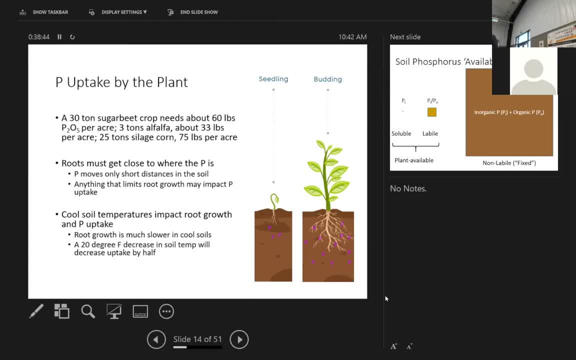 Indeed, you can think of that. So it's going to impact the root, the cultivator, which is something that I've got to be able to get at. So that's something to keep in mind. And also, roots don't grow very well. 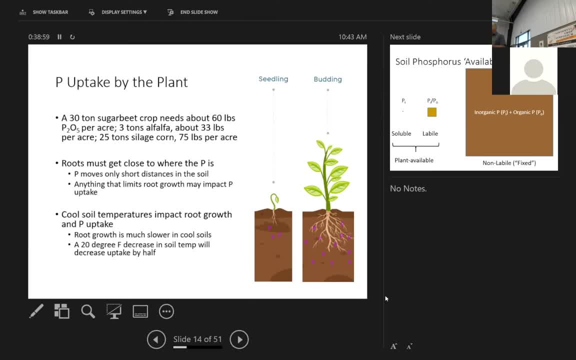 And then the phosphorus reactions and movement in the soil isn't very fast when the soil is acute. So when do we typically have the most problems with phosphorus efficiency? Early in the spring, small root system, cool soils. So that's why. 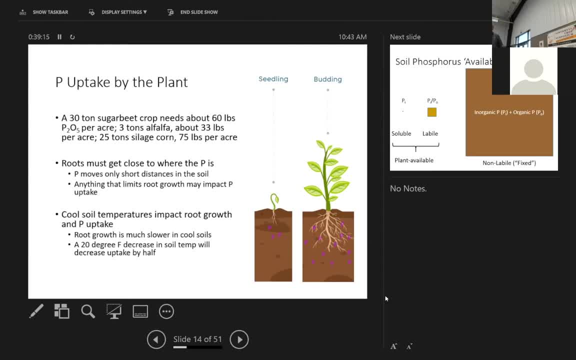 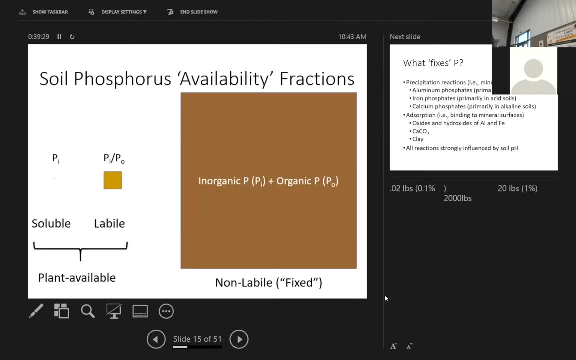 Fertilizers can sometimes be helpful. So a 20 degree decrease in soil temperature will decrease phosphorus. So let's talk about this phosphorus fixing problem. You can divide phosphorus in the soil into three different groups. It may look like there's only two there, but there's actually three. 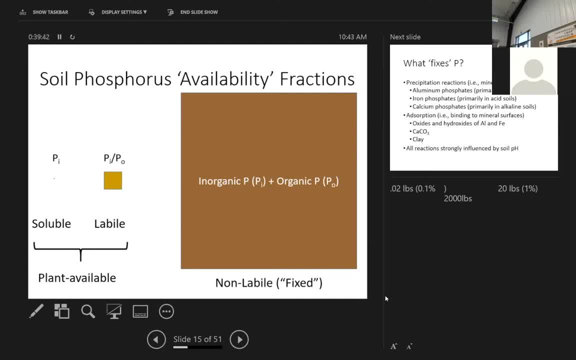 The main one is this one that we really don't like. The vast majority is in what we call non-labile forms, or fixed forms. That can be largely in our soils- inorganic- but our organic matter also contains some of that, And the organic tools are a little more readily available than inorganic, but they're both considered non-labile- non-labile easy for me to say in general. 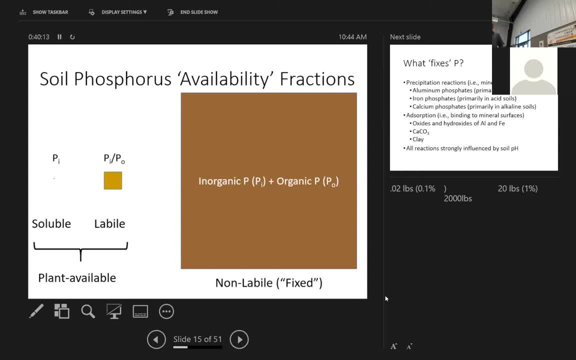 Now we have some exchange between that, So that group and this group. this is what we call the labile fraction, not necessarily in the water and ready for the plant to pick up, but easily accessible. okay, That can be both organic and inorganic, primarily inorganic. 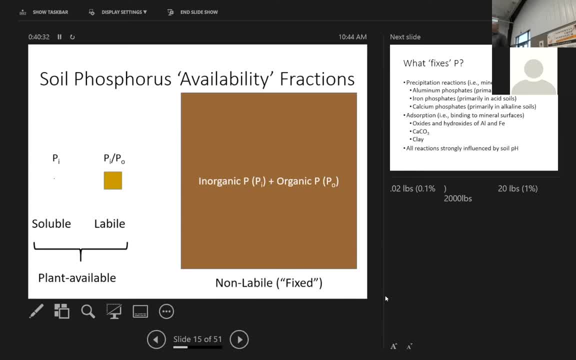 Now, the one that you probably can't see very well is that little dot, And that's the form that the plant can actually pick up into its group. So it's the ions. So they're in very, very Low amounts comparatively. 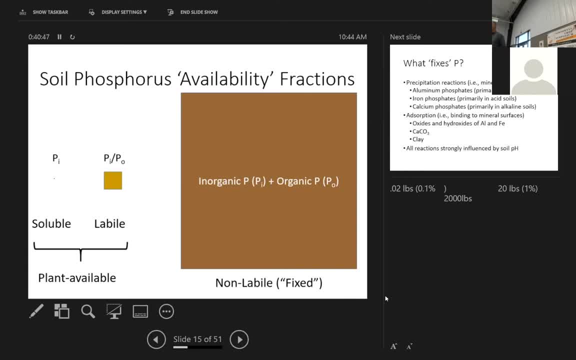 And that's the form that we put the fertilizer on. So we think of this process of putting it on in this form. It goes up this chain and it gets locked up in here. You know, that's kind of our concept of fossilization, right. 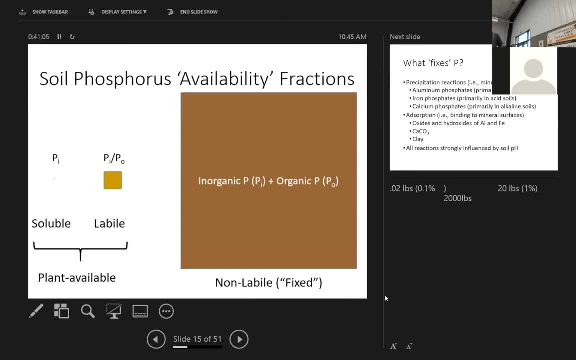 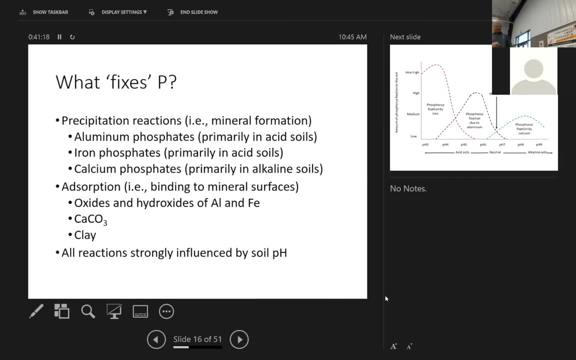 Well, it definitely goes in that direction strongly, but it does go in the other direction. But I hope to show you a little bit of information that shows, Once it gets in this form, it's not necessarily lost, okay? So why does this happen? 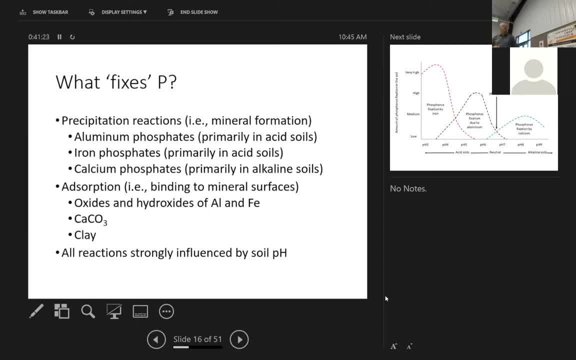 I've already kind of talked a little bit about it. We've got different chemical reactions in the soil with those ions: aluminum phosphates and iron phosphates- Not a problem here, so much Calcium big problem here, And it'll also be attracted to the surfaces of different things in the soil. 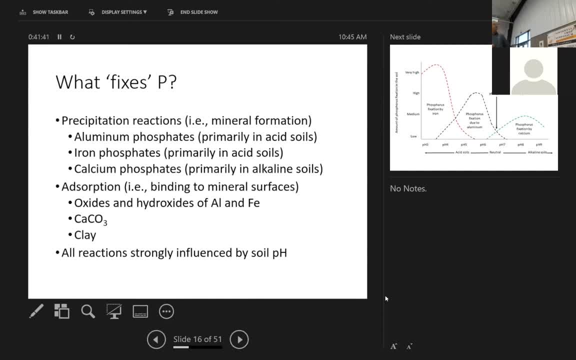 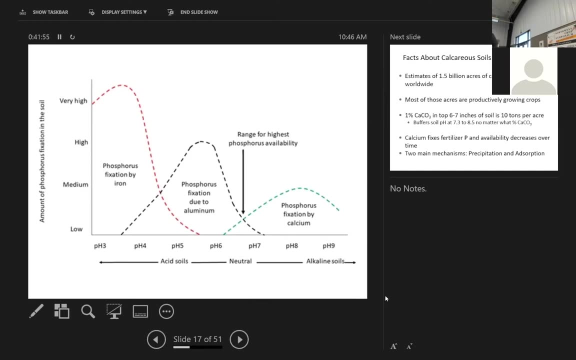 I'll show you some pictures here in just a minute. Calcium: It can absorb some phosphorus and play into the same thing as well. All right, So all these things are pretty strongly influenced by soil pH, And this graph, I think, shows this very well. 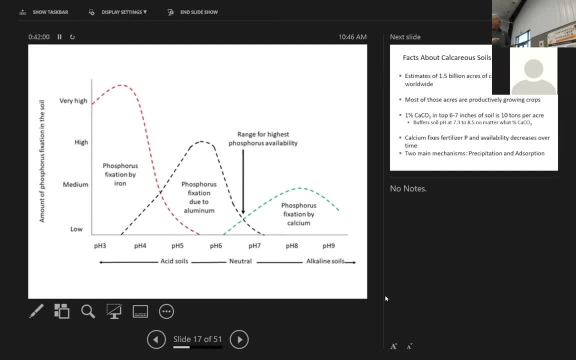 It's very general. Maybe you've seen this before. The soil pH across the bottom of the graph, So neutral soil, is in the middle. pH is 67.. Acid to the left, alkaline to the right. All right, So here's that sweet spot. 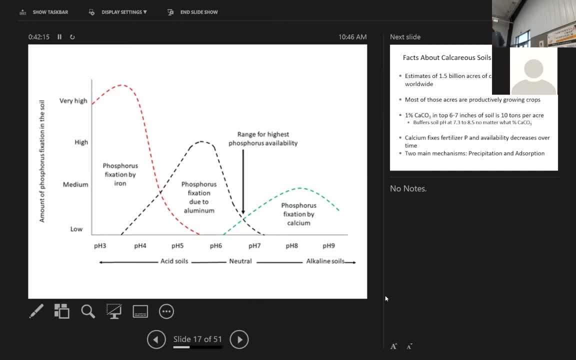 Six to seven. Now, these different lines show how much phosphorus is tied up, the phosphorus fixation in the soil. Okay, And this in general term: low, medium, high. All right, So you can see where that ideal range of pH comes from. 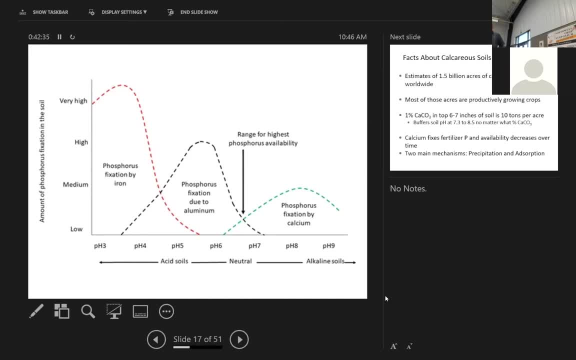 That's where availability is the highest. So you get up into RPA range around eight. I don't know where we see the most Calcium fixation, which you know doesn't look very good when you look at it. But you know that's just the nature of the beast. 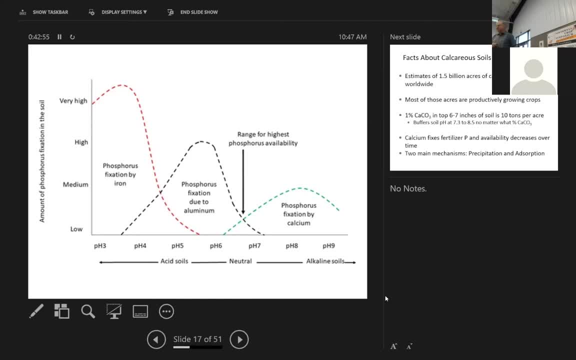 So what else do you notice about this graph? Our soil is the worst case scenario, Not even close right. You get down into these acid soils and, you know, start getting tied up with aluminum, You know. And iron half is really not that acidic. 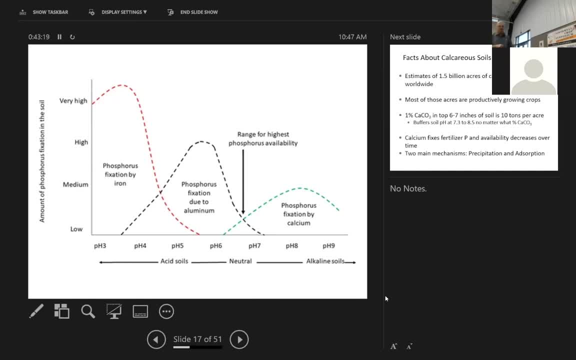 And if you get into the really low levels, you get iron. So I guess my message- and I'm going to hit this again- is: you know, we have some tie-up. It could be worse, You know. That, of course, makes us feel better. 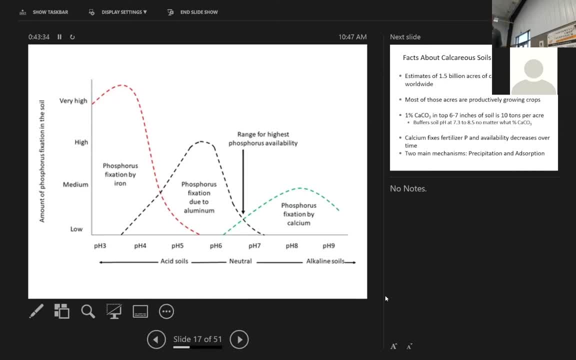 Absolutely So. today we're going to talk about phosphorus. We're not going to take it from the planet's side. We're going to take it from the planet's side, All right? So if I don't get back to that, so the question is about how long it takes. 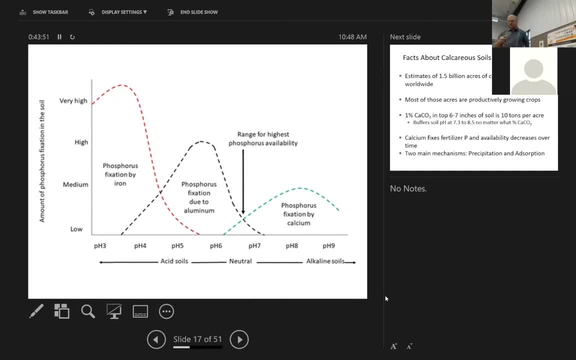 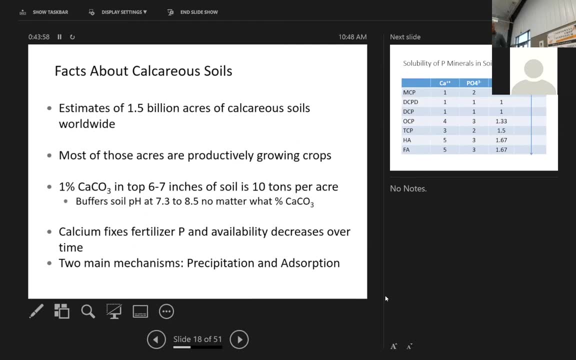 If I don't address it, please call me on it, All right? So let's move on a little bit here. So, calcareous soils: you know we look at them as a bad thing. They have their disadvantages but also their opening advantages. 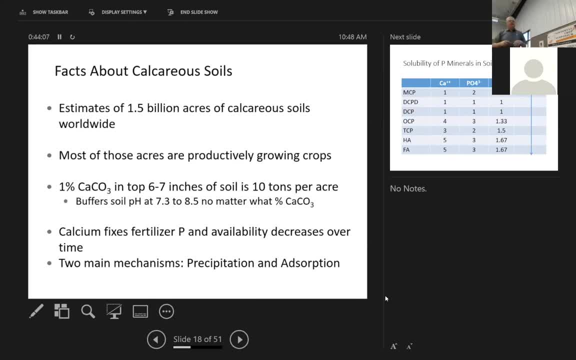 So, looking at that low case- let me hit on this here for just a minute- Um I, I, I did some of my education in Illinois. Those originally were pretty neutral soils But didn't have much calcium carbonate in them. you know as they developed. 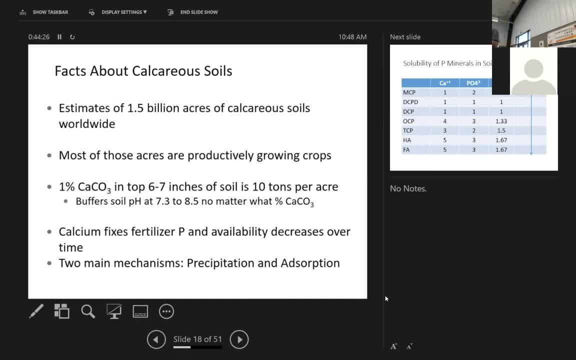 Started farming them. What do you do when you're growing corn, Lots and lots of nitrogen fertilizer right Every year, Unless you're growing soybeans in rotation then every other year? Every time we put on a nitrogen fertilizer, we're acidifying this. 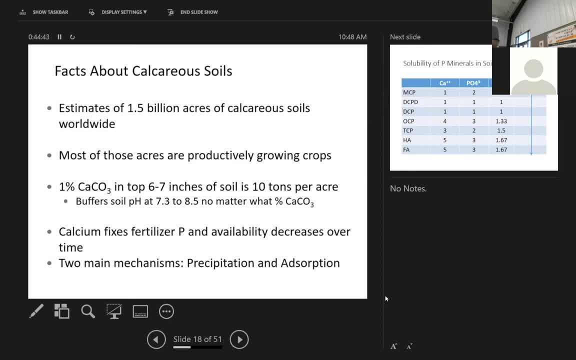 You don't. You don't see it in the future because of that calcium carbonate. But every time you put nitrogen fertilizer on that process of it being nitrified, um acidifies, causes an acidified gene. So it's going to neutralize some of that calcium carbonate. 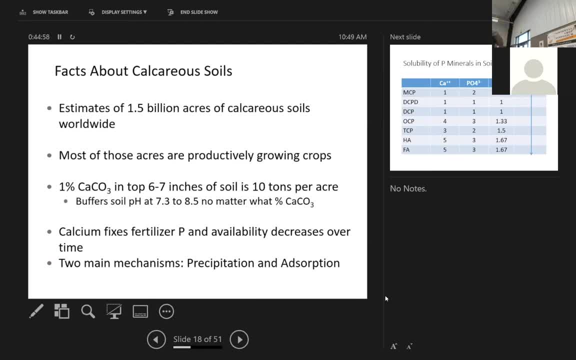 It's going to get rid of some of it And some of it flows into Montana with lower amounts of calcium carbonate and how we've been doing no-till wheat production for our land for years and years, continuously. we're seeing. So what do they do when they start having that pH drop up my line, five tons an acre? 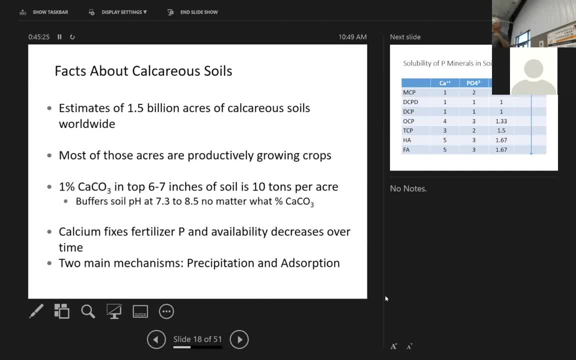 10 tons an acre. what's the one percent? okay, if the one percent calcium carbonate in our soils, the top six inches, which usually weighs about 2 million pounds, 1% of 2 million pounds, about 100,000, 20,000.. 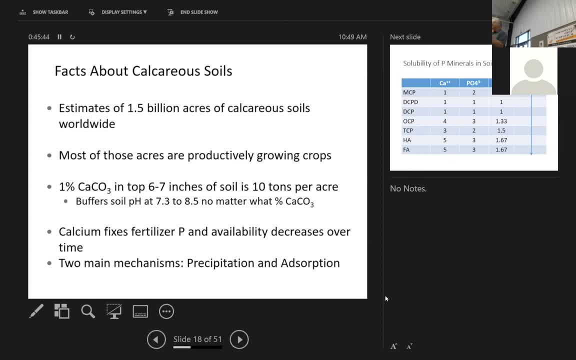 So if you have 10% calcium carbonate, think of all that lime that's already on the soil that you didn't have to put there. I don't want to overlook that. So most of these top layers are relatively productive. Yeah, pretty nice productive soils here. 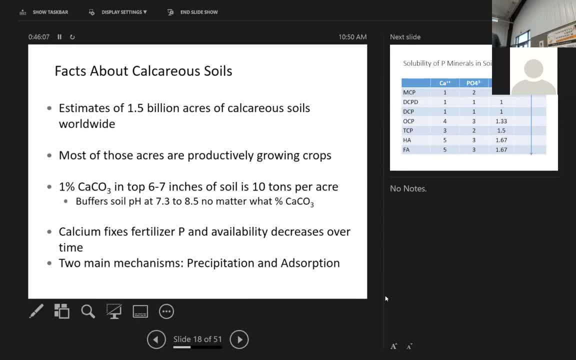 Well, here we go, Right here my calculation. Hopefully I got that right. So it is water. we do have calcium fixation and there's really two ways that that happens. We kind of talked about both of them- precipitation and adsorption- and I'm going to tell you: 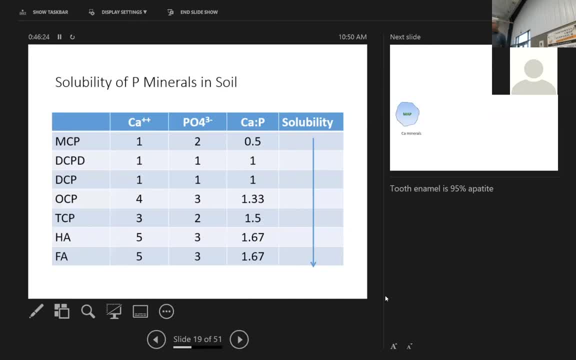 a little bit more about that in just a minute, But this kind of gets to your question, Jared, thanks. So what happens when we put that on this? MCP is kind of the most soluble form of phosphorus in the soil. After we put that fertilizer on it's monocalcin phosphate and we've got a lot of phosphate. 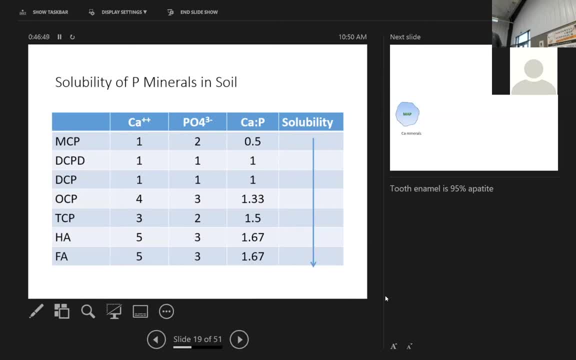 for every calcium on it. Okay, so it's pretty soluble, pretty available, but that phosphorus is kind of going to kind of go down this chain to the less available forms over time. I'm going to get to the time scale in just a minute. 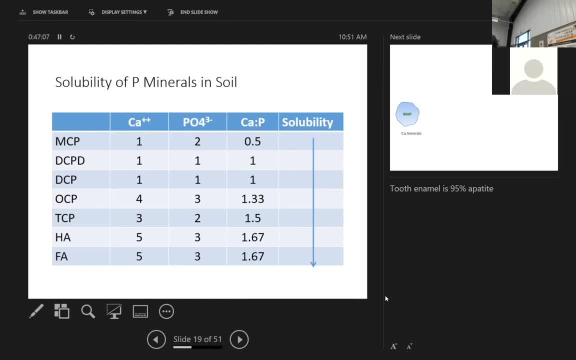 This is a little less available, so forth and so on. I suspect that you know we have a lot of this dicalcin phosphate not super available, but not super tied up either. Depending on our particular soil chemistry, we might get into this octocalcin phosphate. 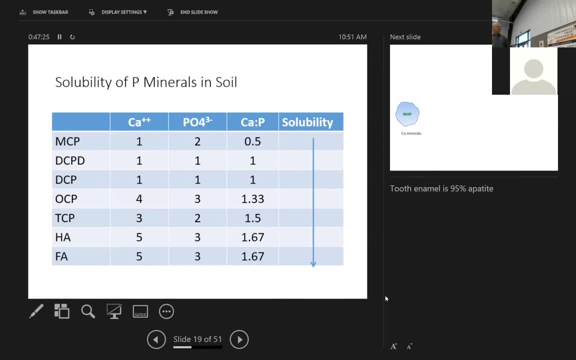 which is a little less soluble yet, and then some soils, and with enough time we'll get down into these lower levels which are very insoluble. This is called hydroxyapatite- hydroxyapatite, the HA there just to give you an idea about. 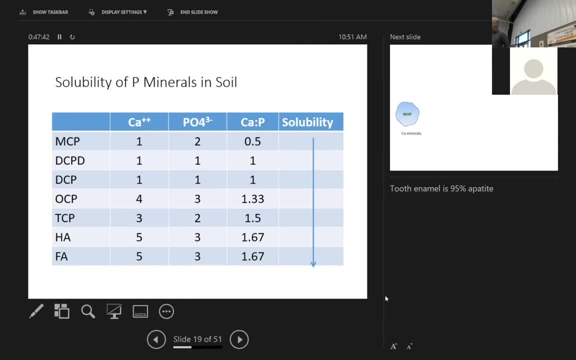 how soluble that is. Your cheap enamel is about 95% epithelial and the enamel it does erode over time, but very slowly right. So that's pretty unavailable and chances are. you know we don't get a lot of that. 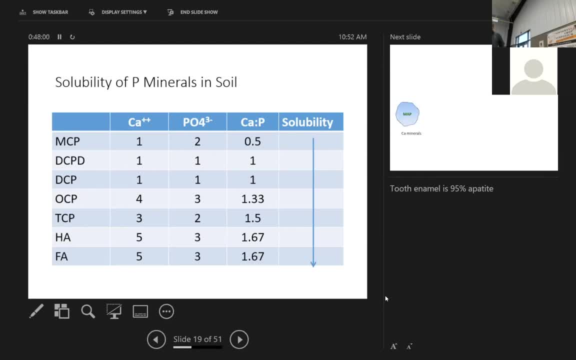 develop in our soils, but it is one form that it can get to, And the last one on here is floral epithelial. so that's epithelial with fluoride added. What happens When you brush your teeth with fluoride toothpaste? your enamel gets even harder. 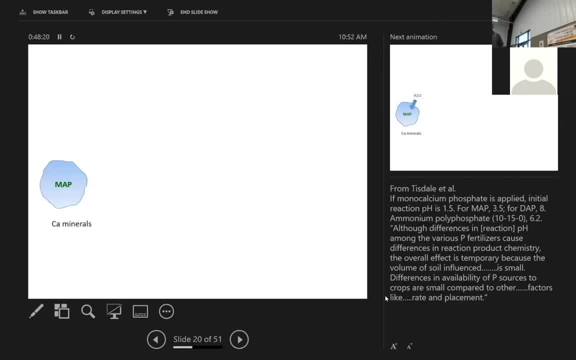 So those are the species we're looking at. So this represents a fertilizer molecule. I'd say NAF here probably really should be a calcium phosphate from the source that I got this from. So we have that, We put it in the soil and we have our calcium minerals in the soil. 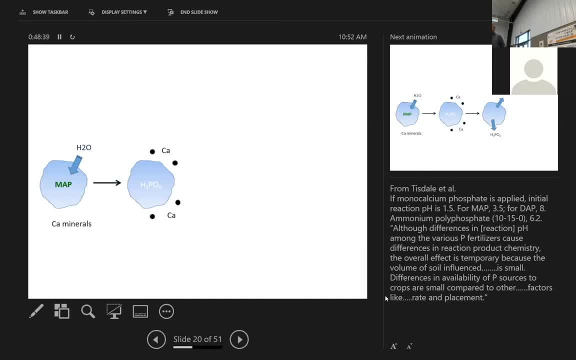 We get water in that, So that starts dissolving. that That's the fertilizer material, which is water-soluble, And when it starts we also have some other minerals in the soil around that particle. We develop phosphoric acid inside that granule, which again is very soluble and acidic. 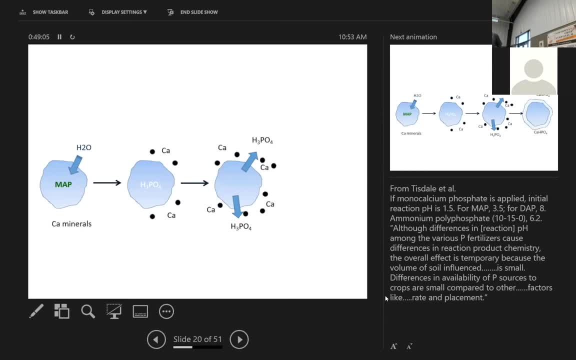 So that's going to then move out into the soil around, it react with chemicals and the calcium, and it dissolves a little bit of those calcium minerals, Releasing that calcium, so it can tie up the phosphors. The first product we get, though, as I mentioned a minute ago, is this dicalcium phosphate. 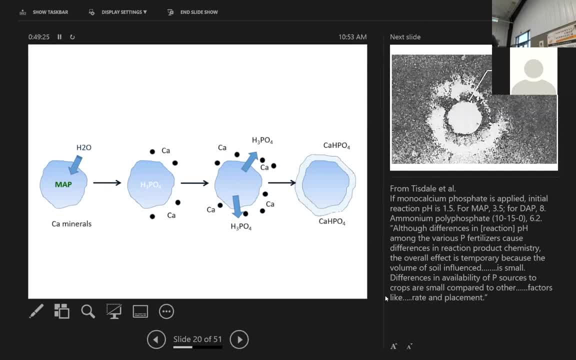 which is relatively available, And it's not going to move very far from that fertilizer particle, like I mentioned, because it just isn't mobile in the soil. So we get this little halo of calcium phosphate around that fertilizer particle, Again mostly available. 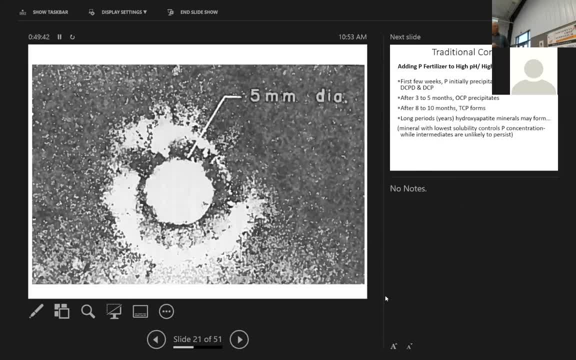 Plant can get to that pretty well. This is what it looks like in real life: Fertilizer particle about three-sixteenths of an inch in diameter and as that phosphorus moves out and diffuses, just another three-sixteenths of an inch and it starts reacting with that. 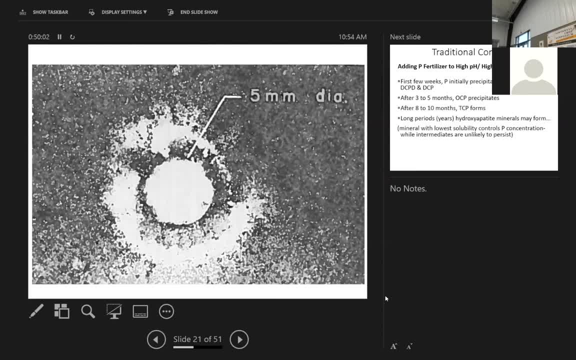 calcium and forming calcium. So that's what's happening when you put a dry fertilizer on there: Liquid reacts. similar, Only it's just a little different. So that's what's happening when you put a dry fertilizer on there: It's just a little different physically. 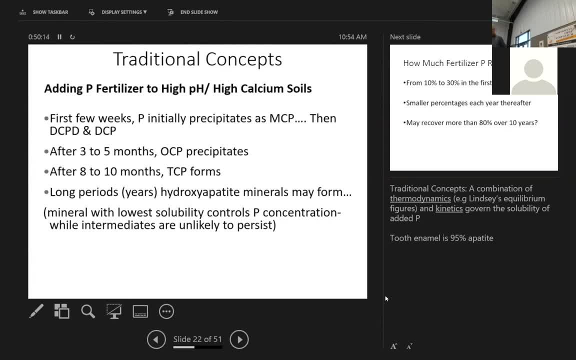 Liquid versus a particle. All right, So let's talk about some of our traditional concepts and kind of getting to this timing question. So in the first few weeks after we put that fertilizer on again, we go to that fairly available monocalcium phosphate. 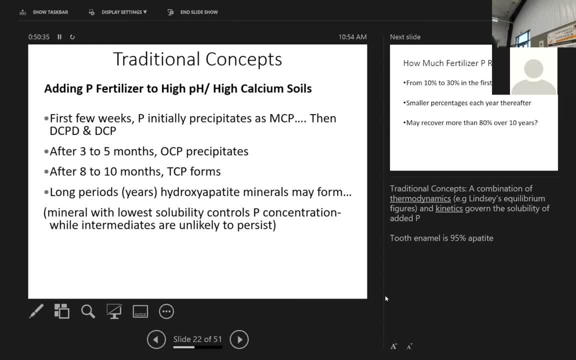 And then some of these are a little less available, but the plant can still get to it. Okay, Out three to five months We might get some of this less available material forming And even longer forms, longer times, you know. it's just going to continue to become a little. 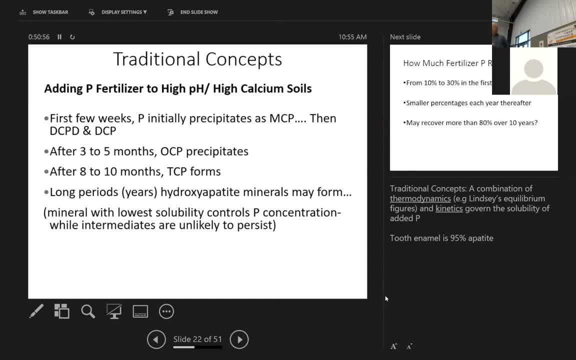 less available Long periods of time. we might get some hydroxyapatite Again if our soil chemistry is favorable to that. So it does kind of progress over that kind of a time, So within a year's time. we're talking about you know, we're talking about you know. 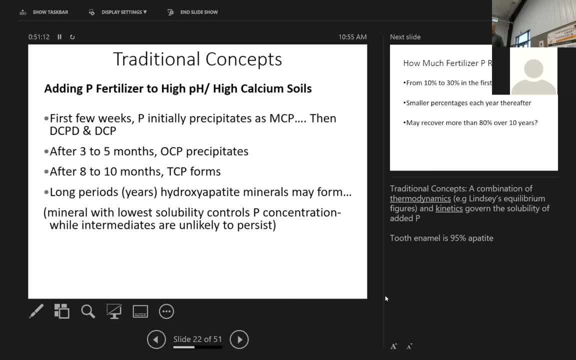 we're talking about, you know, pretty good availability. But you know, starting in a matter of weeks, it's going down now And certainly a few months, and we're going to see significant decreases, like maybe up to 50% reduction in availability. 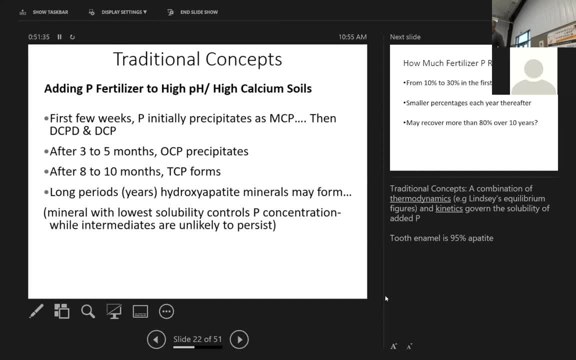 Yeah, Typically we fertilize our – Yeah, Yeah, We fertilize our alfalfa fields in the fall, So the fertilizer has time to break down and be usable for the plants. Is that the wrong thing to do, then, if it's starting to get tied up in the soil? 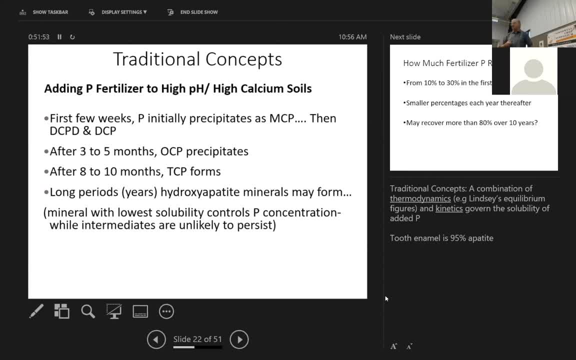 I would say no for a couple of reasons, And I'll touch on some of this a little bit later as well, But two things: When you're putting it on alfalfa, you're putting it on the soil surface, So it does need a little bit of time just to get some moisture on it and get it into the soil. 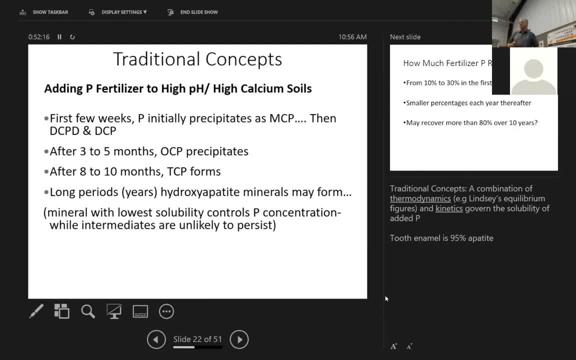 Keep in mind it's not going to go very deep, But deep enough to get to the root, So that I think it's beneficial to put it on in the fall. for that reason Also, soil temperatures are getting a lot cooler in the fall and a little bit in the fall season. 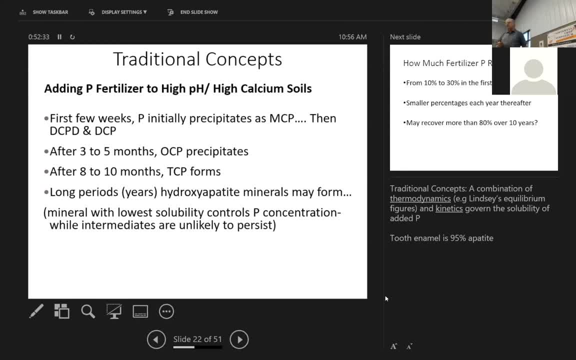 So those cooler soil temperatures are going to really slow down. It's safe And it's going to be a good irrigation reaction as well, And so I think the wrong about soil is frozen. I think we're kind of keeping a little steady state until it lands up. 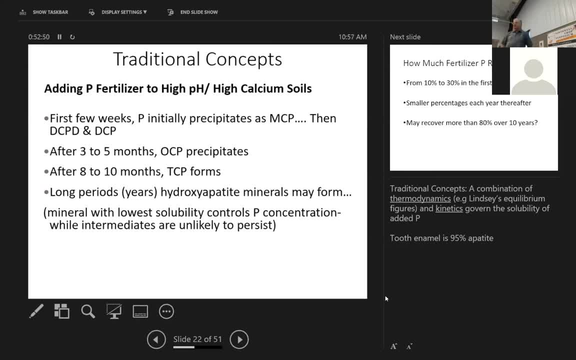 So again, we'll touch on this again in just a minute. One of the core principles of fertilizer management is putting it on at the right time, which means closest to when the plants can use it, which would suggest spring of date. But 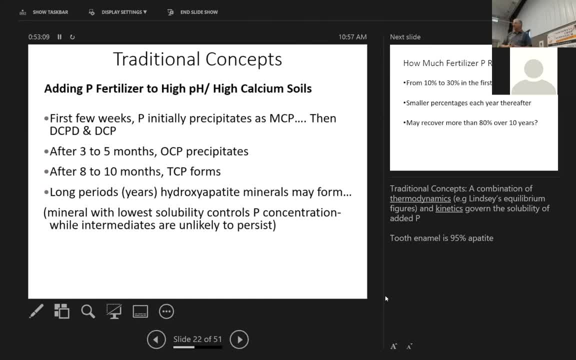 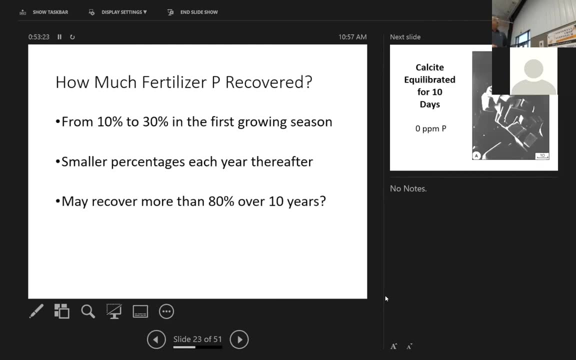 Again, we've got to get it into the soil if we're going to talk to the application. So it's kind of a toss up between spring and fall, but I think we're leaving it down. Okay, All right. so these are the numbers that scare us. 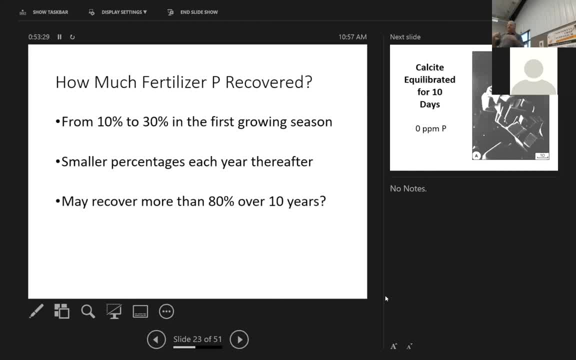 Fertilizer recovery. First growing season of that fertilizer phosphorus we put on the soil will get maybe 30% in the crop- $1,100 a ton, and then again 30%. Yeah right, That's the scary one. 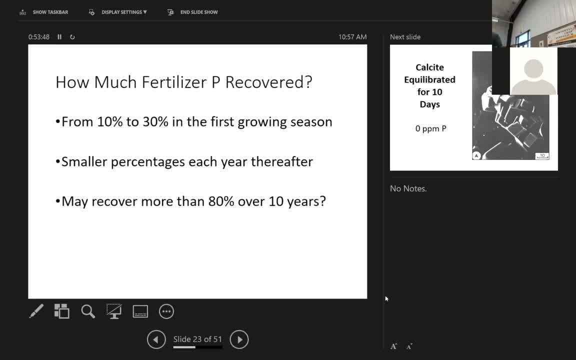 But keep in mind that's just in the first growing season. We're kind of feeding that reservoir, that big, huge reservoir of phosphorus. Some of it will come back, Probably not all of it, You know. over years, maybe 10 years, you know we might get 30% of that back. 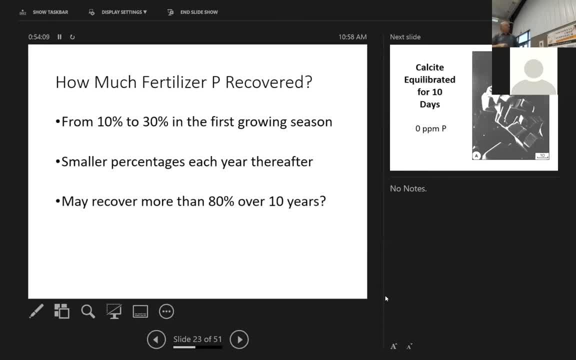 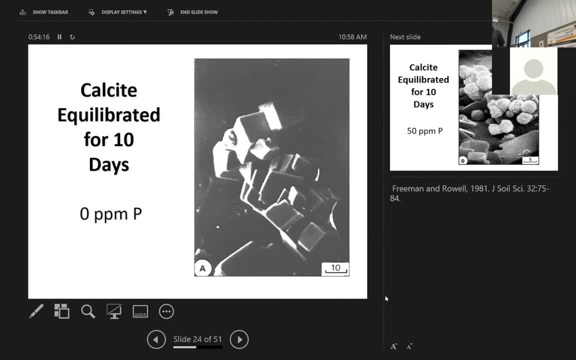 That's just kind of some rough rule of thumb figures, but it is a reversible reaction, All right. So we talked about precipitation of phosphorus with calcium. This is what happens with calcite or calcium carbonate. This is an electron micrograph of calcium carbonate crystals exposed to zero phosphorus. 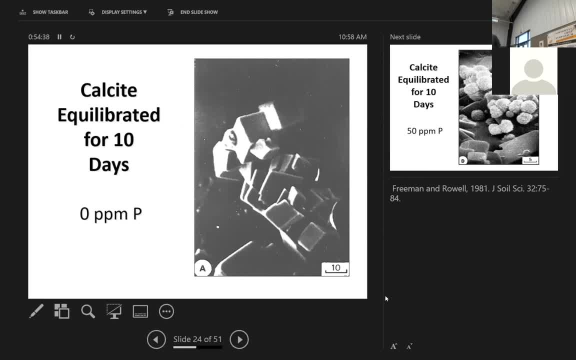 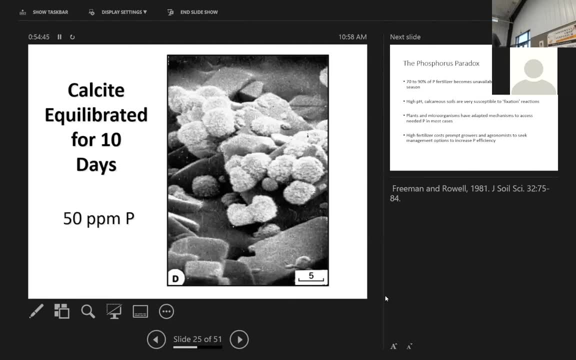 Okay, Nice, clean, beautiful-looking crystals Just equilibrated with water for 10 days. Okay, If we add some phosphorus to that, 50 parts per million. you know we still have those calcium carbonate crystals, but we're starting to see some of the phosphorus get attracted to and down to that calcium carbonate. 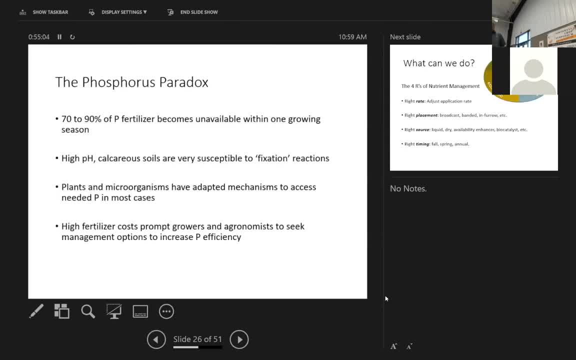 So that does happen, Just part of the process. So there is a little bit of a paradox. You know, we talked about fixation. I think we kind of beat that to death. Now I kind of want to talk a little bit about what some of our options are. 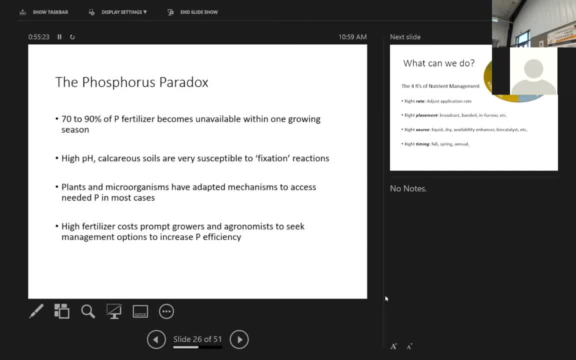 Let's see here. As I mentioned, plants and microorganisms have adapted mechanisms to help with this process. We'll talk about a couple of those, And, of course, this becomes more of a concern when our prices are the way they are now. 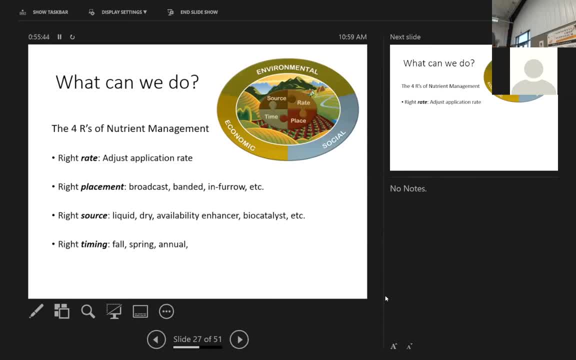 So basic principles of nutrient management. You've probably heard this before, If not. well, here it is The four R's in nutrient management, And this is these are principles that we hope will improve our fertilizer use efficiency. Okay, So the mean the four R's. 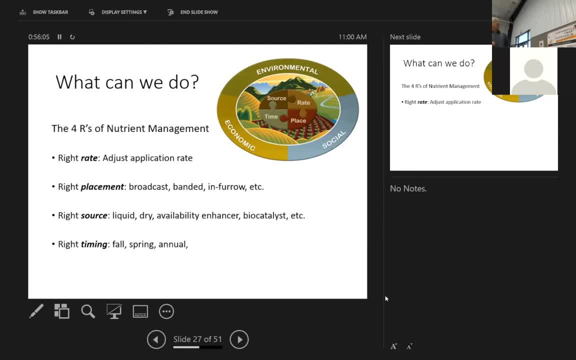 You know, have Certainly environmental impacts- Phosphorus can be a pollutant Economic, obviously for our production systems- And social impacts as well. So what are the four R's? The right rate, The right placement, The right source. 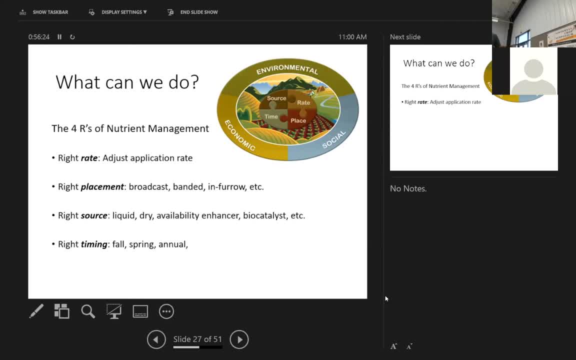 And the right time, Probably not need to say anything, And we're going to talk about some of these things as we go along, All right. So let's start with the first one: The right rate. How do you know how much to throw? 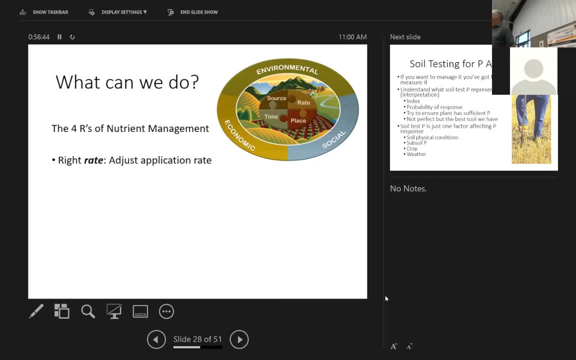 Good answer. I wish I had some candy. I'd throw some candy at you, Okay? Well, the answer is soil test And the question was: well, you heard my question, All right, So that is certainly the first two. 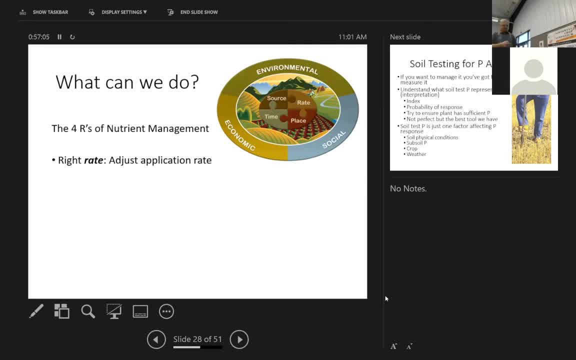 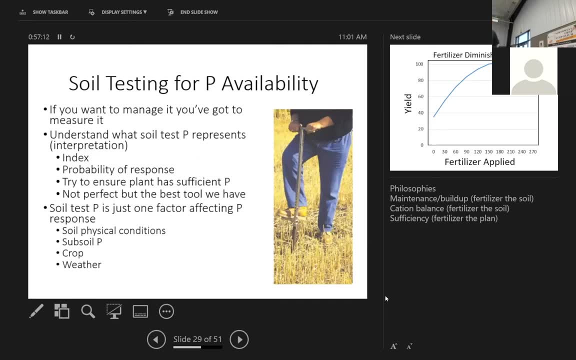 That's part of the equation. So, Yeah, Let's talk about soil testing. You knew I was going to have a slide on you, All right. So With As with A lot of the things that we manage in life, 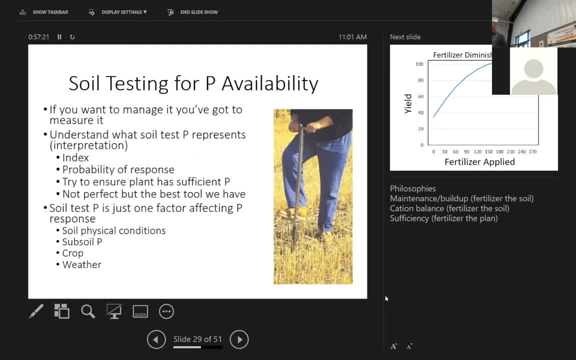 It makes it a lot easier to manage. Sometimes it can be a little difficult to understand what a soil test is. telling you Agree, Yes, Disagree No. Me too, But we have to understand some things about what a soil test is. 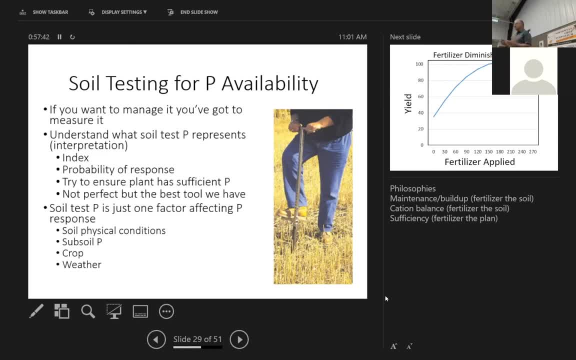 It's an index. With nitrogen We can measure the amount of nitrate in the soil. We know that's all available to the plant, So that's a pretty definite. The phosphorus is not quite so easy. Well, nitrogen is not either, because there's a lot of other things going on with nitrogen. 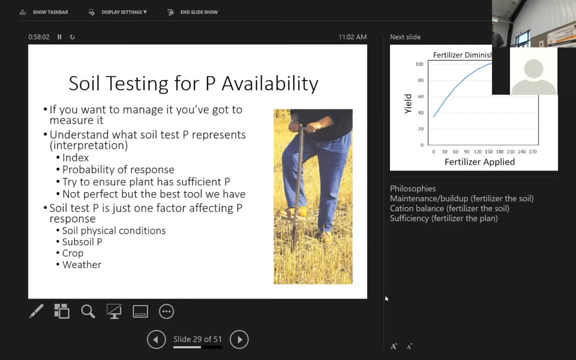 That particular test is pretty straightforward. So We We develop Procedures to give us some numbers. We then correlate with How a plant responds to. That's kind of what a Phosphorus soil testing For us, And it kind of tells us what the probability of response is. 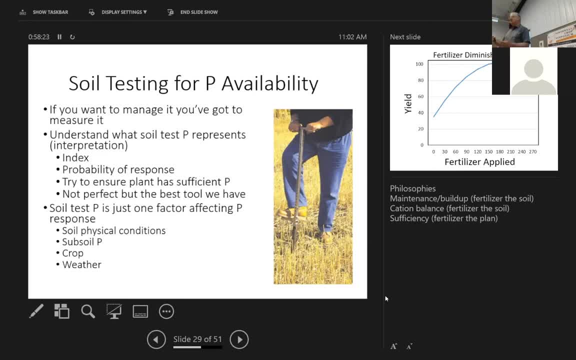 So we have a. If we have a soil test level that's very low, We can be pretty sure that if we put some fertilizer on, We're going to see that benefiting. If our soil test is medium or high, We might not see it. 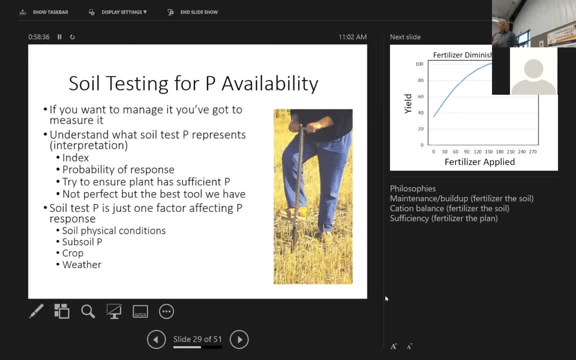 That year Might be fertilizing the system For Anyway, Or we may not need to put anything on it, Which is Most likely What we should do. All right, So Some different philosophies to handling soil, testing and. 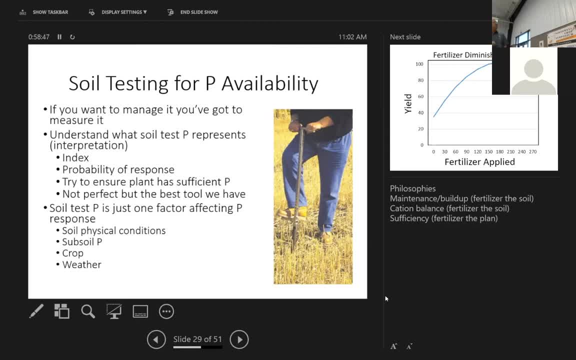 Interpretation of soil test results. The one that we generally focus on In Western United States Is just Making sure that the plant has enough To Be Fertilized. Soil, Soil, Soil, Soil, Soil, Soil. 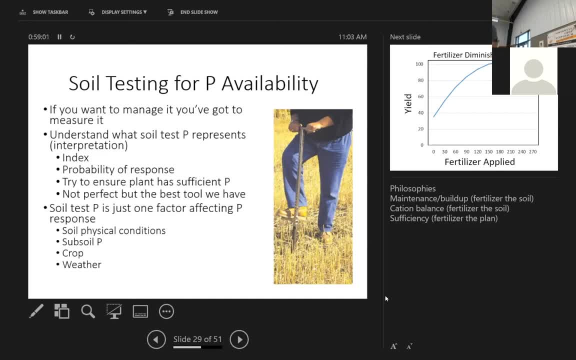 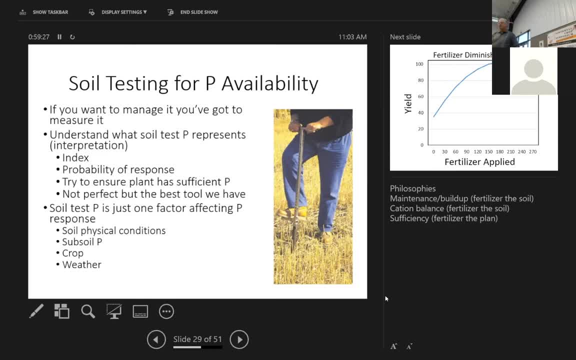 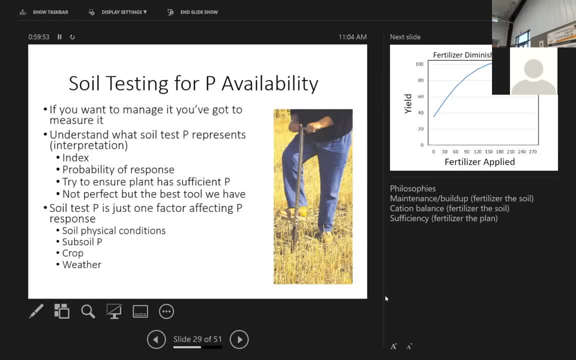 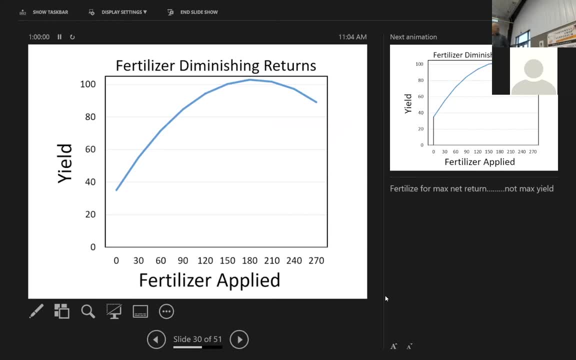 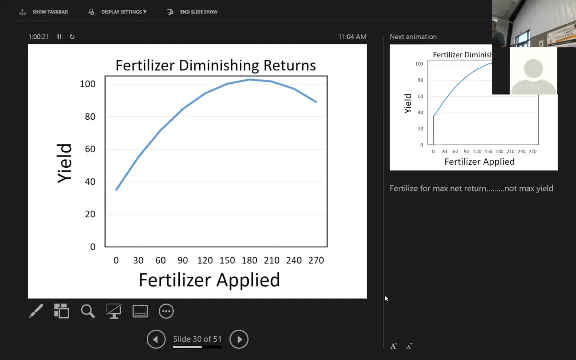 and we measure the yield at those different levels of phosphorus, You get the yield response. Okay, seen one before. All right, You don't usually look this pretty. I made this one from fake numbers, But this is a couple of points I want to illustrate here. Yeah, we'd expected when we put on zero fertilizer that we wouldn't get as much yield. 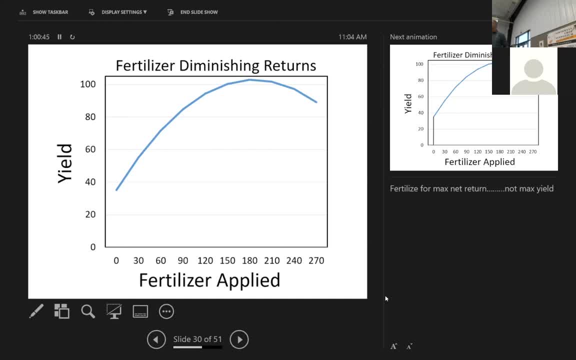 Now we'll never- I don't think ever- get zero yield, So we're going to start here somewhere. Okay, so we put on zero pounds, we get 38% of our yield, 38% of our yield, 38% of our yield. 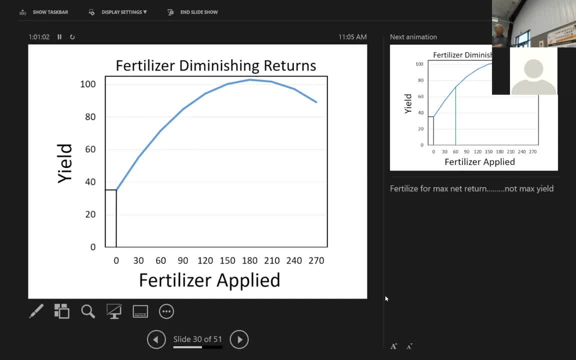 38 bushels, or whatever you want to put on this field. Okay, All right, So then let's go to another level. Let's go to 60 pounds. Okay, we got a response. Soil test was low, so we're going to have a pretty good chance of response. 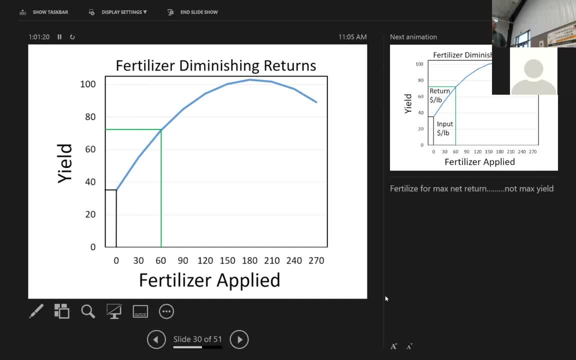 We did get a response. So we get: we're going to go from 38 to 70 something. Okay, pretty big jump Right, Right. So this is where we start. So we're thinking about economics. how much does it cost me to buy that 60 units? 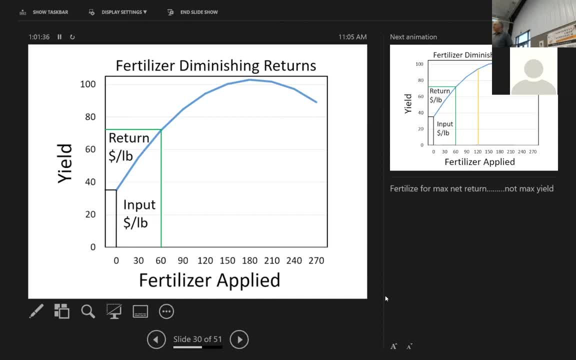 And how much did it return to be? basically comments that you think about every day, I'm sure. So as we go up this curve. put on 120 pounds, they were up to 90 plus, but we didn't get as much bang for a buck with that same input cost as we did with 50.. 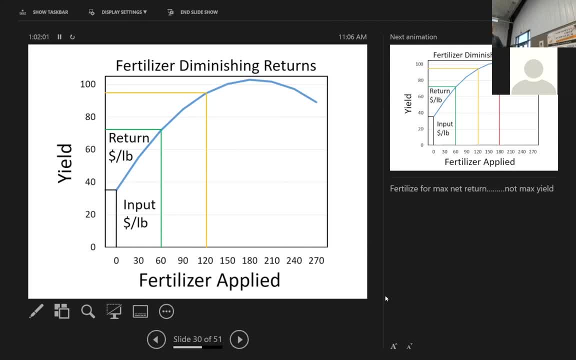 And that's just a general basic principle for this kind of response. yield response. Okay, now it's still up here to the top of the curve. You know we always want to have the best yield in the valley right. How much are we willing to spend today? 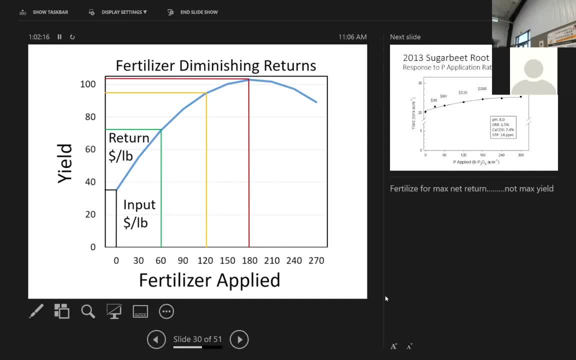 Right. So we put on that next 60 unit application And if this is percent then I'm doing really well. so I'm going to do about 103%. But the point is, you know much, much less return. So what is the value of that crop that you're producing? 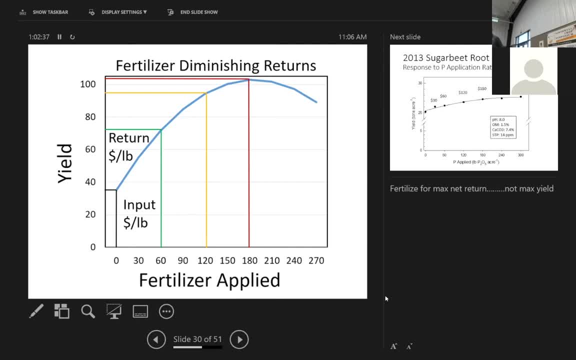 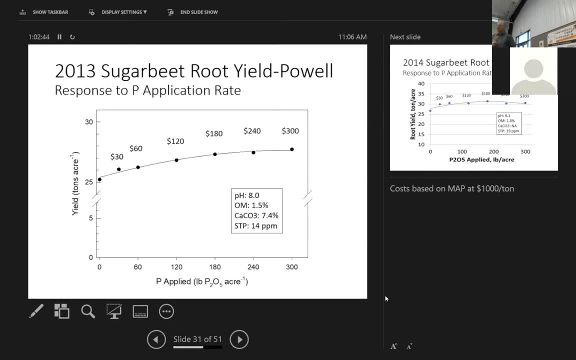 And is that input cost justifying what you're getting? Right, Make sense, Right? So let's put some real numbers on it from Powell here. Mike helped me with no, I helped Mike with this study a few years ago, a circuitry study where we did some different phosphorus treatments. 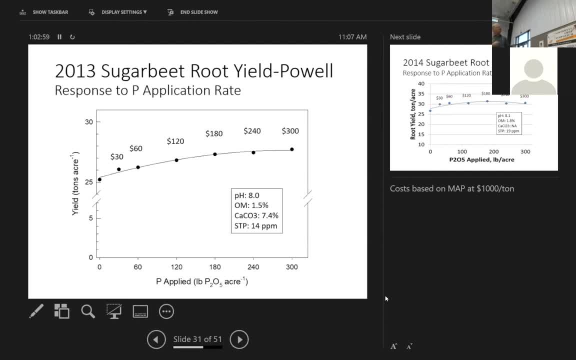 I'm going to share a little bit of those results. This is the yield curve from one of the years 2013,. at the research station, These are the characteristics of that soil or that site that we put it on: pH of 8, organic matter: 1.5, 7.4% calcium carbonate. 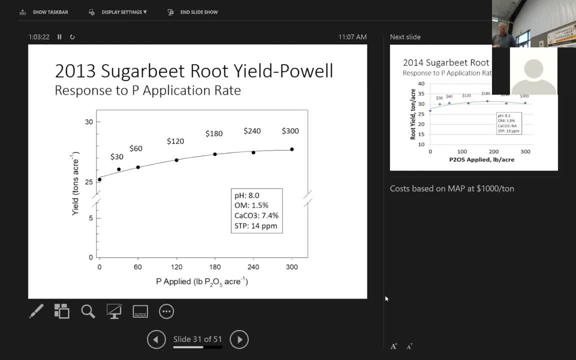 So we're up there And soil test: phosphorus is 14.. Now one of the problems with doing phosphorus research on research is that researchers don't like to have nutrients be a limiting factor when they're doing variety trials or other kinds of research. 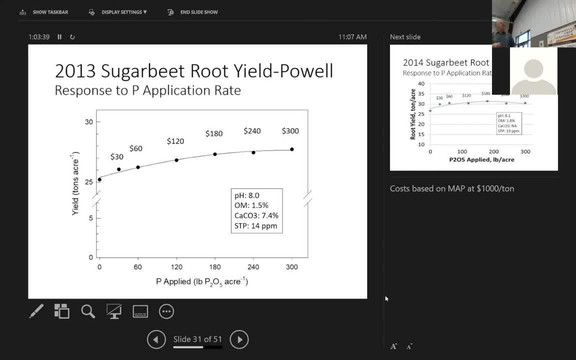 So it's hard to find a spot on a research farm where we have real phosphorus. This would be a medium Really. you know, in the 5 to 10 parts per million range is where we really expect a response. So we're above that. 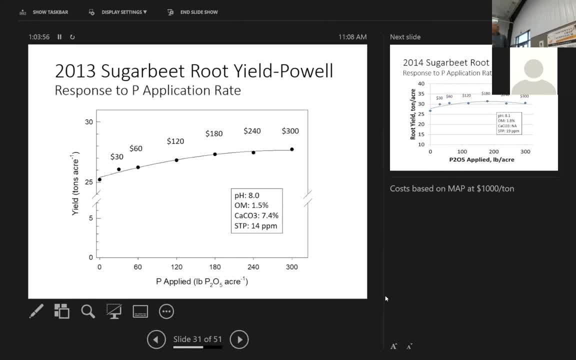 We did get a little bit of a response as we went from zero to way up to 300 pounds of phosphorus. You would not do that. I don't think Especially at $1,000 an acre or $1,000.10.. 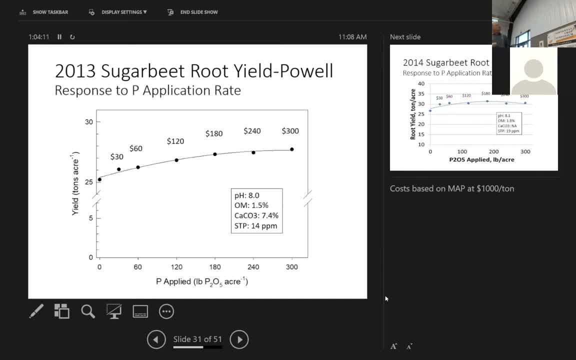 That's just what these numbers represent. So as we went from zero to 30 pounds, we got a pretty good bump, Kinda like our yield curve on the previous slide would suggest The biggest increase of all of them. We did continue to get increases all the way up to about 180 pounds per acre. 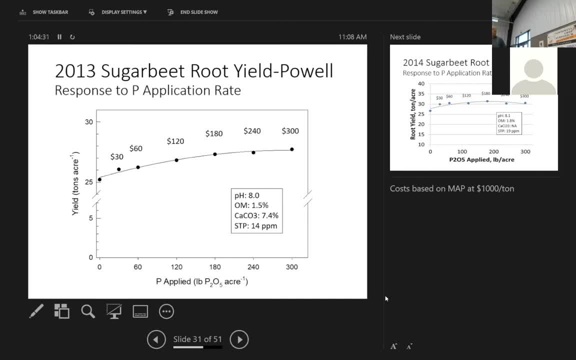 So that's pretty good. We did continue to get increases all the way up to about 180 pounds per acre, but, um, you know, just going out a number for the value of a sugar beet crop, i'm going to say 50 pounds, or 50 to 10 roughly. i think i'm close, um, and so we're putting on, you know, for every. 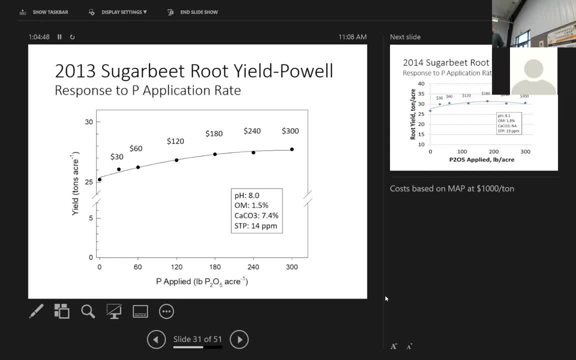 30, uh, 30 units of phosphate, uh, it's costing us 30 down. so for that intent of that, you know, put in 30, getting off 50.. you just have to go to 60 in the piece prices. certainly don't want to be up around 100, right. 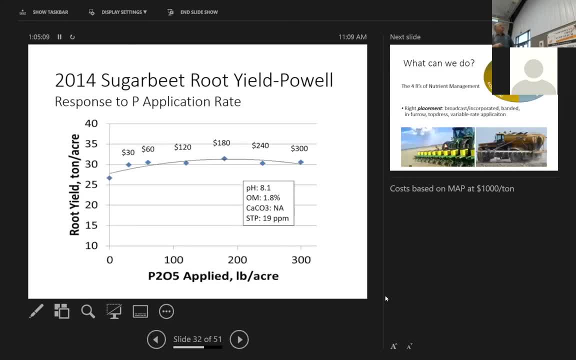 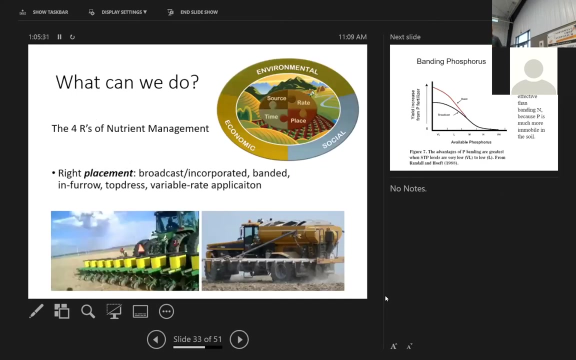 all right, so same same concept, different year. uh, same study. uh, 2014. again, we fit a curb to it, but you could almost say we got a good bump with that, that 30 pounds, and then it's pretty flat. yeah, right right. pretty simple dollars and cents there. all right, so what? 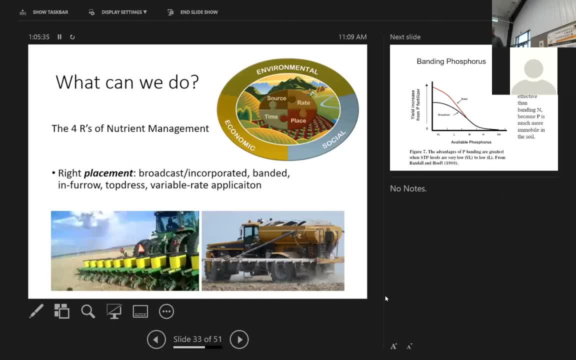 can we do next item on our list of placement? uh, if we talk a little bit about that, we have some options. um, we can be broadcast incorporated, which is our normal procedure. put it out there, work it in. that has its advantages. you've got that phosphorus distributed throughout soil profile. 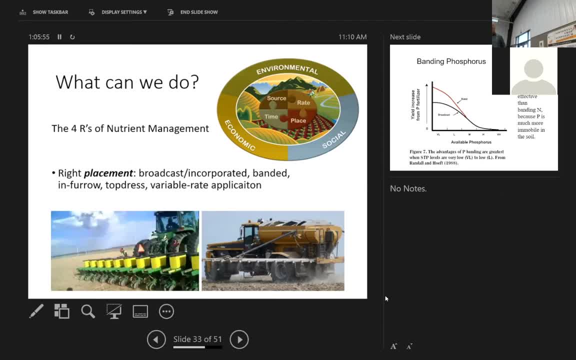 soil and get to that phosphorus pretty easily. however, that's the maximum exposure of that phosphorus fertilizer. for those ion reactions in the soil right, no protection, unless, unless we have some kind of product that we can add with it that might help. we'll talk a little bit about that. so 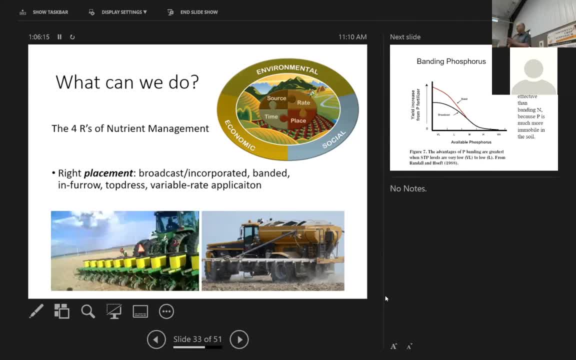 we can band it. that puts it in a concentrated form. less exposure to the soil, so preserve that availability for a longer period of time. okay, and typically we can get the same benefit from less phosphorus if it's banded. how much, uh of a? how much could you reduce your phosphorus rate? so that's. 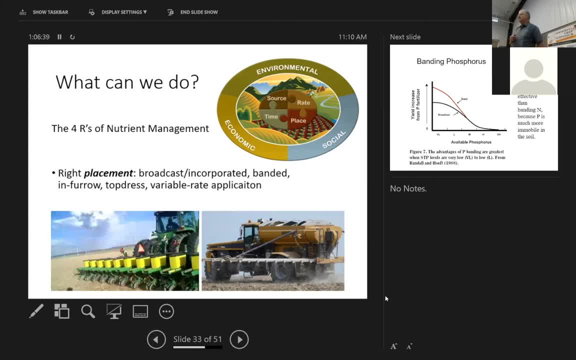 another opinion. some people say up to 50 percent. um, i'm a little nervous about that number. i think 20 to 30 percent is probably pretty, pretty safe. we could reduce our rates because of dandy. um, so banding is an option. um, how about in furrow as a popular? 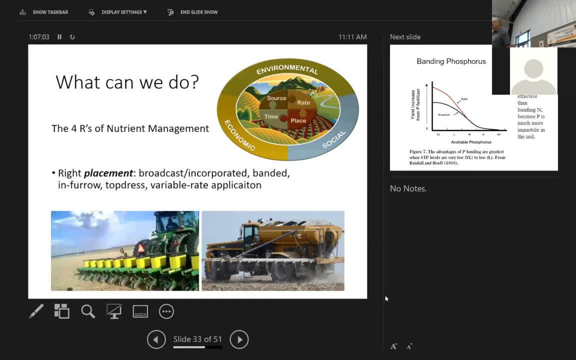 some of the the big growers do that quite a bit. put a little bit of phosphorus in with the seed on the dry land farms especially. um haven't done that so much under irrigation. but there are some people doing some things with referral stuff, particularly in the red river valley. 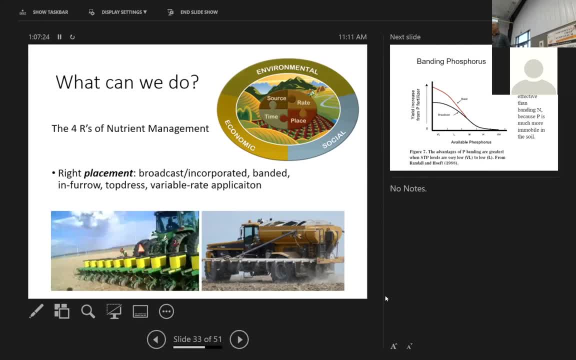 with corn and sugar beets, put a little liquid phosphorus in furrow and nothing else. they'll fertilize the rotation crops regularly with phosphorus, but they're just just put it in for all for the beets and the corn. so so that's an option. it has its risks and its benefits, um, risks being that anytime you put salt, 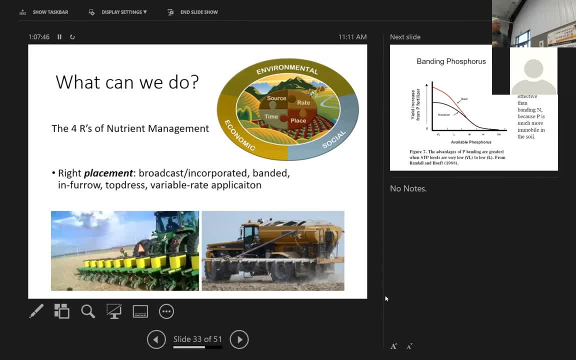 in it to see you. you're risking seedling injury. okay, all right. uh, top dress. um, the alfalfa, you can put a little bit of phosphorus in it, which you raised. you know, you're just putting it on the top for that appropriating advantages. and then, uh, variable rate. oops, there's a typo there. i thought 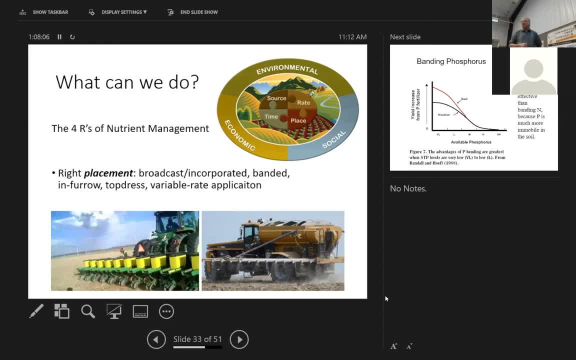 i got all those. sorry about that. i always find one when i stand up here and do this um, so that's putting it um in the right location in the field, hopefully. uh, we'll talk about that again in a few minutes. all right, let's talk a little bit about banding and, when we might, i'm going to talk a little. 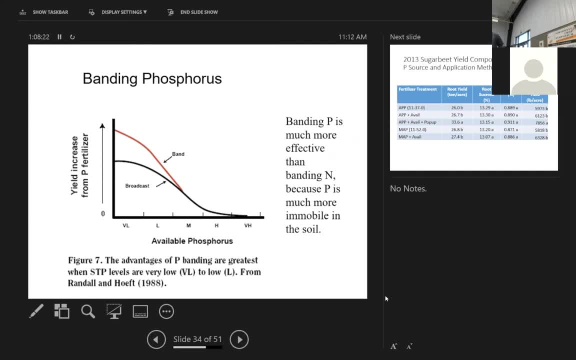 bit about banding and when we might. i'm going to talk a little bit about banding and when we might expect to see a benefit. there are really two scenarios where we would expect to see the biggest benefit, and the first is illustrated here, uh, from my uh, one of the scientists i worked with. 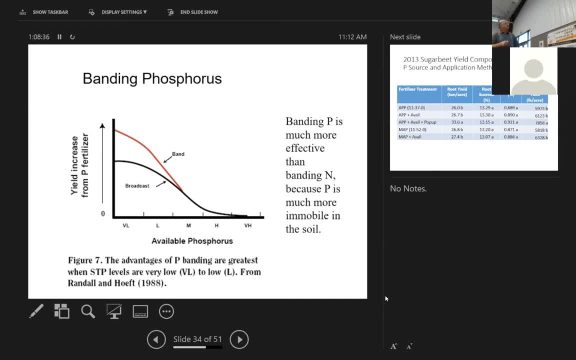 in illinois, bob faith um shows that uh, a yield increase from fertilizer. again this soil test level. don't expect to see a big increase out here. more as we get to the lower soil test levels with broadcast we're going to see a benefit, but as we get into these 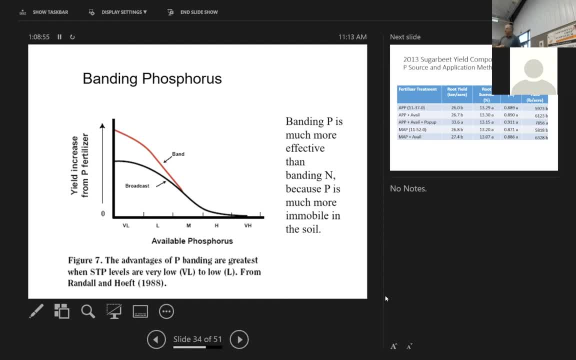 low levels. that's where we would expect to see if more of a benefit from the banding, again preserving this availability a little bit. the other scenario where we see more of a benefit from banding than broadcast would be in a no-till situation again. in illinois we did some work with 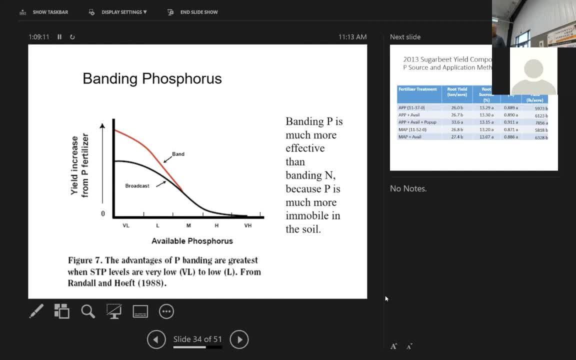 corn, uh, didn't really see a big benefit from starter fertilizer in full tillage, but in, that's what we did. cool soils, uh, we each don't go quickly and it's it's harder to get the fertilizer where you want it to. so a couple of scenarios where 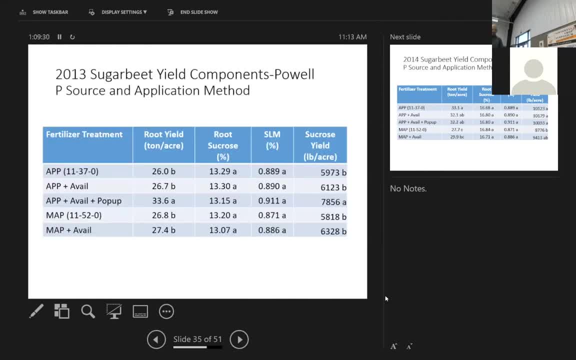 banding would be particular. all right. so in the study that that mike did, that that i helped out with, um we, we compared some of these things. our app is is a liquid phosphorus ammonium polyphosphate. you do that alone and and with an availability enhancer that you probably heard of. now, the concept: 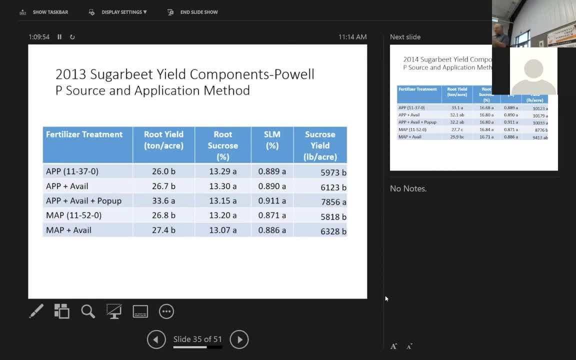 behind the veil. as i understand it, is that it it kind of diffuses out into the soil ahead of the phosphorus and reacts with the calcium before the phosphorus gets to it. so it kind of prevents the calcium from doing its damage for a time. okay, so conceptually it has some advantage. and then we 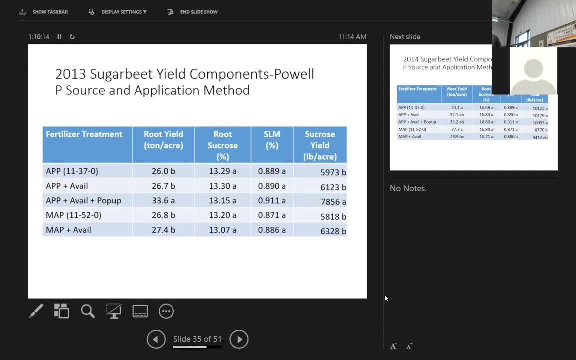 also put some imperil in with that treatment as well, and then we did broadcast of 1152 dripping it out of there. so in 2013, um, our pop-up treatment really did well. lower yield that. that year weather wasn't great, um, so lower yields overall. so having that, 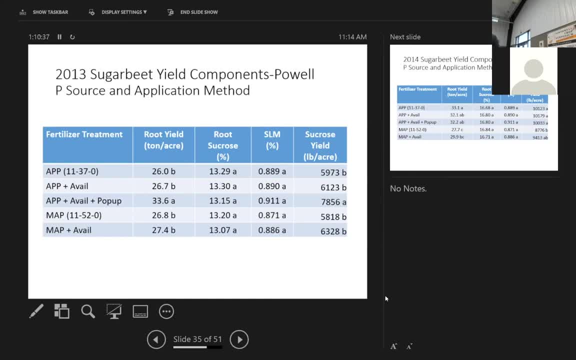 readily available during those conditions didn't see much benefit from uh the avail in either circumstance. but there's a numerical difference there that statistically that's pretty strong. so that was uh 2013, 2014, same treatments, um, and then this year we saw an advantage to the banded fertilizer. also happened to be the liquid. 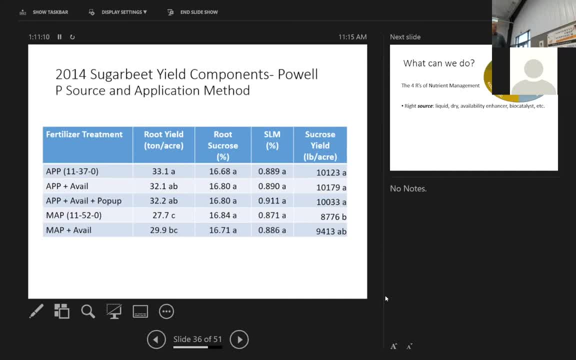 i don't know if it was because it was liquid wood, because it was banded, that it did a little bit better than the broadcast with that, but uh, probably a combination of both. i suspect that the placement was probably the driving pressure this year. uh, the pop-up didn't really provide any. 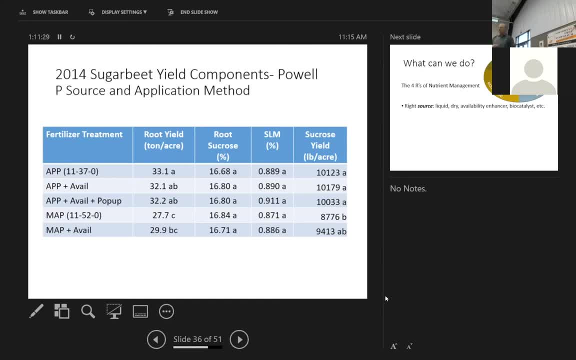 additional advantage. i know in at least one year we did see a little fans. that is a risk, all right. so a little bit of indication here that at least with a map that avail might have helped a little bit- not statistically significant, but close- if we, uh, if we loosened up our 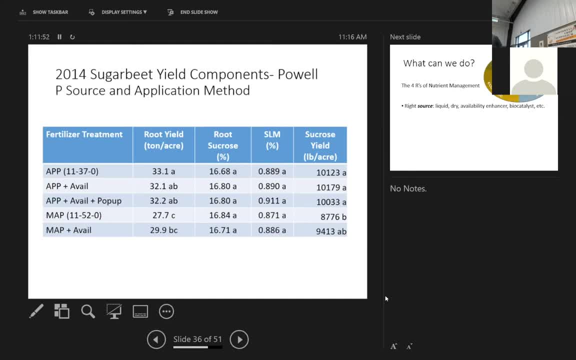 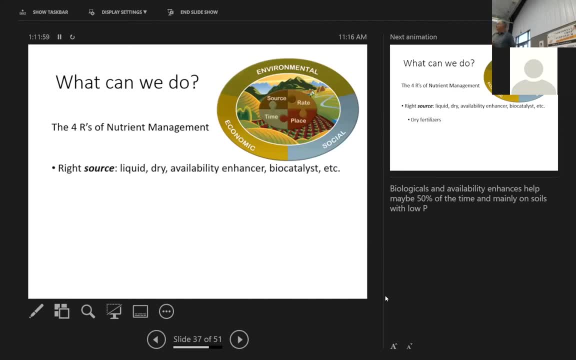 our criteria a little bit, we might be able to say it's significant. thank you so, bart. uh, you know, certainly with my interest in seed production, you know our grass seed producers, especially on heart mountain, and you know those soils really calcareous and most of those guys say a soil test is never going to show. 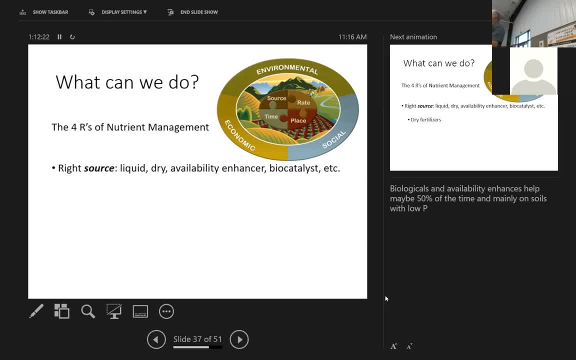 them that they need any phosphorus and yet they're putting down 100 units. you know, pretty regularly, maybe not every year, but every other year, and and they say they see a response: um, it's not, you know, it's not bart stevens with his plots, but but i have to believe they're not putting it on with their. 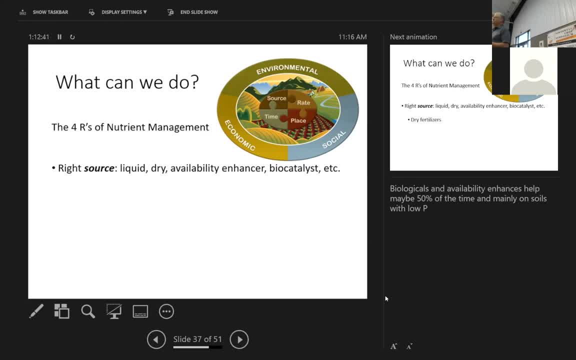 without some return on investment, um. so with that in mind, as well as something some recent work with by allied seed, they've been working with ofos um for alfalfa seed production especially, but it certainly piques my interest that ofos might work with other crops and they're putting it on as a foliar speed fairly late in the growing season. 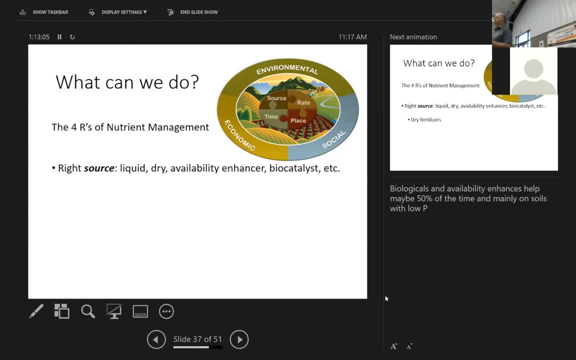 and they're seeing significant yield increases. um, and and i i believe what they're putting a lot of that yield increase to is is increased seed size. it's going on late enough in the year that it's not probably, you know, affecting seed set, but it is. 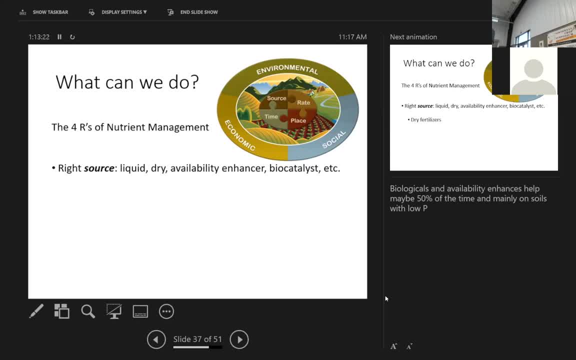 it is affecting seed size and i believe it also, they believe it's in fact affecting maturity. so you have some of those- later you know later- florets that were pollinated, that are actually make seed successfully. so can you, can you speak to and maybe also just a foliar feeding with. 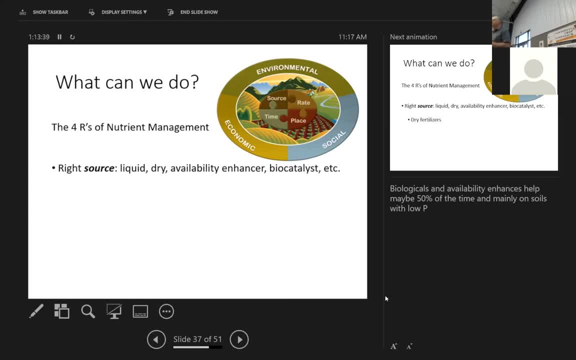 phosphorus and its availability, maybe throughout the growing season as well. there's a lot in that question, right? good question, thanks, um, short answer and i kind of hope to to make this my final point, um, but i'll make it now and then emphasize it again later. there's so many different options out there for products and 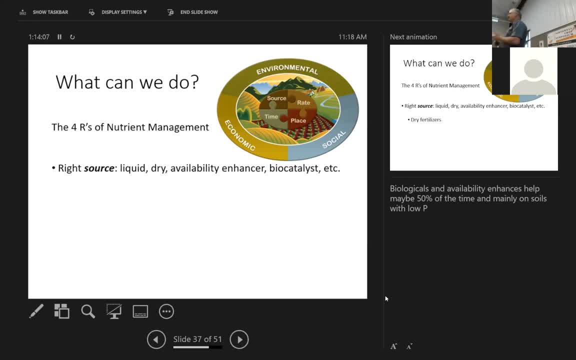 in different ways to handle our fertility that it's really impossible to do a good job of evaluating- evaluating them all in a research setting, as you suggested. so i'm a big believer in you know, something might work, try it and if it looks like it works on your farm, keep doing it. so i think 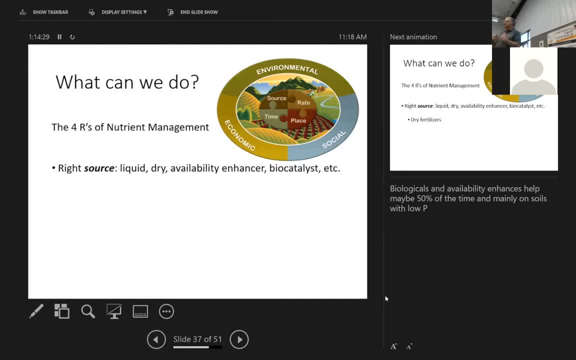 that's a huge part of this equation, but, as a scientist, i'm going to touch on it. the last, but it should probably be more of a focus- i've located it up um, the other part of your question, uh, foliars- um, as part of that micronutrients, micronutrient study that i did, uh, we did put. 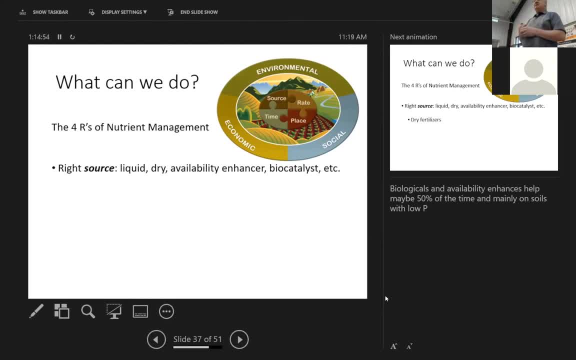 on some foliar treatment and, yeah, the plants take it up. you know you can put it on foliar, it gets it into the plant. so it's an effective way to put on a little bit of fertilizer and if the plant is in a high demand situation where it just can't get enough to fill out the 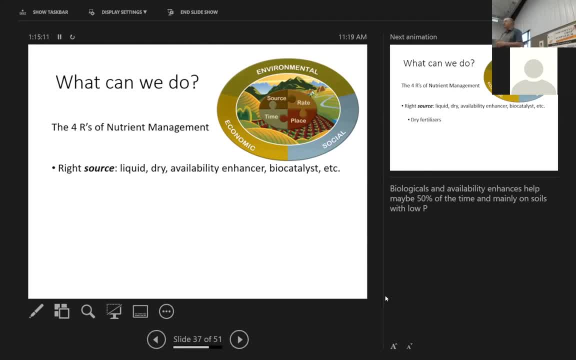 seed or or set seed or whatever the case may be, it may be bad. don't have any research data to back it up. don't have any issues with the data to say no, it doesn't work. you can probably find some out there to support either either side to that or you. 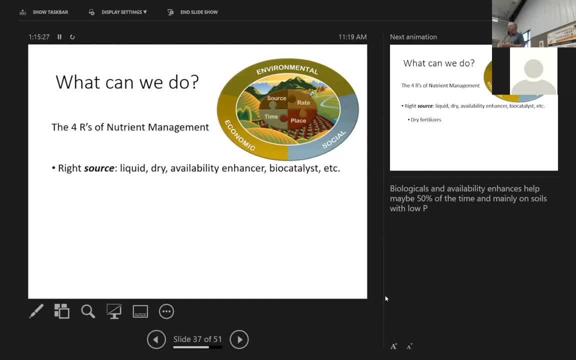 but, yeah, the works on the farm. yep, all right, we're getting close. how far over much time am i doing there? all right, the next one's a little shorter. you guys, you want to take a break? okay, i'm close. um so, uh, source kind of touched on that already. um, you got dry, oops. 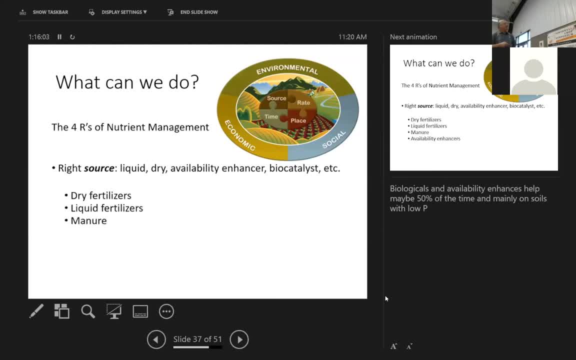 i think i got it back um. you got dry fertilizer, liquid fertilizers. manure is a great source of many nutrients a little harder to manage. uh availability enhances a lot of those um out there as well. talk about one um with high fertilizer prices. a lot of interest. 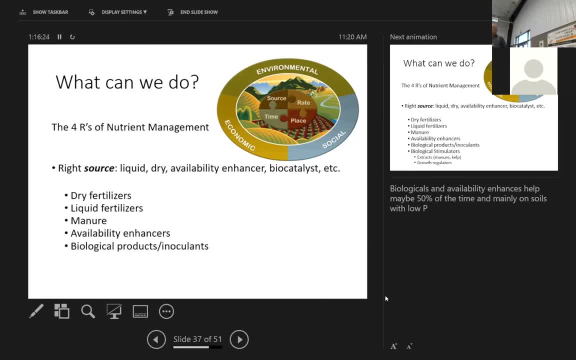 in some of these products, uh, biologicals, uh, we've got different kinds inoculants, biological stimulators, uh, ranging from extracts from like manure and kelp that have a lot of different organic compounds, to growth regulators that help stimulate. stimulate with you, and you know that there may be situations where any of these could be a benefit. haven't done. 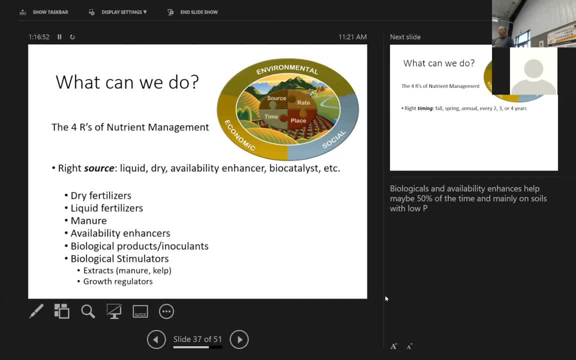 a lot of research with them. i'm gonna gonna try one this this summer in a study um, and it'll be interesting to see, uh, how those things work. but again, um can't share a lot of data with you on that, but try it on the farm, see if it works. all right timing, while we talk about this a little bit. 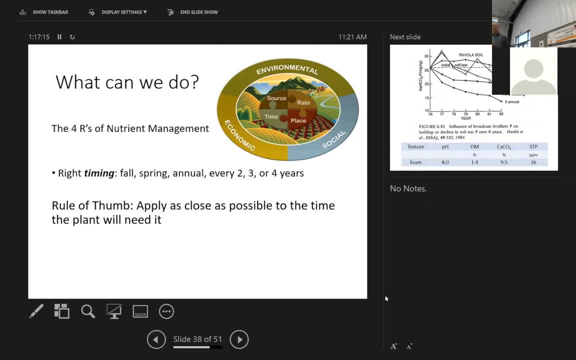 um, you know, we're going to put it on the fall, in the spring. uh, every year, every two years, every three years. these are all questions that are valid questions and there's a rule of thumb, as i mentioned before: put it on as opposed to when the plant needs it, as we can, but economics are part of this. 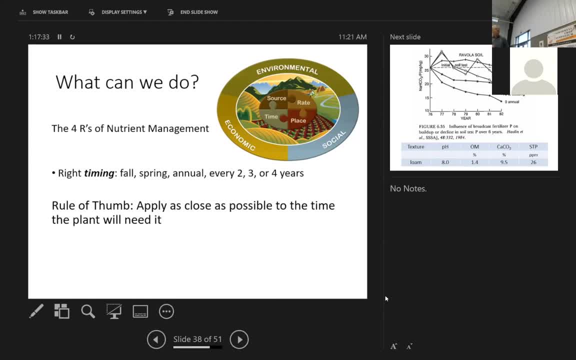 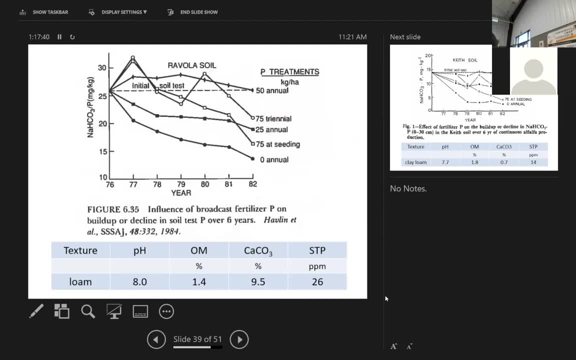 as well. you know that has to be a huge part saving trips across the field. all right, so just a little bit of data here from a really old study from colorado. uh, really good study, though kind of, looking at this, this very thing in a new alfalfa stand goes way back, like i said, 1976. 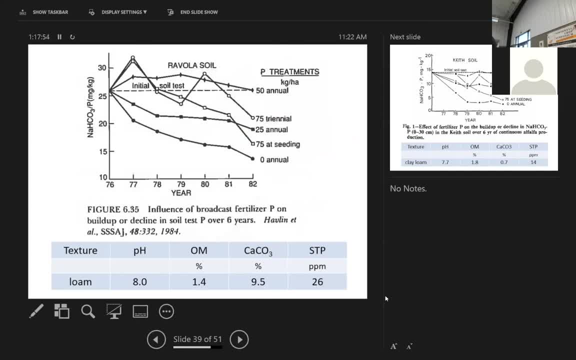 but the principles still apply. so the crop was seeded in 1976 and they did slow test and yield collection here over the next six years. these are the characteristics of that soil. this one was in western colorado iph: low organic matter, high calcium carbonate. now both of these soils have a pretty high 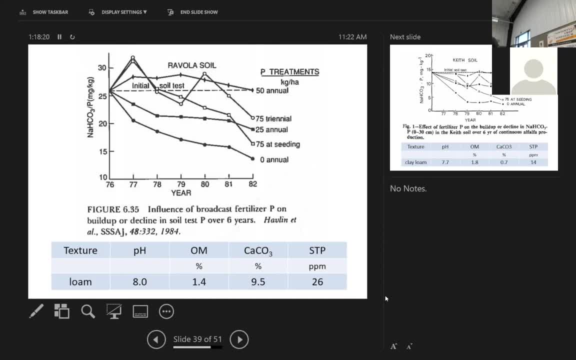 soil test factor: 26 parts per million- pretty high. you wouldn't necessarily expect the response, but this is looking at what happens to that soil testing level over those six years with, uh, five different approaches. okay, this is where we started. okay, so let's start with doing nothing. okay, don't. 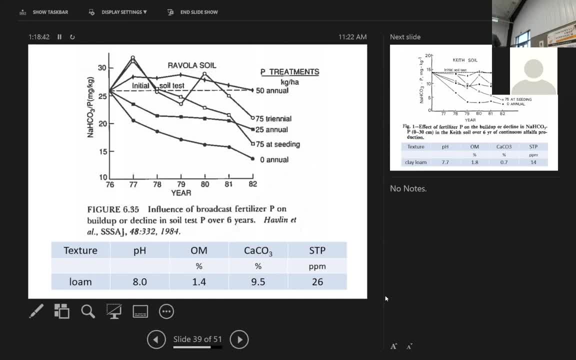 put any phosphorus on at all, test level drops pretty quickly over over that time. um, you know, just down in close to that range, 10 parts per million worth. so we can draw it down and draw it down. you know, first, first couple of years it's doing pretty good shape, all right. well, what if we put a little bit on every year? 50 pounds a year. we keep it up there and maintain that pretty well. if not increase a little bit for 50 pounds, well, what if 50 pounds is too much? you can't afford it. 25 pounds really didn't not as bad as we were, but it does continue to drop, all right. so what about? 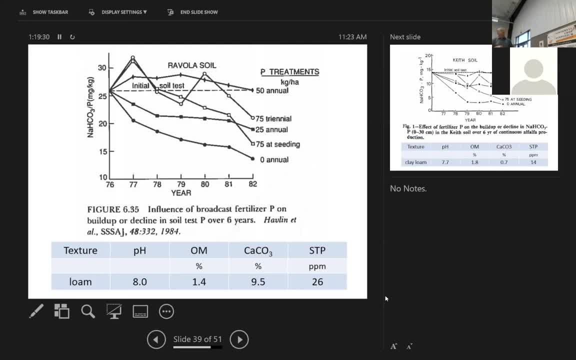 uh, putting a bunch on it, exceeding, firing it down. we do that quite a bit, been recommended to do that for quite a few years. put on two or three years worth. so they put on 75 pounds. you don't sorry, this is kilograms per acre, so i think this is more like 20, 40 and 60 pounds. 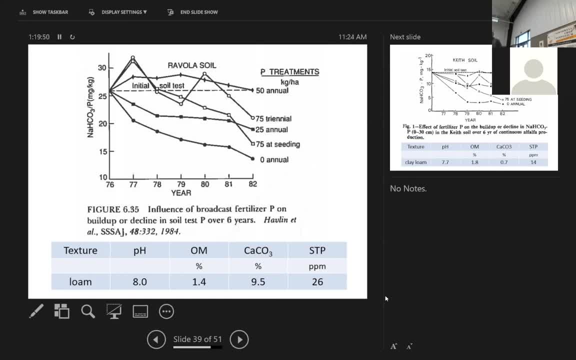 so we put on 60 pounds first year at seeding. didn't do anything for three years. well, let's take two different scenarios. didn't do anything after that for six years, and we did pretty good for the first three, maybe even four years, and uh, and then we dropped off. and then, if we added a 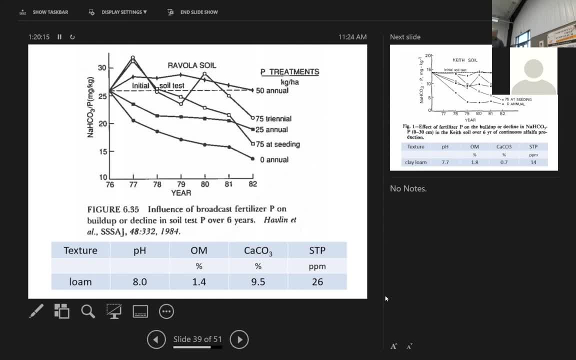 another shot after a few years, bump it back up. it's kind of like beautiful. so what's best comes down to an economic question, i think. um, certainly from a an efficiency standpoint, you know, putting a little bit on every year makes some sense from an economic standpoint, you know, maybe maybe every two or three years makes sense too. so again, i think, 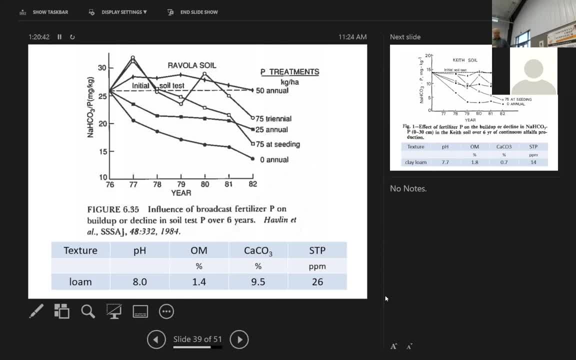 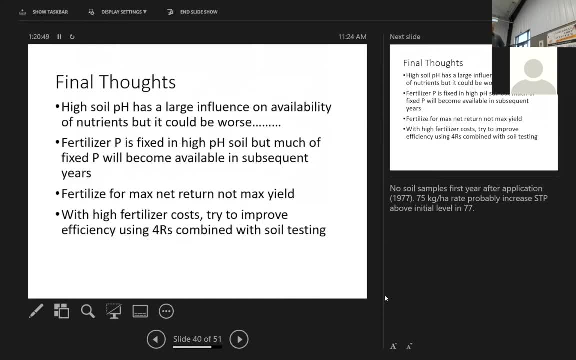 that's something that each grower kind of has to support, and i think that's something that each grower kind of has to support figure out on their own. um, another soil type kind of shows the same thing, so i'm just gonna skip over that one. 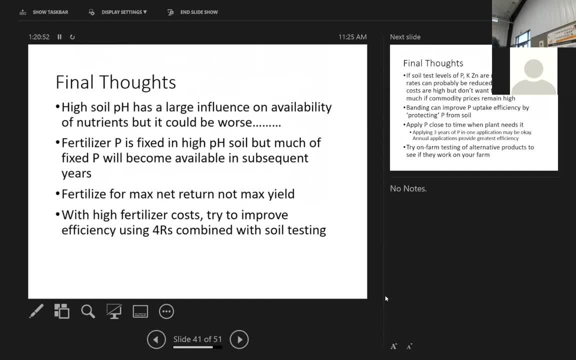 so a couple of final thoughts. um, so our soil ph is some something you definitely need to be aware of, and how it our nutrients. but, um, we could do, we could do here on the ph fertilizer. p is, yes, fixed our high pH soils, but we do get some of that back. and fertilizing from max net return is probably. 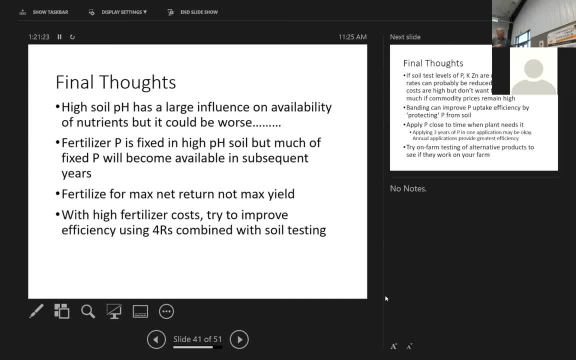 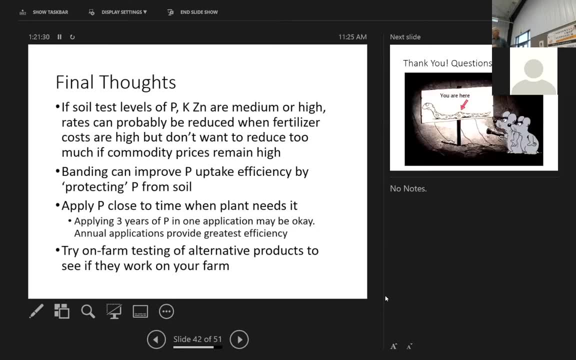 pretty wise right now, instead of maximizing them And then just keeping in mind those four hours as you make some of those decisions, Kind of looking at the nutrient package as a whole. Let's see what do I say there. If our soil tests are in that medium to high range, then 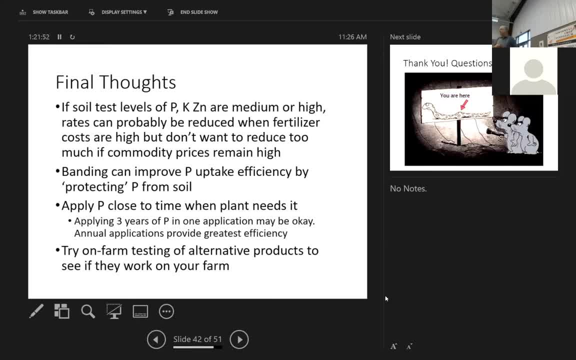 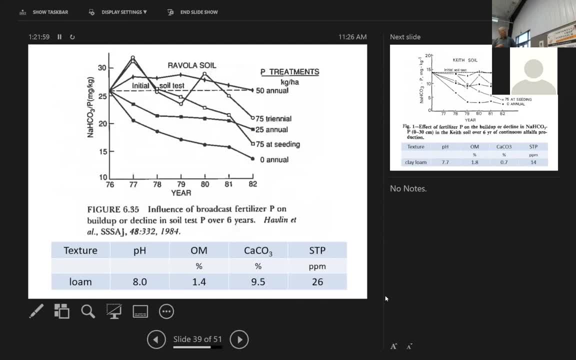 on a short-term basis when costs are high, probably cut back a little bit and save some money and not hurt. Oh, I did want to go back on that phosphorus study Didn't really have a whole lot of impact on yield. 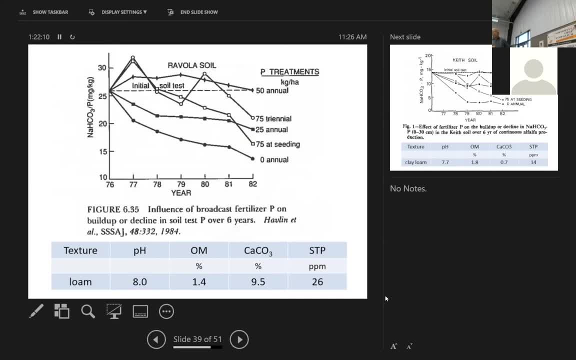 Now, part of that, I think, is because they took a 30 to one foot soil sample and really all the actual phosphorus is in the top few inches, So we might have been diluting some of that, Might have had more phosphorus available than this is showing. 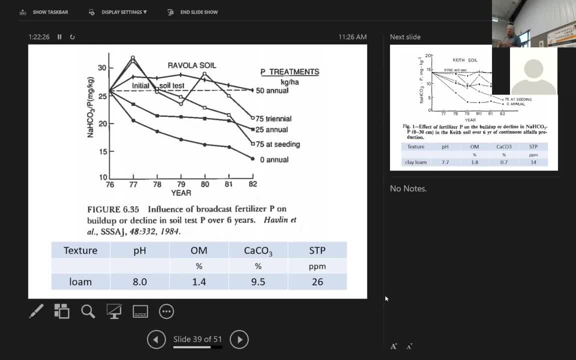 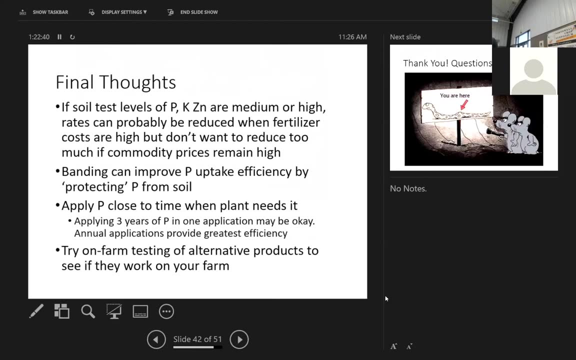 But also, once you get an established fertilizer, alfalfa stand, you got that extensive eat system and it's getting every bit of phosphorus that it can. That helps us too. All right, so back to this. You know you've got to keep economics as part of the process, part of the equation. 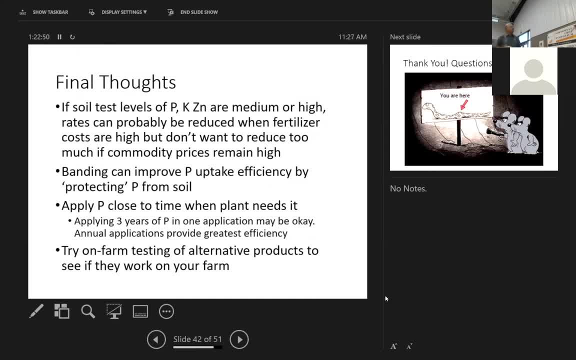 Talked about banding. It can be beneficial in certain circumstances and timing. And then, finally, back to Mark's question. Try some things out on the farm, see if it works. I know that's hard to do, Hard to take a step and just do something different on one step It can provide. 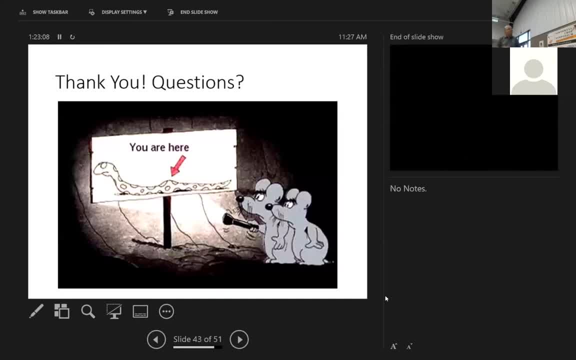 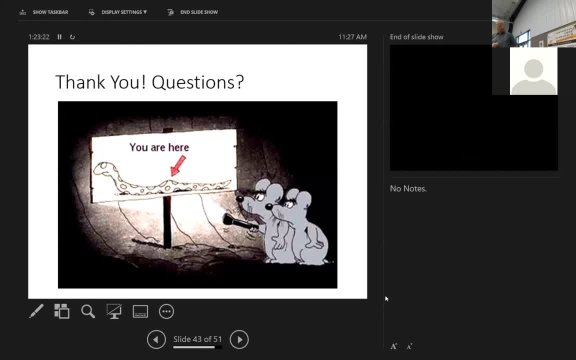 Actually this is. this is a little misleading. I think we're more likely here. Make you a little Feel a little better. I hope So over those years when the phosphorus becomes available again. that's just all natural processes, or is it a combination of? 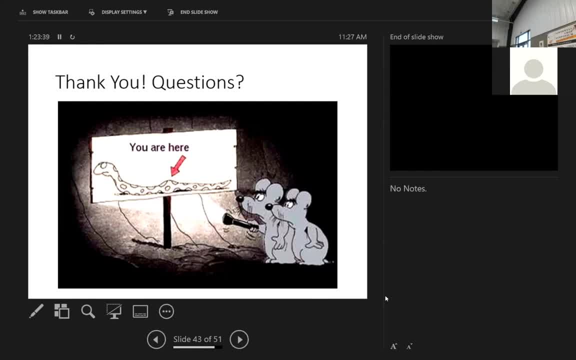 of putting more fertilizer on, or different fertilizers or something, some kind of additive, to help break that apart faster. well, i think, in that situation that i described, it's natural um whether or not there are products that we can add to to speed that up. i guess as a matter of 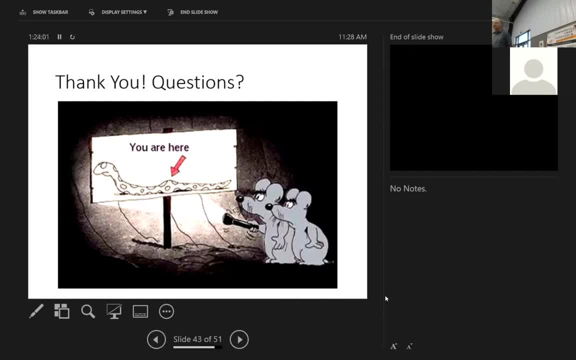 debate in the research community has been for years. uh, they've looked at microorganisms that are supposed to be able to release some of that phosphorus, seeing some benefit from that in some parts of the world. uh, haven't really shown a lot of benefit to the state. um, that's. that's kind of old research, a lot of new products now, i had to say. but i think most of the products that we're looking at now really are, you know, focusing on um, that root zone, either increasing the root zone and and protecting that phosphorus fertilizer, rather than mineralizing and releasing. 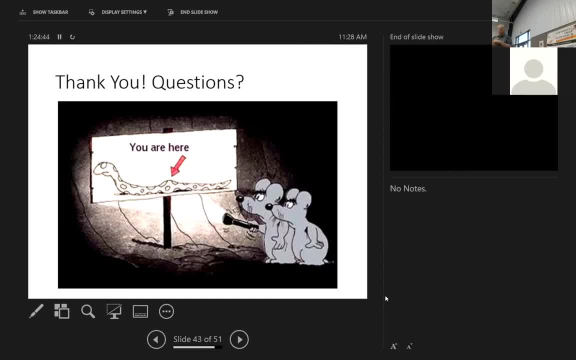 in my understanding. somebody from the fertilizer industry could probably correct me, but i'd say primarily: okay, great, thank you very much. we'll take a. we'll just take a five minute break here and we'll we'll get, we'll switch presentations and go from there. you. 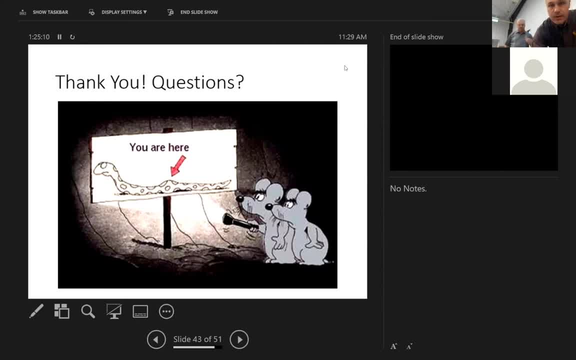 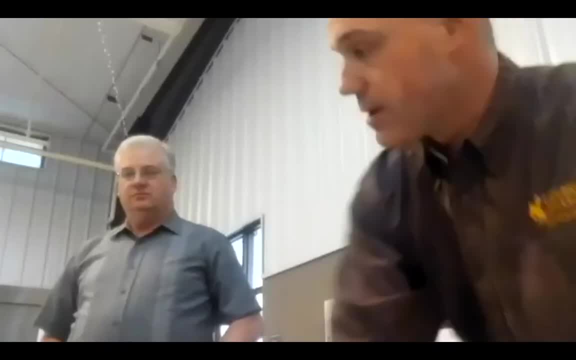 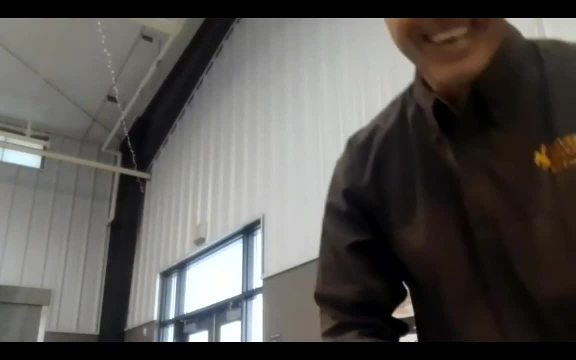 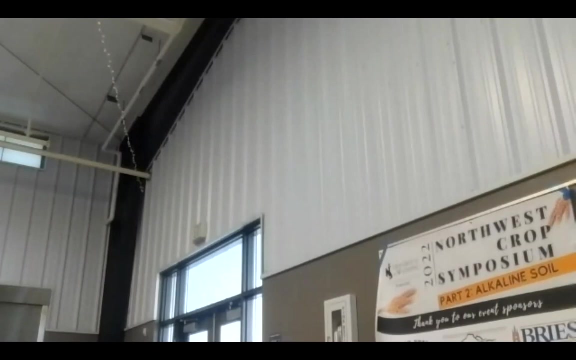 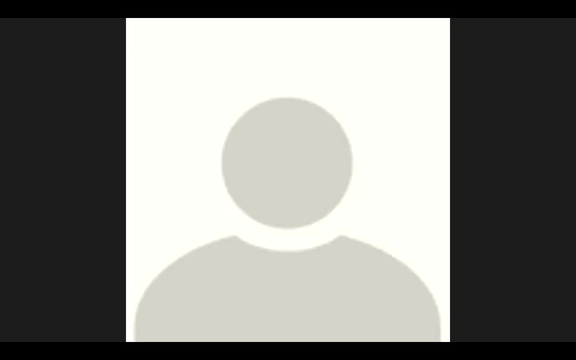